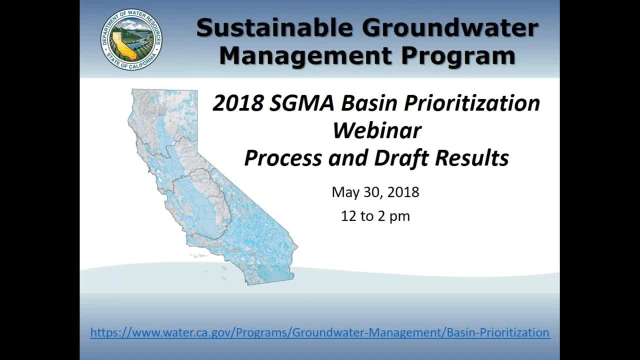 All right, So welcome everyone. This is a presentation today of the Sustainable Ground Water Management Program's 2018 SGMA Basin Prioritization Process and Draft Results. My name is Trevor Joseph. I'm one of the program leads here for the Department of Water Resources. 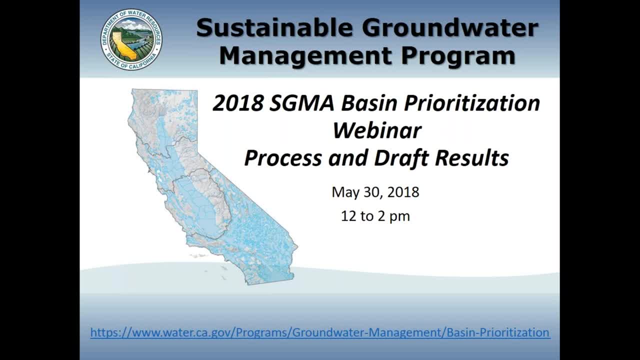 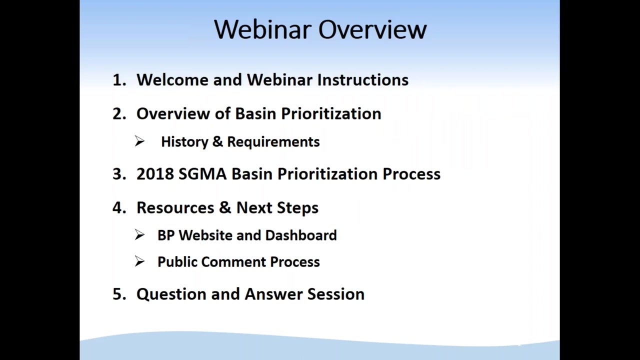 I'm joined here by my colleagues Steven Springhorn and Roy Hull. In addition, Sep Horry, who is a consultant, helping us today with our webinar broadcast, One moment while we advance the slides. Today, we're going to focus on some instructions related to the webinar. Stephanie will go. 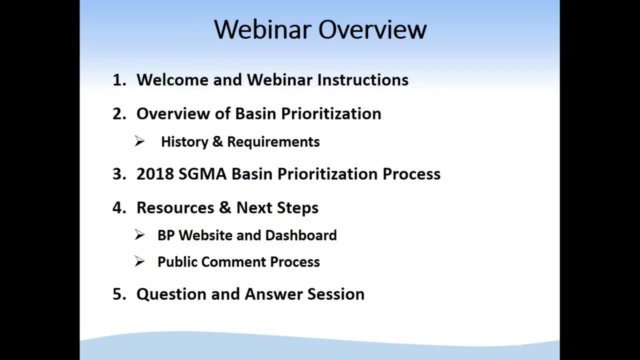 over that I'm going to provide a presentation, a brief few slides of her providing the overview of basin prioritization, some of the history and requirements. Roy Hull, the project manager, is going to go through an overview of the actual 2018 SGMA Basin Prioritization Process. 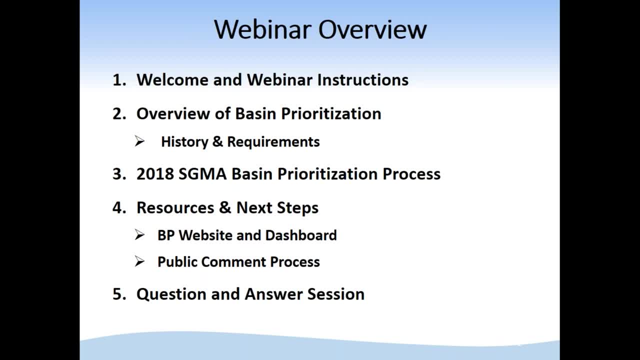 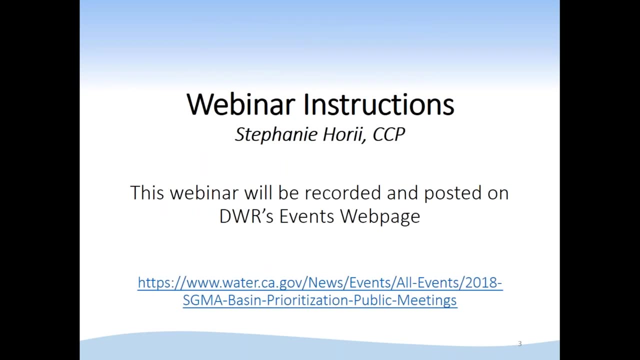 And finally, Steven will provide some information on resources and next steps. So we're going to open soon And then we'll open the webinar for a question and answer session. okay, good afternoon everyone. my name is stephanie roy. was sacramentus state for collaboration. 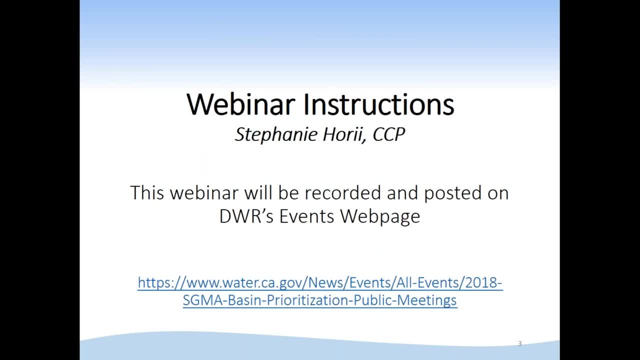 consensus program. i'm going to take a quick moment to go over how you can interact and provide questions during today's webinar, and you can get started by getting started with hoch: vivid information, soft listening explanations so that customers can contact donation students. this review and hint and answer to specific questions is on our website, which we alsobadwinnessinfo. 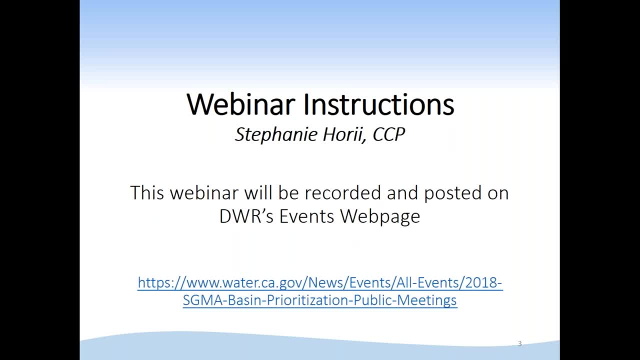 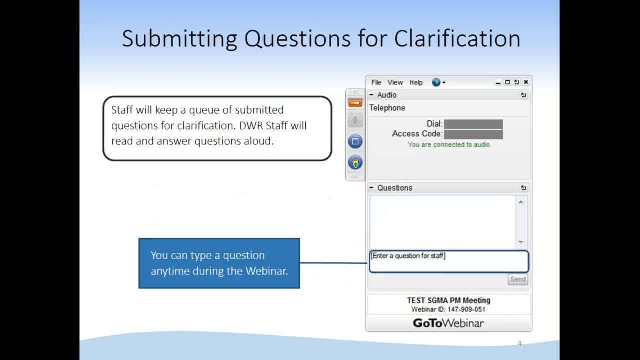 As you can see on the slide, today's webinar will be recorded and will be posted after today on BWR's events webpage. Now for submitting questions. for clarification, you can submit your questions at any time during today's webinar via the questions box there indicated on your webinar control panel. 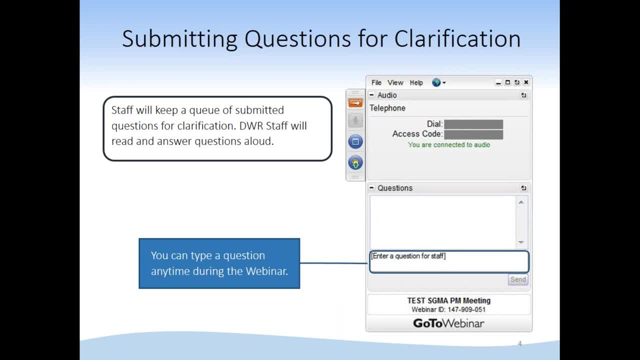 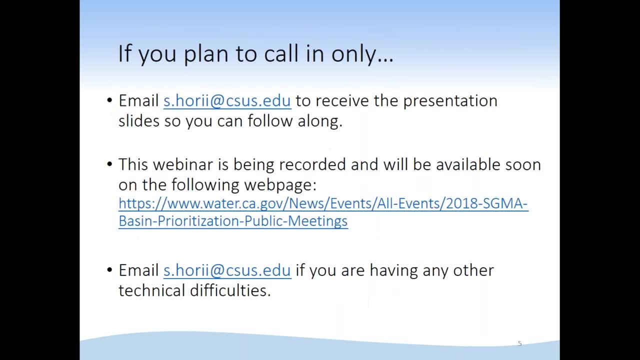 BWR staff will be keeping a queue of those questions and when we get into the clarifying questions- Q&A period, they will read your questions aloud. For those of you who plan to call in, only you can email me to receive a copy of the presentation slide. 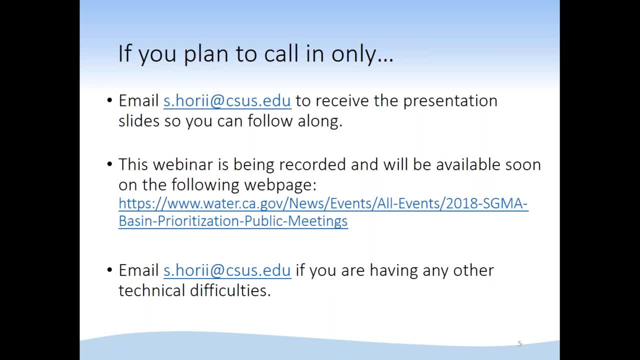 so that way you're able to follow along. That email is spelled SHORII at CSUSedu. That's going to be that same email address that you received When you registered for the webinar. and again, webinar is being recorded and will be posted to the webpage. 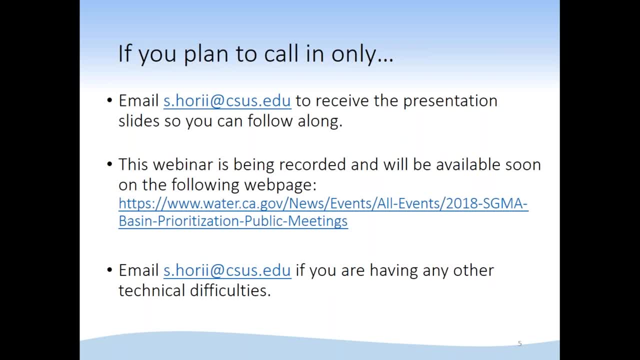 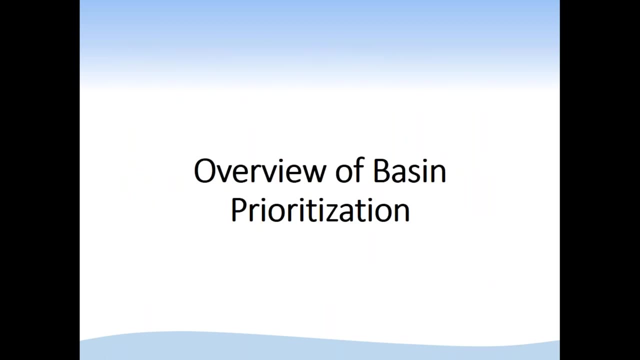 that, for those of you watching the webinar, is on your screen. So, and in general, if you are experiencing technical difficulties, feel free to reach out to me and I will help you as best as I can. With that. I'll turn it over to Trevor. 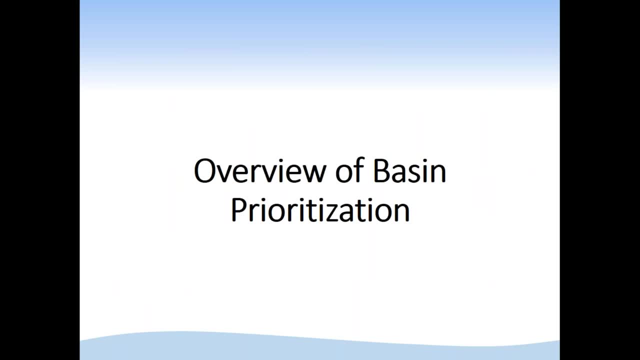 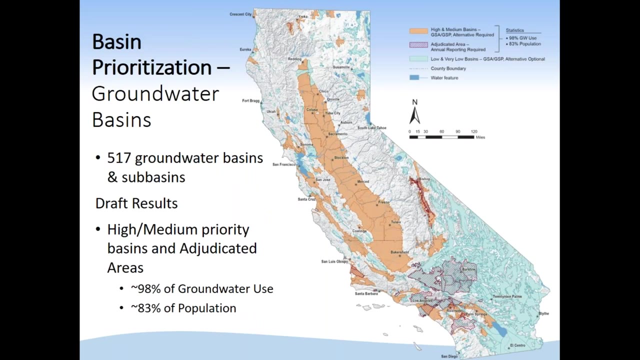 Okay, great, Thank you. So, as I mentioned, I will provide some background, some history and some of the legislative intent of the Basin Prioritization Project First, I'm actually going to start out with the draft results. So this is a map depicting the 517 groundwater basins or sub-basins throughout the state. 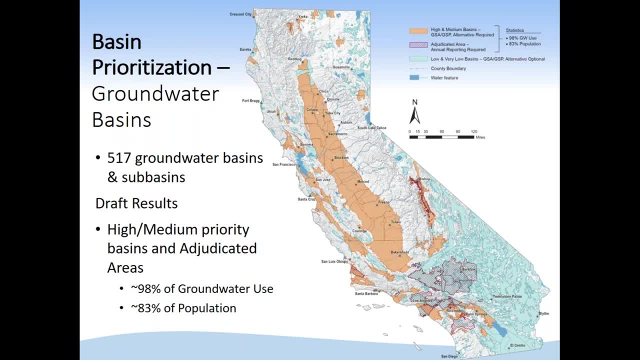 A little hard to see perhaps at this scale, but all of the orange colored areas are high or medium priority basins, which is a little hard to see at this scale, but all of the orange colored areas are high or medium priority basins. 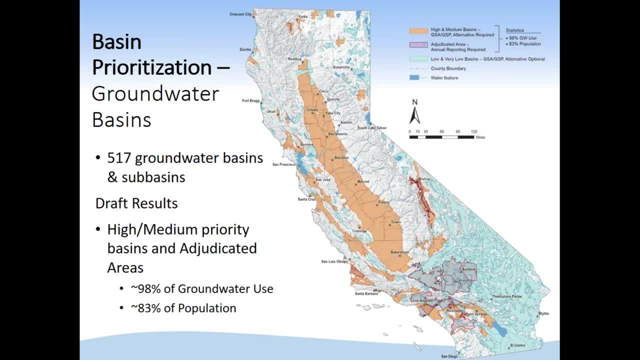 which have a special significance in the CASGEM program and the SGMA program. We will touch on that. The other basins shown in kind of a light green are low or very low and then the hatch pattern are adjudicated areas Also have kind of special requirements under the Sustainable Groundwater Management Act. 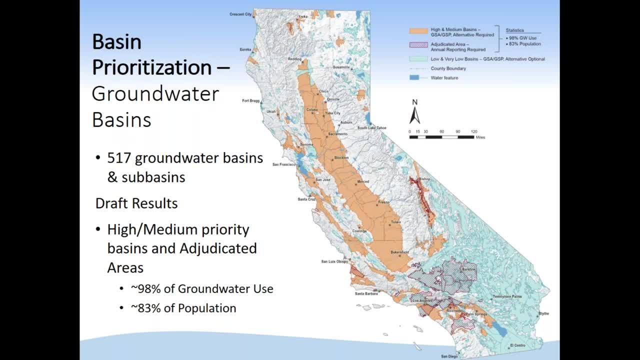 As I mentioned, there's 517 groundwater basins or sub-basins throughout the state currently and we've gone through a basin question prioritization process and have draft results that we will present the process and the information today. but the bottom line from a statewide perspective is: 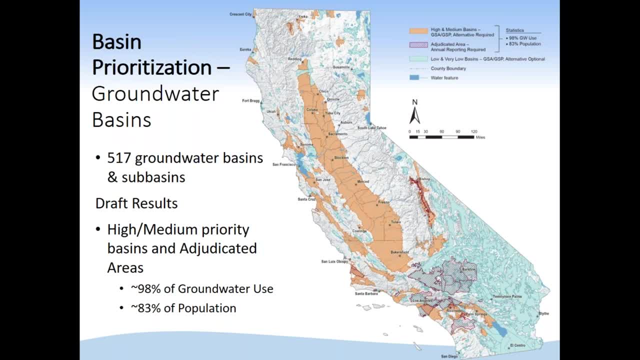 there were not significant changes from prior prioritization results, meaning approximately 10% of the basins or sub basins change priorities statewide. of course, we recognize that there's a lot of significance in terms of some of these changes at an individual basin scale and can certainly appreciate that. 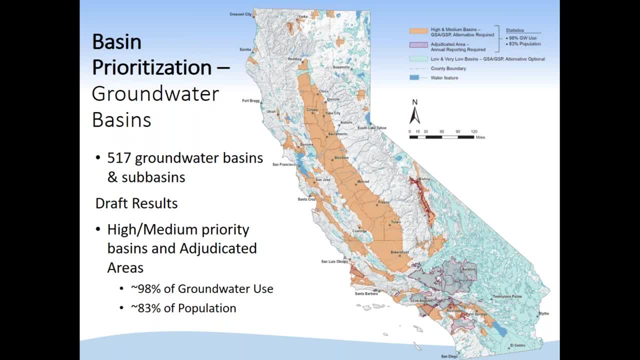 currently, based on these draft results, the high priority, high and medium priority basins and adjudicated areas represent approximately 98% of the groundwater use overlying or from those 517 groundwater basins and represent approximately 83% of the population that overlies those 517 groundwater basins or. 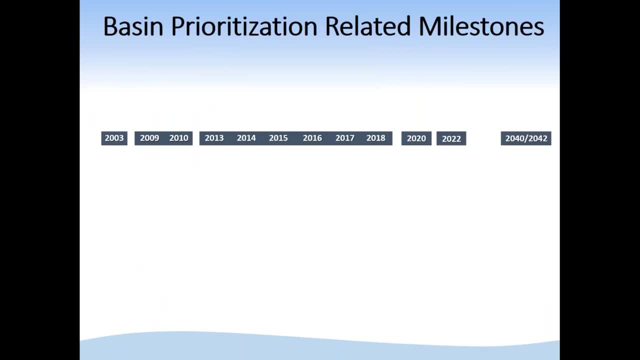 sub basins. So here's a timeline to characterize the major milestones related to basin prioritization. So first, important to note that basin boundaries are documented and defined in bulletin 118.. The last comprehensive bulletin 118 that the department has prepared was back in 2003.. Another significant 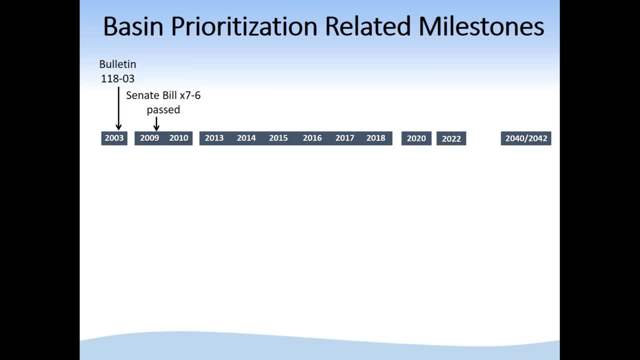 milestone was the passage of Senate bill x76, which really established the sustainable groundwater management program requiring the groundwater elevations be monitored seasonally. As I mentioned, the CASGEM program was initiated back in the 2010 timeframe really identified the extent groundwater elevation monitoring was required in each basin and directed DBBR to try to 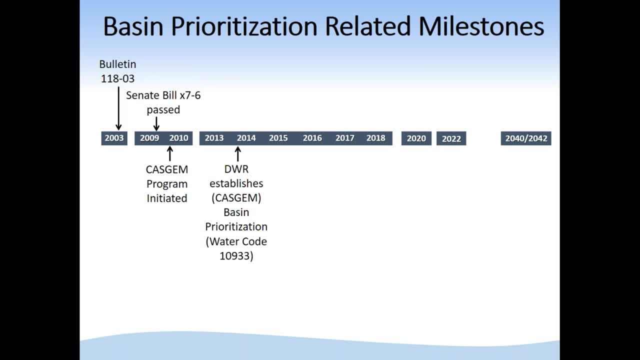 prioritize basins. Fast forward a little bit. the last basin prioritization related to the CASGEM program was what we call the 2014 basin prioritization. that was done in accordance with the requirements of Water Code 10933.. SGMA became effective January 1st 2015.. One of the significant requirements and 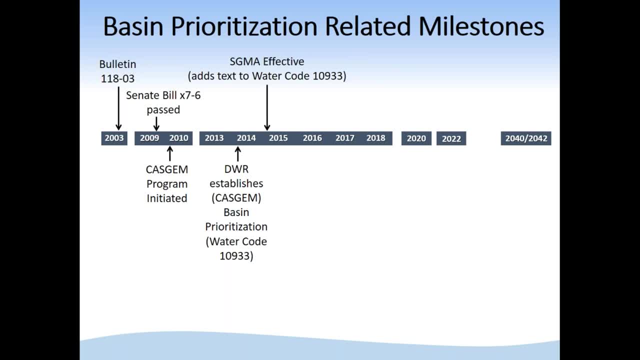 issues that SGMA identified was some addition added text to the Water Code 10933 that describes the specific requirements or criteria that department needs to evaluate when considering prioritization. In addition, SGMA required that DBBR identify prioritization of basins by January 31st. 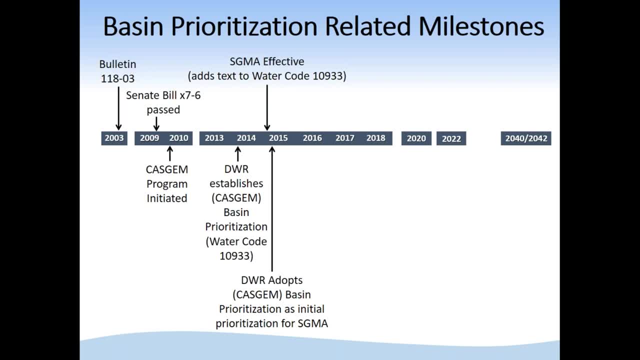 2015 for initial determination of which basins are required to form groundwater sustainability agencies and groundwater sustainability plans. At that time, DBBR adopted the CASGEM 2014 prioritization as the initial prioritization for that purpose. DBBR also modified basin boundaries under groundwater or. 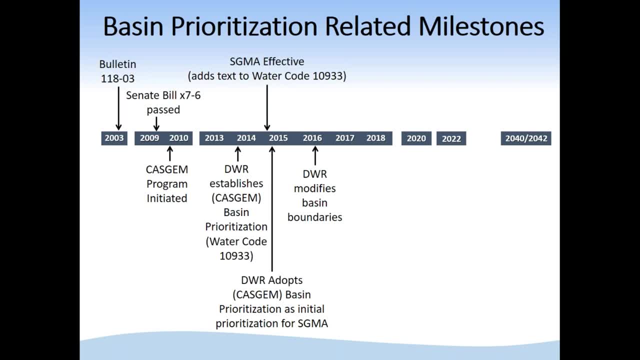 excuse me- under basin boundary regulations- emergency regulations- As you can see here, the basin boundaries are modified based on the regulations. Those boundaries were finalized in the fall 2016 time frame and we incorporated numerous statewide jurisdictional and scientific modifications at that time. DBBR then completed and published an in-term 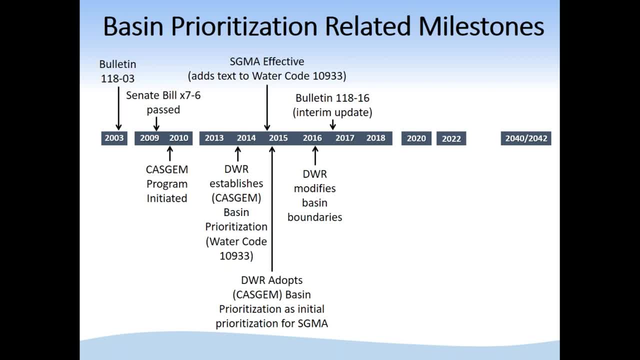 update of bulletin 118-16, which provides again those documented defined basin boundaries. This is led to the 2018 SGMA basin prioritization results- draft results that were released about a week and a half ago. I will get into the description of the legislative requirements in terms of why we've updated basin. 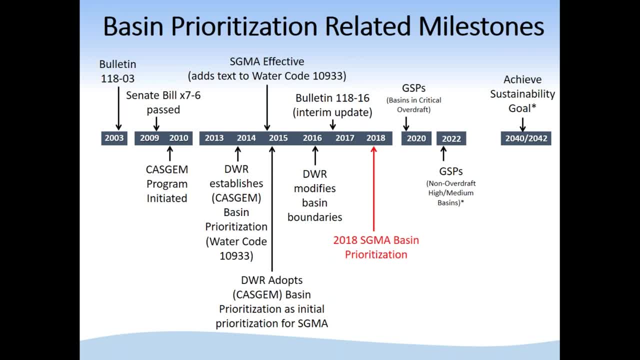 prioritization on subsequent slides. Of course, from a SGMA- Sustainable Ground Water Management Act- perspective, the Act clearly 값的目的: the requirements for GSA, from our sustainability agencies, to prepare, from our sustainability plans by certain deadlines for basins that are subject to. 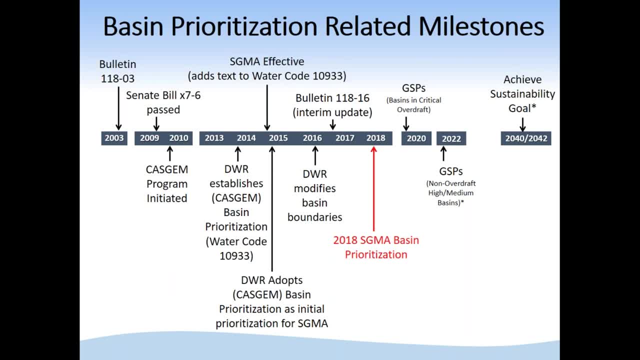 critically conditions of overdraft. that deadline is January 31st 2020. for all other high medium priority basins, that deadline is January 31st 2022 and, of course, those basins have 20 years to reach sustainability. it should be noted that Sigma also identifies a different time line for basins that change. 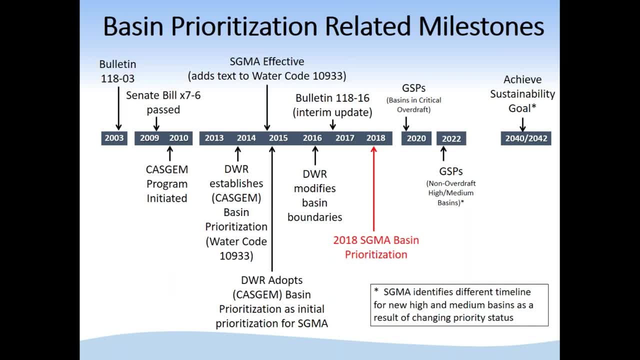 priority to high and medium as a result of base and prioritization, and so, as I mentioned, these are draft results at this time. Steven will touch on the next steps, but when these results become final, there will be different timelines for any basins that have moved to high and medium priority status. 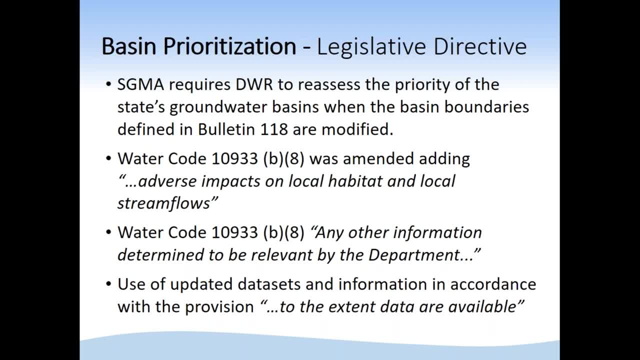 so the legislative direction under Sigma is articulated here. one Sigma requires that we reassess the priority of the state's groundwater basins when basin boundaries defined in bulletin 118 have been modified. in addition, the water code 10933 was amended with Sigma to include adverse impacts on local 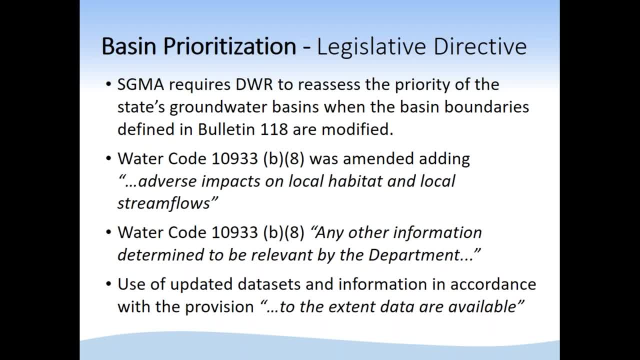 habitat and streamflow. third bullet indicates part of that water code section that describes that the department can look at other information determined relevant when completing based on prioritization. and finally, DWR has an obligation to look at updated data sets and information related to the provision to the extent. 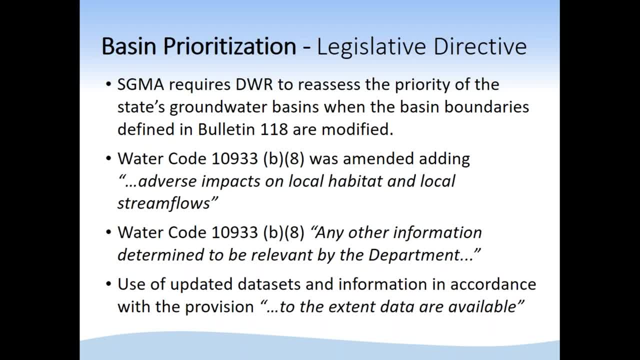 data are available. I should mention at this time that related to that third bullet with the Sigma 2018 prioritization process department looked at four factors that were not looked at at the time of the 2014 cash down prioritization. other information that we determined relevant with the 2018 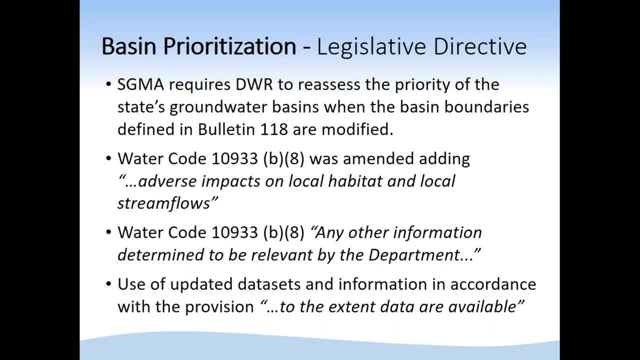 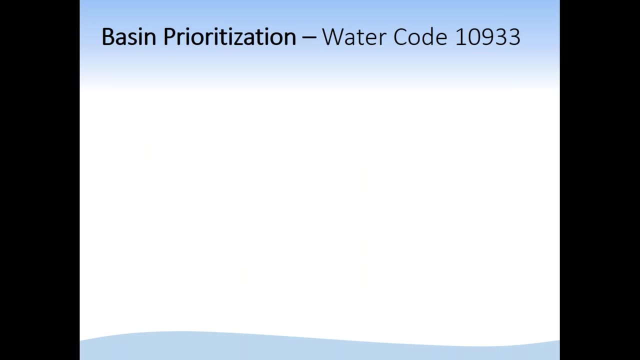 Sigma prioritization included the adverse impacts on local habitat and stream flows, looking at adjudicated areas and the non adjudicated portions of basins. where there are adjudicated areas, critically overdrafted status of basins and groundwater related transfers, and Rory will touch on more details related to these four additional factors on a subsequent slide. so water: 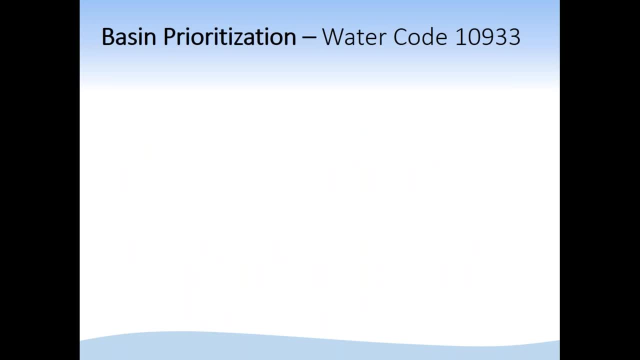 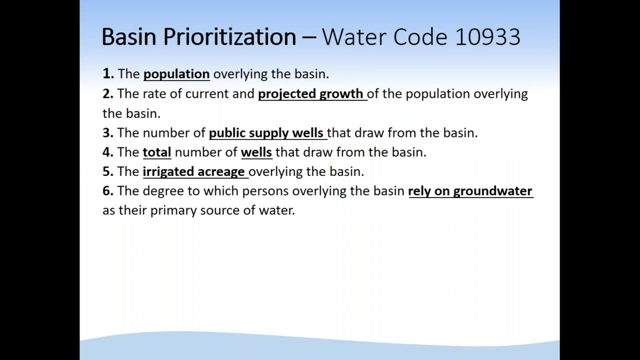 code 10933, the. the code that we need to follow in completion of our basin prioritization process includes one: the population overlying the basin. the projected growth related to the population. number of public supply wells that dry draw water from the basin. total number of wells that draw from the basin. irrigated acreage. the degree that the 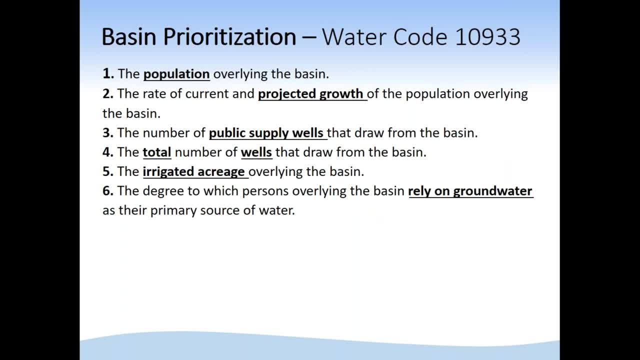 basins. persons overlying the basin rely on groundwater is the primary source of water. documented impacts. there are a number of other Esto. there are some additional details there in terms of what type of document impact, and then the aforementioned other information that we deemed relevant, including the adverse impacts on local habitat stream flow in Roy, will touch on. 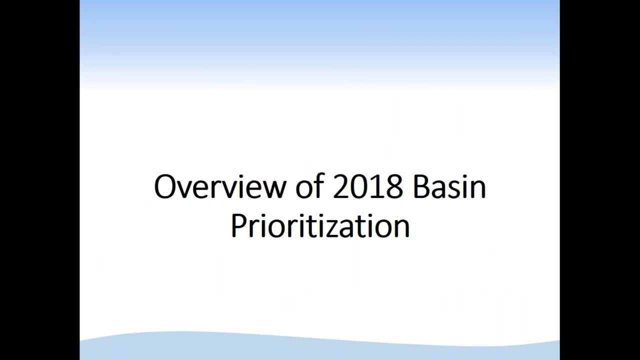 the process we used for each of those eight components or criteria and water code. I'll pass it over to Roy. good afternoon, this is Roy Hall and I'm going to cover all the different datasets. I'm not going to go in to two different data sets. I'm going to go into two cases that are water. 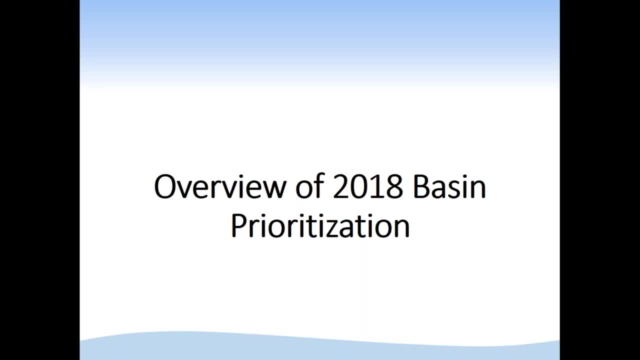 different data sets. I'm not going to go into two cases that are water and we're going to go into two much detail on the process because most of it is documented in the document that you can download from the website. but one of the things I do want to cover is 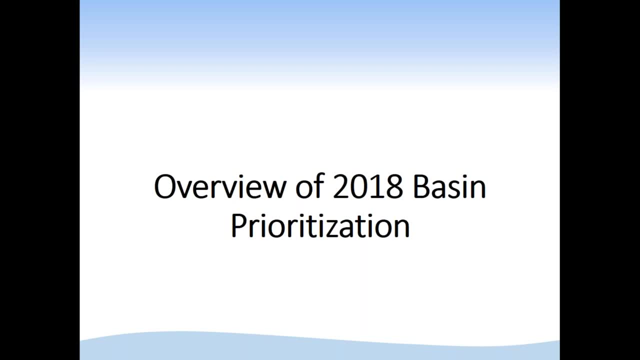 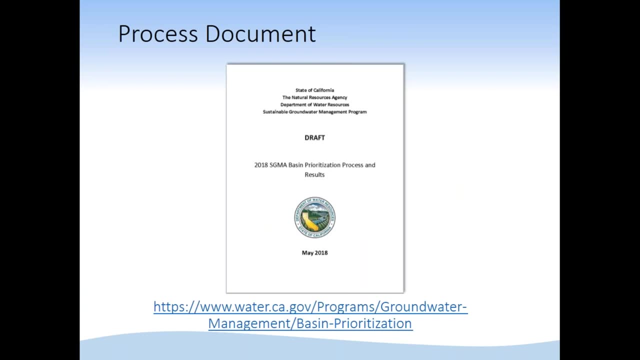 a lot of the different data sets and how they related to constructing the basin prioritization of 2018. as I said, here's the document. it's available. the website- on our website you can download it. it has all the pertinent information concerning each of the different components, broken down by components. 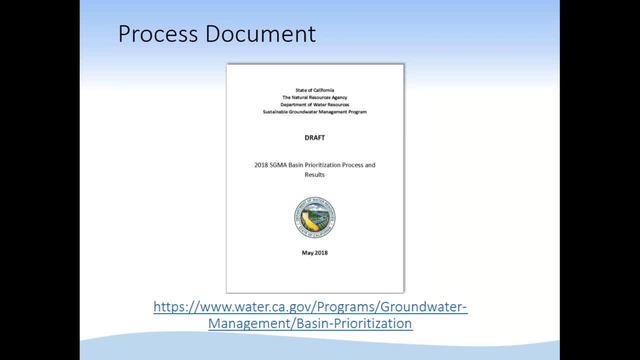 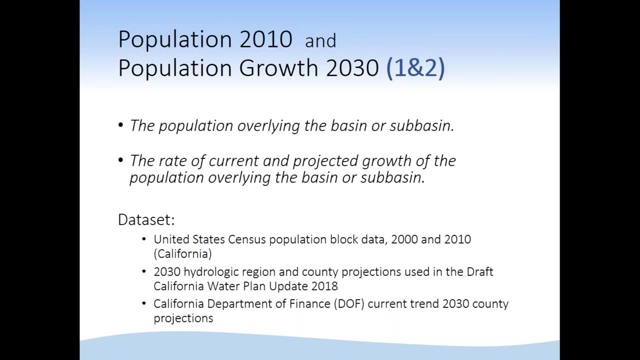 subcomponent levels, as well as any available appendices and things like that to help support the information provided. okay, I'm going to cover these in the order that they are covered in the technical document and also in the water code that Trevor just went through. on some of these, though, like on the 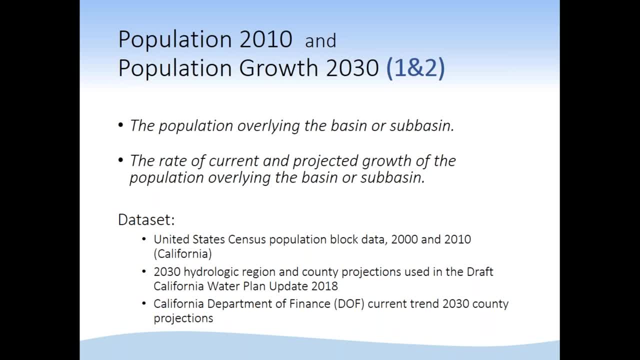 population, of population growth. a lot of the data was similar and shared in the process and the data was shared in the process and the data was shared in the process with the similar, so I'm going to cover them at the same time again. population over overlying the basin or sub basin: we use 2010 and we use the. 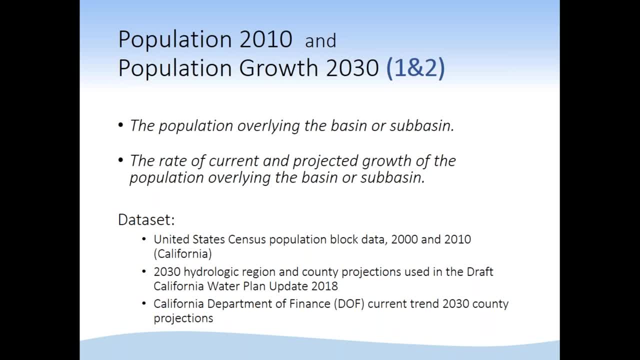 United States census block data. it was a. it was a. the biggest challenge there was intersecting those population blocks with respect to groundwater basin boundaries, but that was the basically that was the data set we used in the process. we used for calculating both 2000 and 2010. 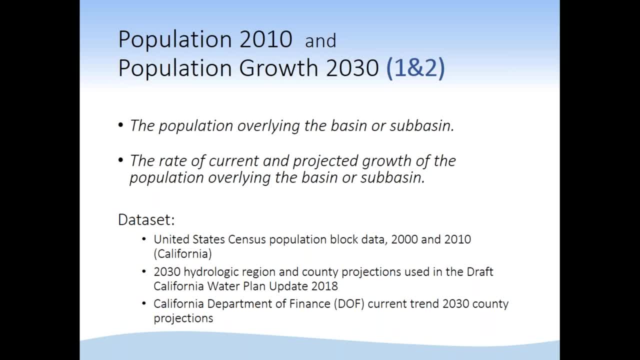 when we went into the rate of current and projected growth for the population overlying the groundwater basin, we had to do a little few more things that we used 2013 back in 2014 based on prioritization, so to maintain consistency between the two different. 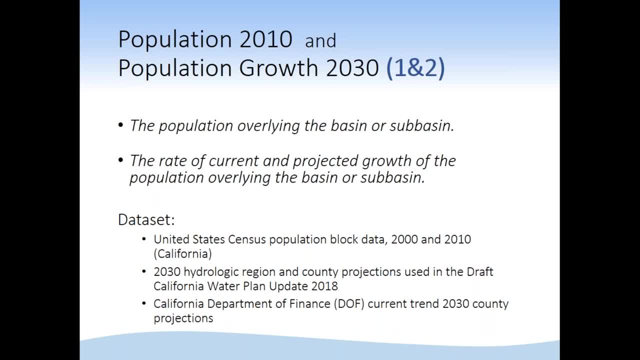 prioritizations. we maintain 2038 as well in just this process. in that process there was a big effort to try to maintain my with what we are projecting with respect to the California water plan and they do all their processing on a hydrologic region and county hydrologic region. 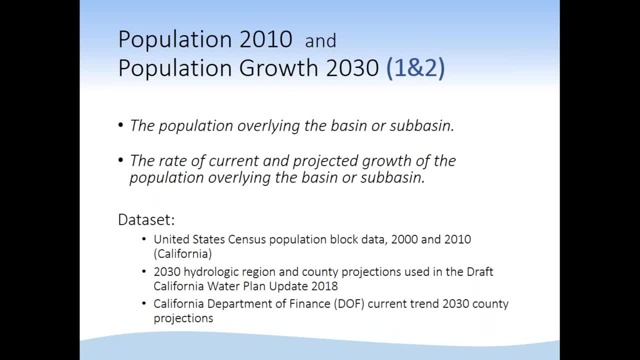 levels. so all we all we did in this process was basically inserting groundwater basins and reallocated all the different populations and the tables from the county Department of Finance so that, when we were all done, between basin and non-basin area within a hydrologic region came out to the same of 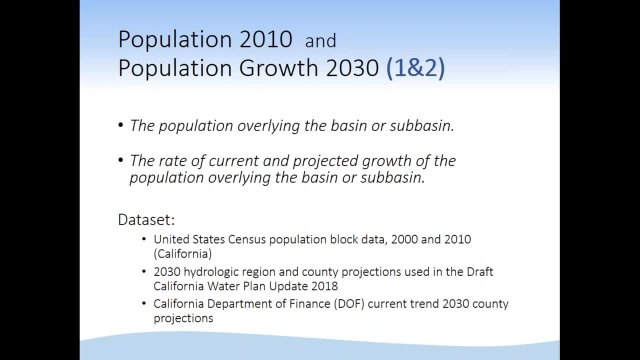 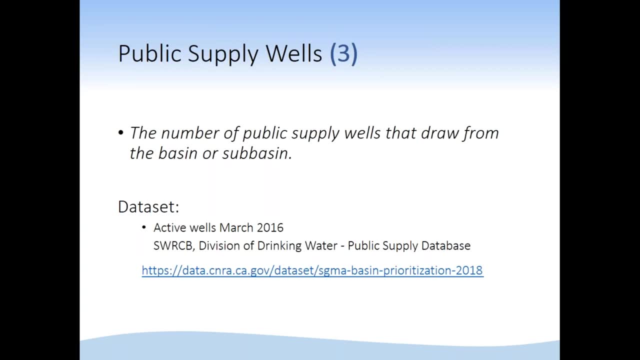 predictions that the water plan predicts for the particular hydrologic region. so it was more of a check and balance type process. public supply wells: we worked with the department, the state water resources control board. division of drinking water: we worked with those, the folks that were there back in 2016- to secure the data set that is behind all their public 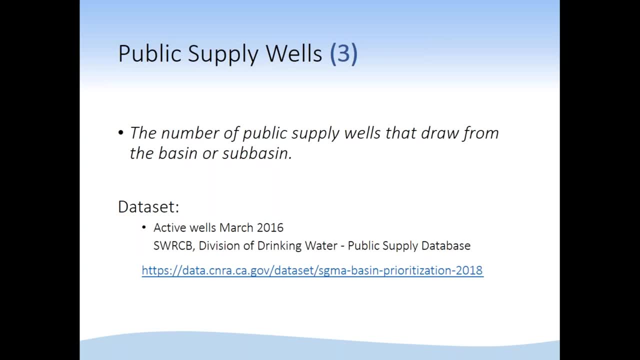 drinking water systems where they both get, collect information both on availability as well as water quality. so they provided us with their data that they had, and it's roughly about sixteen, seventeen thousand different public supply wells throughout the state by the time we were done with it. with what? 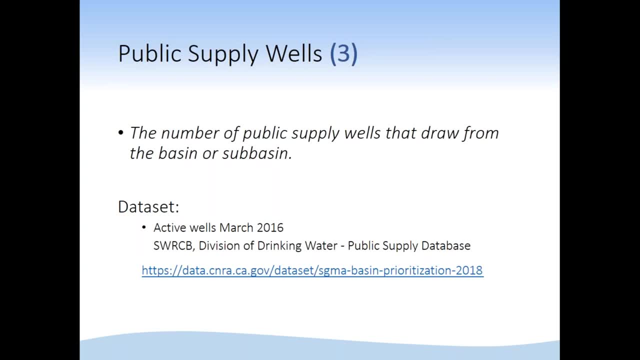 was in groundwater basins. a number of rough was roughly about eleven thousand wells are scattered throughout 517 basins. that data set is going to be available on our segment basin prioritization open portal website. if it's not there yet, it will be there shortly, within the next day. a couple 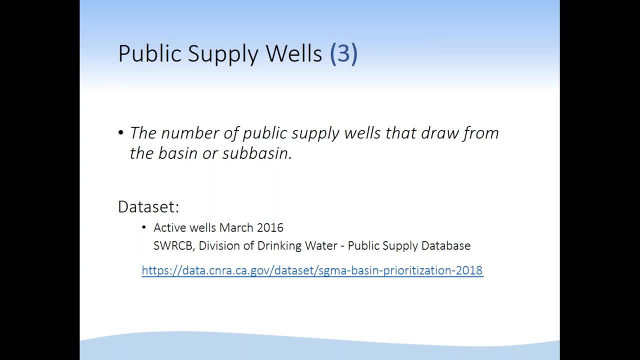 days, but you'll be able to download it and then it's sorted. it's an Excel spreadsheet, each one of those spreadsheets, so it'll be a zip file and it'll be based off of the state water resources control board. they have divisions, regions for the 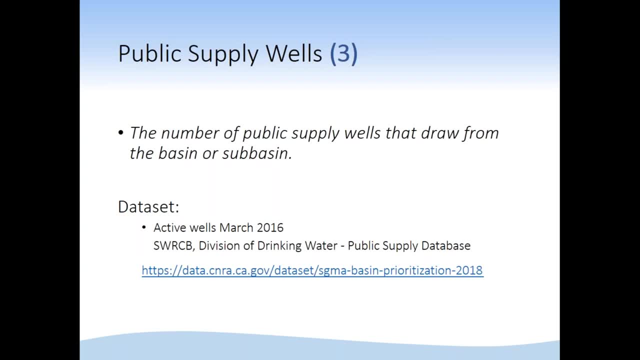 regional quality water quality board, which also corresponds to our basin ID. so when you see a 1-0 0, 1, that means it's the region board, regional board, zone 1. anyway, they're all broken up into one through nine. so if your basin starts, 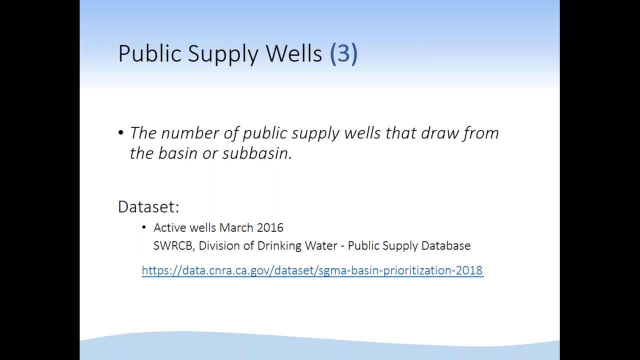 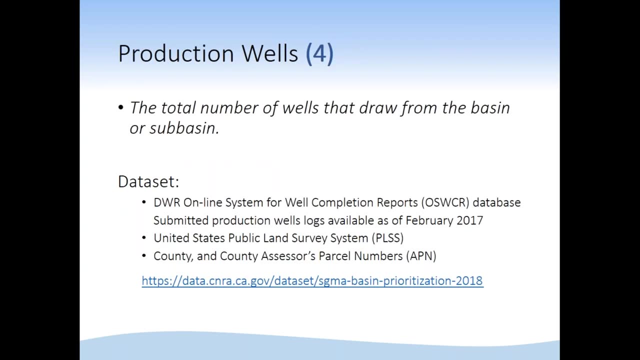 with a forward look to the forest, and they'll all be in. they'll all be available here in the next couple of days. production wells: we pulled the data on this particular requirement from our Oscar, which is the online system for well completion reports. we pulled it back in February 2017 at the conclusion of. they had a huge effort to digitize. 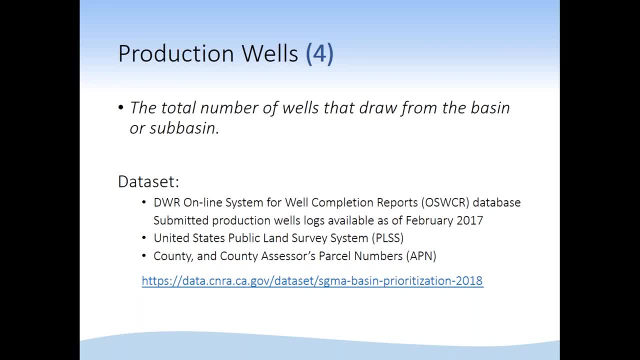 scan and key a lot of well logs that were not previously in the state water system. so I was waiting until that was completed. after they added about another two or three hundred thousand well logs, then we kind of pulled that system out in order. our well logs are all categorized and labeled and spatially. 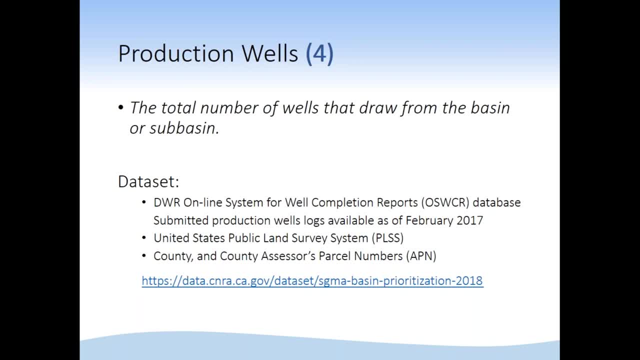 down to township range section in most cases. so that means each one, each one of those wells that are identified in that log at a minimum is one square mile. we know where that well is. so that kind of led to how many of them are in the basin when they are in one square mile at a minimum. 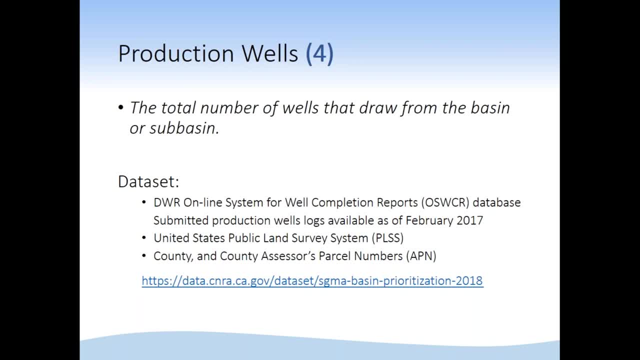 some of them are even much greater than that, because they only give us township range, which then means that, well, somewhere within 36 square miles. so with the use of the public land survey system for mapping these and county and assess or parcel numbers, we were using all the, all the clues we could possibly do to. 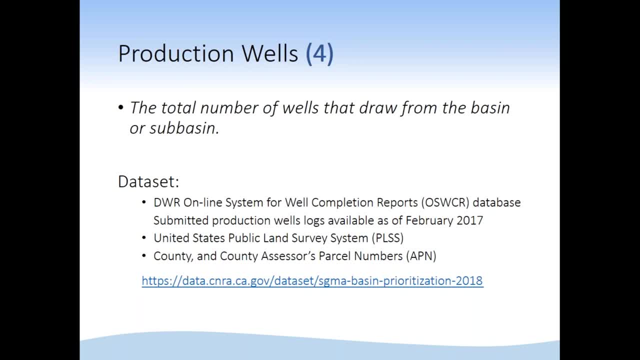 try to figure out where these wells were located within a, within any reasonable certainty, of one square mile. now, the sections which are identified in the public land system have are either in one of two things, and the document goes into this a little bit more than what I'm going to go into here. it's: 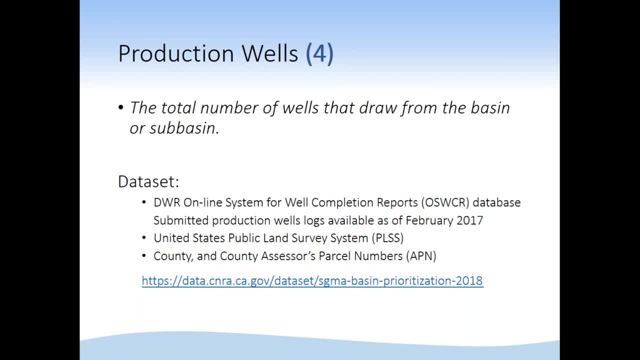 either completely within a basin, which means any all the wells that are identified within that section are assigned to that basin, and if it, if it crosses a boundary say, between two basins, then we simply did a proportion between the two, and in some cases it was three basins in other. 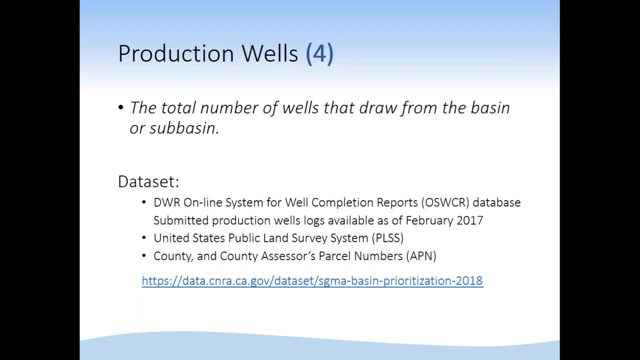 cases it's somewhere in and out of basins. so we only allocated a portion of those. but we don't know exactly which wells are in which where within that section. so that was the best we could. that was the best we could zero in on that. the parcel numbers would allow us to go into a little bit more little. 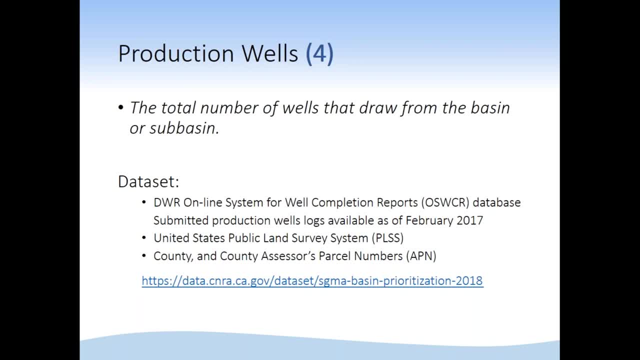 parcel numbers or parcel locations and be able to identify where these wells are actually. that complete data set again will be in a zip file that you'll be able to download to the whole state here in the next few days. I have a preliminary copy of it. I need to go through and do some QC on it before I can post it as soon as. 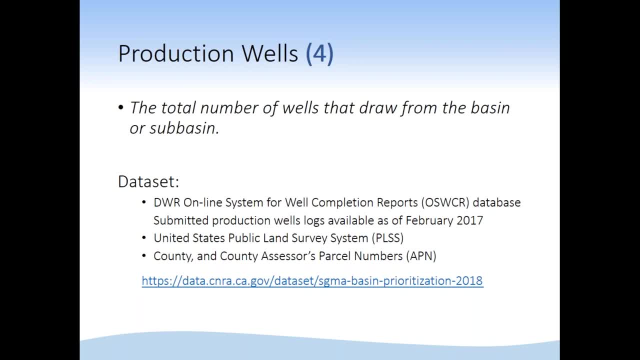 it would get up there would be tomorrow, but it would probably be either later this week or first of next week. same website, same location. before I go off of that, then the next piece of information about that particular process would be: after we figured out where they were, then the next step would be: were those? 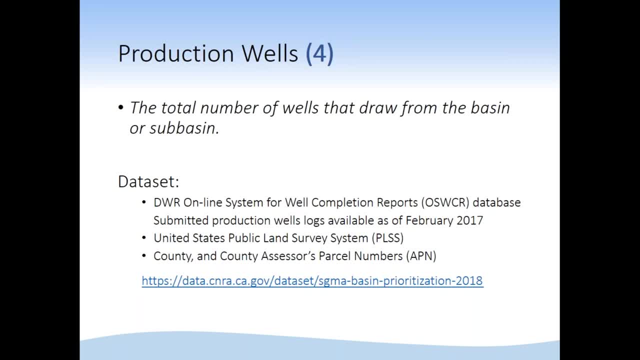 were they production wells or were they monitoring wells you got? you need to understand that these well logs are submitted by drillers and other entities and they're not always clear exactly what the well use, what the well use is or or was unreadable or it was a faded copy, things like that. there's a lot of. 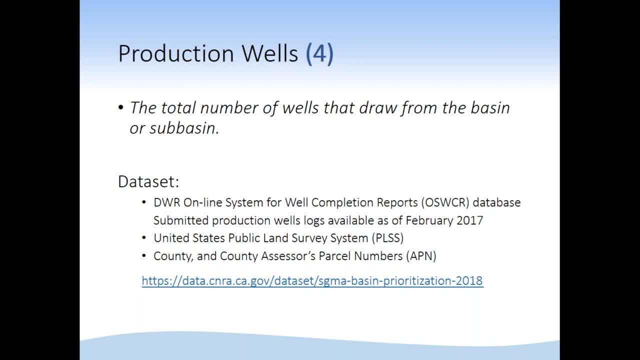 reasons for that. so we had to come up with a couple of different analysts, basically looked at the information provided to be able to make a determination based off well depth screening intervals, groundwater- excuse me, gallons per minute, casing sizes, things like that that help us identify what looks, what is obviously a production well versus what is obviously. 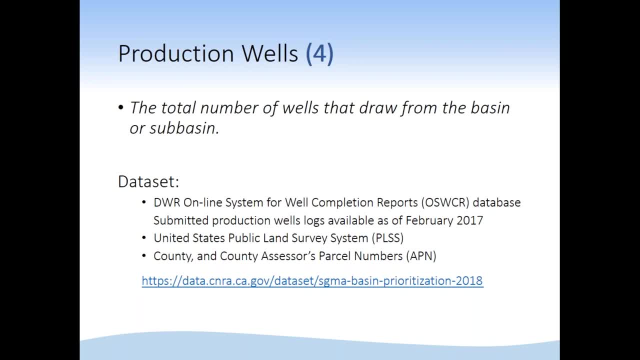 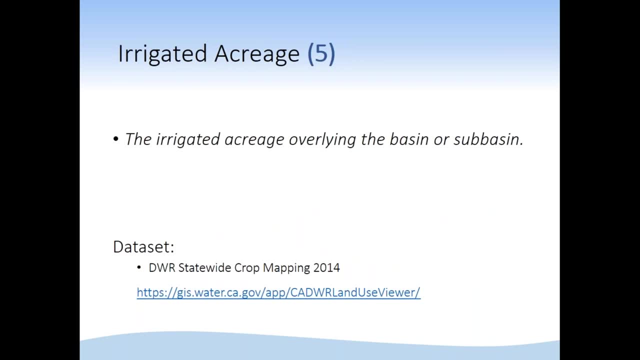 a monitoring well or a non producing well. so we let kind of the last question that we have- and I think it may sound a little underrated that i'm not fully off on it, i'm not totally sure you guys work with with land iq and we developed a lot of stuff. I go further. 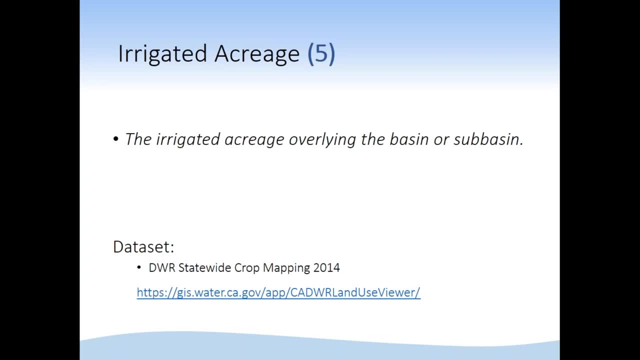 back in 2014. we use basically exclusively DWR surveys for all the lane use, but they they don't cover the same year. they are over span of years across the state. so it was really difficult for us to get a more accurate, consistent 117 basins, and so we worked with land IQ who did a remote sensing for us to 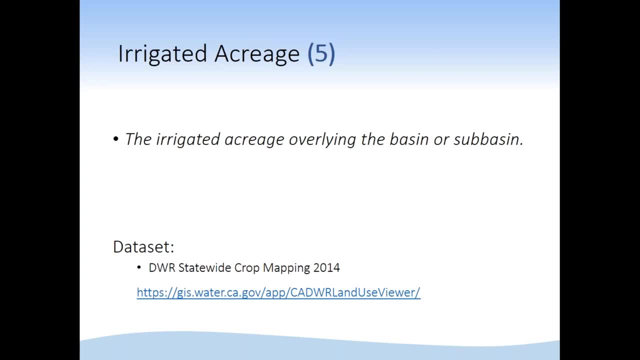 basically map the entire state of California for us for the for a particular year in the first year that they provided us data was 2014, which was also very good because it also is that transition before, not excuse me, it was the transition of pre Sigma and policy, so it was worked out really nice from. 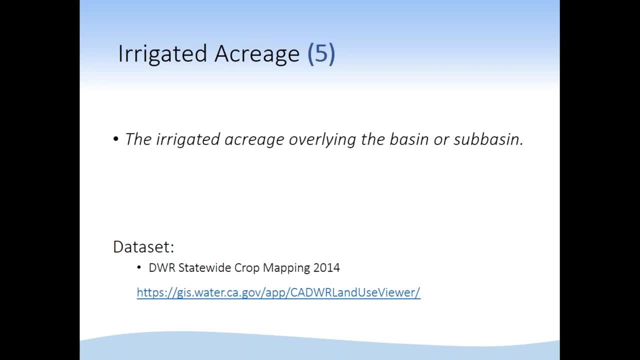 that standpoint. that data set has been available for download and it's available for anybody. the website is on the bottom here. it's been there for less seven or eight months. it's a and we use that data set for both. this, obviously, this particular component, but it was also used in the groundwater reliance. 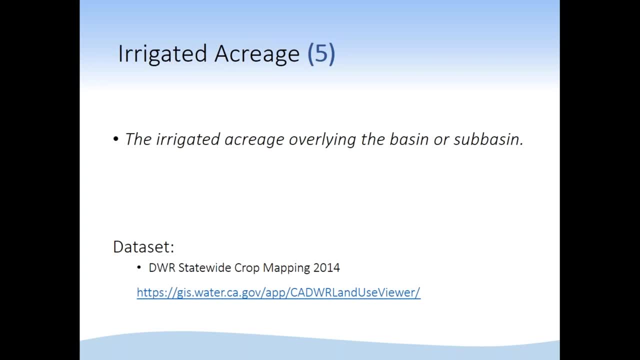 section of the of this processing all the all the land map in that particular data site is considered irrigated acreage. we did do some post processing on the base and prioritization data on places where we knew there was dry farming. that was not evidently clear for remote sensing and we also made some 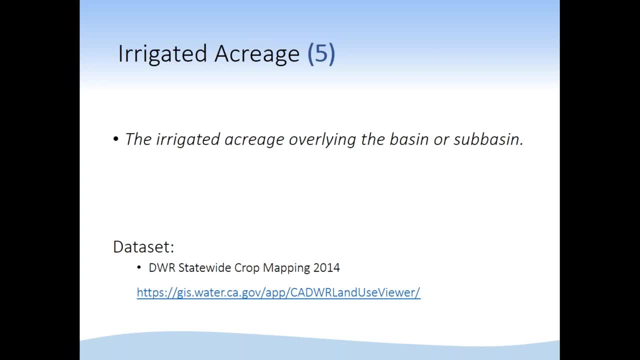 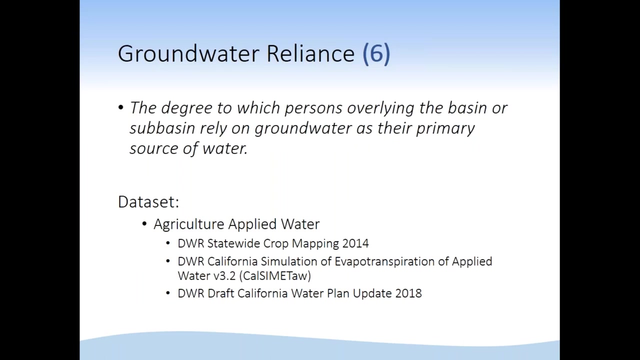 adjustments on some pasture lands that are not irrigated there. they're also kind of like dry farming anyway. so those were post processing that only applied to base and prioritization, but currently all that data is still up there, as is groundwater reliance. there's actually two pieces to this. one is the 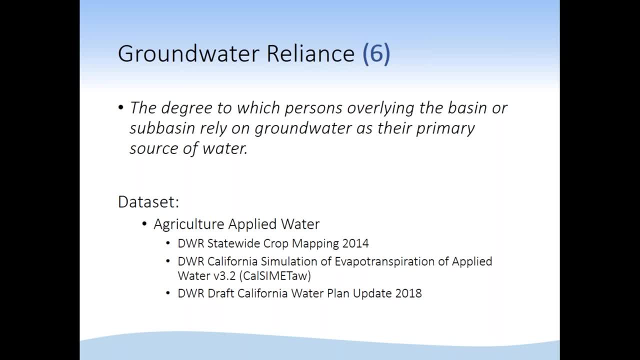 volume of groundwater, that is, is used by the basin, and the other one is the percent of that groundwater is reliant upon in that ground, in that groundwater basin. essentially we call it 6a and then 6b is the percent 6a drives 6b you. 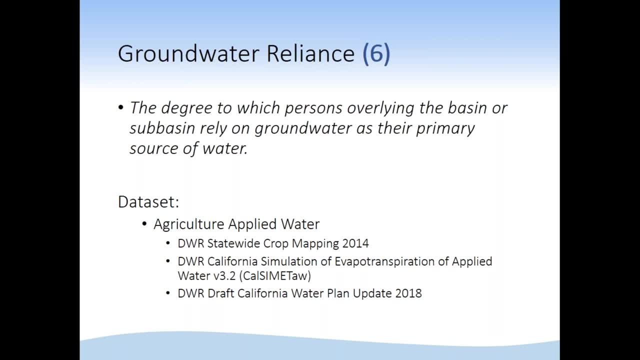 know, 6b drives 6b and then 6b drives 6b, and then 6b drives 6b and then 6b drives 6b. so we didn't do anything special with 6b other than take the results of 6a and 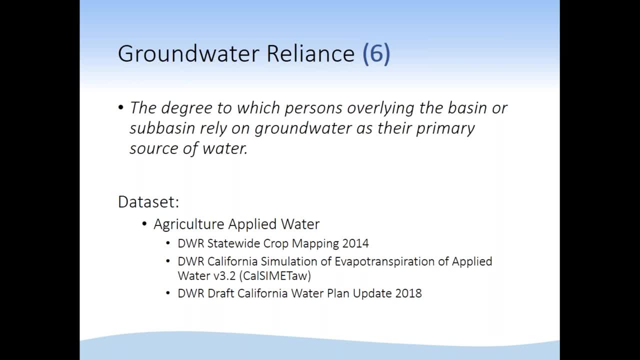 do some and do the calculations for percents, but anyway. so 6a is broken into agricultural and urban. I'll cover the agricultural first. again, we use that land IQ statewide cropping map from 2014 to identify all the crops in the basin and all the acreage and then, through the calcium etah we developed 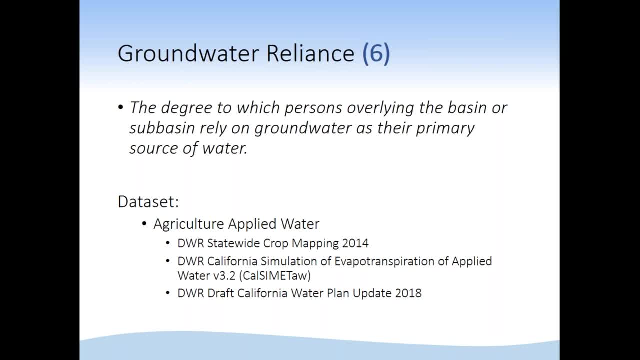 by base and all the unit values for all the crops, that basically one acre, one acre of X crop uses this much water within that basin and from that then we basically took the ground for the cropping maps and the totals to determine the the applied water and then, using the work that they've been working, 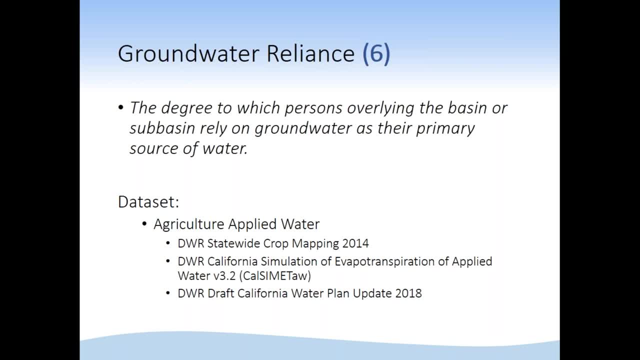 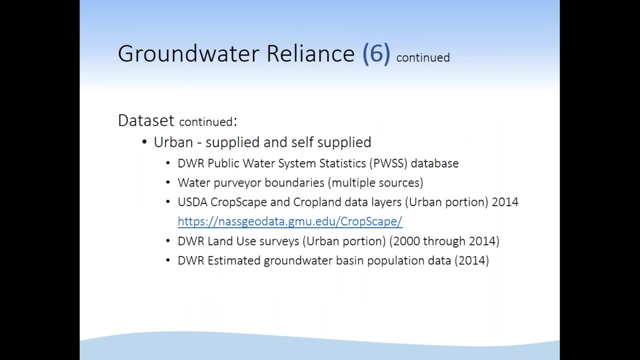 on with respect to the water plan 2018. we use their water balance information to try to determine what is the ratio between surface water and groundwater. so that's where that information came from. on the urban, urban was a little bit more complicated. we had to use quite a few more different data sets to get to where 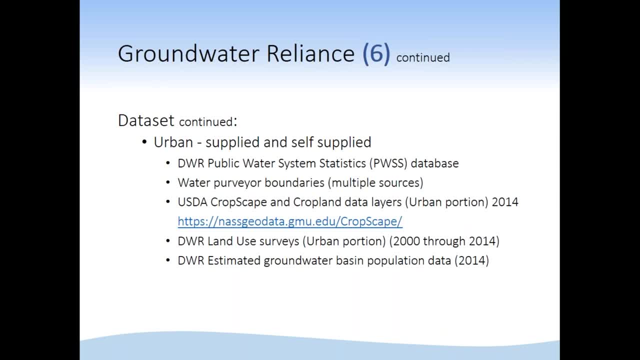 we wanted to be with that one. the first was the what we call the DWR- public water system statistics database, which is actually a poll from the water board. all the purveyors are required to produce annual reports. that has a lot of different pieces of data that they're required to report and we generally just 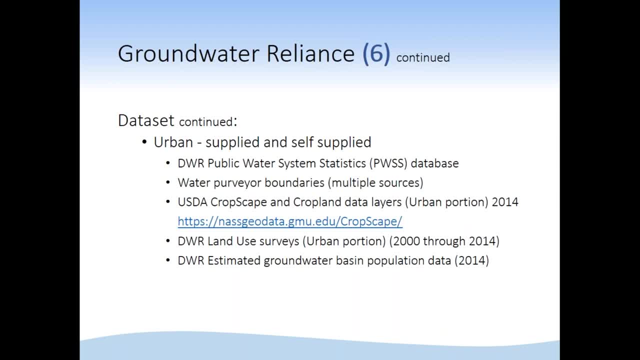 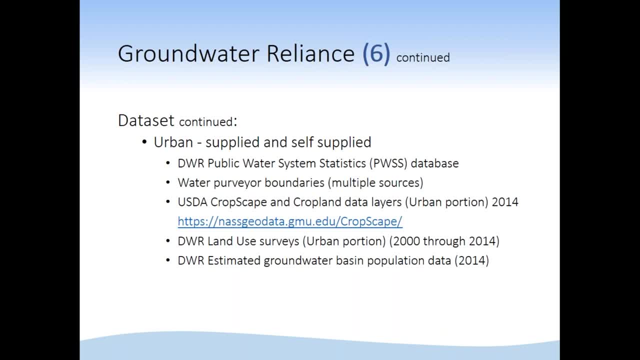 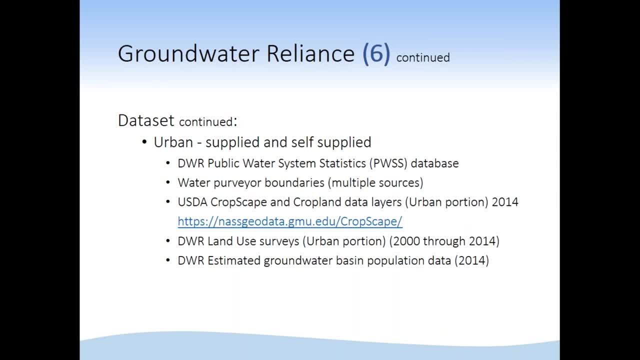 supplied by the actual water purveyors, or we, or they're created by us, or their, or they're created by somebody else. anyway, we use there. they come from multiple sources. these are all the different water district boundaries. then we created a, an urban layer that was a little bit more detailed. 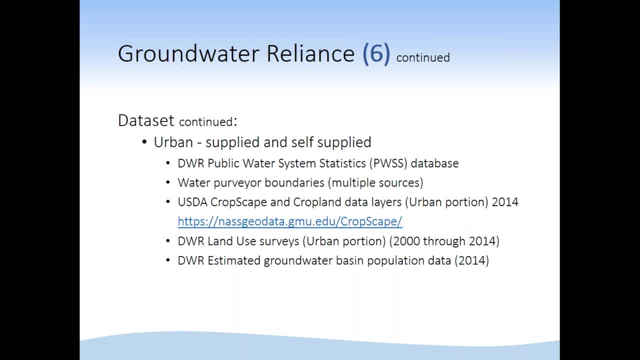 then, what you're going to find in your traditional urban layers that you can download from various sources. we started with DWR land use surveys because they're highly detailed with respect to where urban is located, and so we use any surveys that were done between 2000 and 2014 that mapped out urban layers that 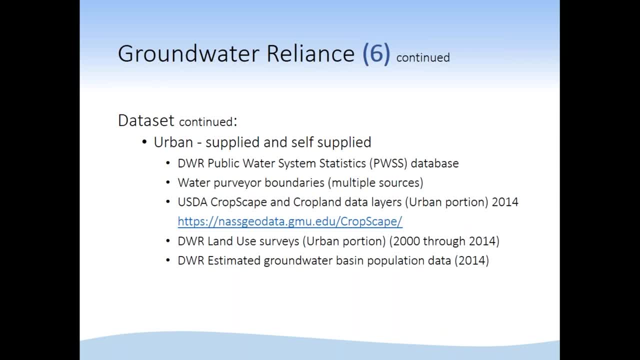 was the primary data set that we used, and then we backfilled anything that came out of USDA crop scape cross layer that was mapped as urban. so then we, between those two data sets, we were able to have a pretty good idea of where all the urban is in there. so you're asking: so what do we need that for? and that is: 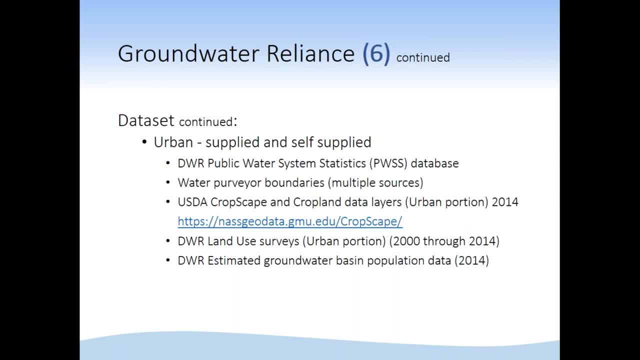 a very good question. let's say we use that to fine-tune a lot of the urban purveyor layers that we had, because most of them are not most of them, but there was quite a few of them that we were able to find, that we were able to find. 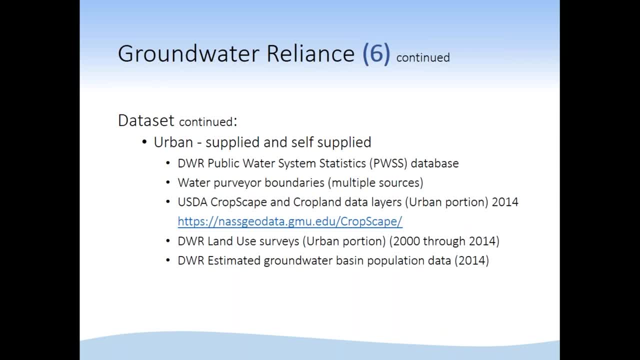 some of them that have. they're just big, they're block areas, while there's areas within those urban, those purveyors that are not services there either parts, or they're undeveloped things of that nature and we have to be able to understand, because most of these water purveyors do not. they're not always 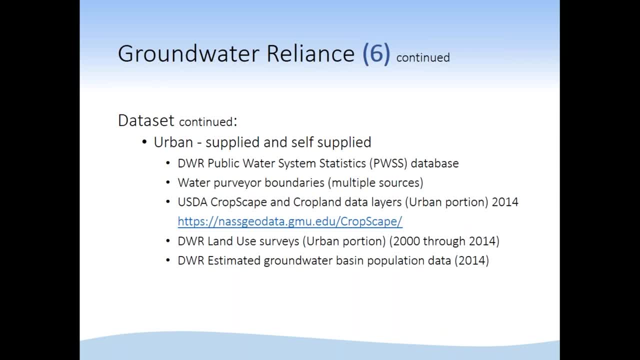 located completely within groundwater basin. they straddle multiple basins and they can also straddle non-basin areas, so to get an accurate representation of the actual area, we needed to exclude some of the areas that are basically undeveloped. the next part that we had to do: we had to estimate population, so we 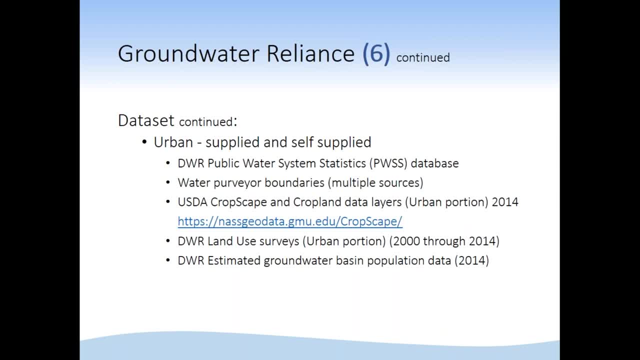 used a tool that's documented in the draft manual that basically created a 2014 population estimate for us, because that's really critical for us to determine whether how much of that water is going to be in that area. so we had to much the urban users are providing to. 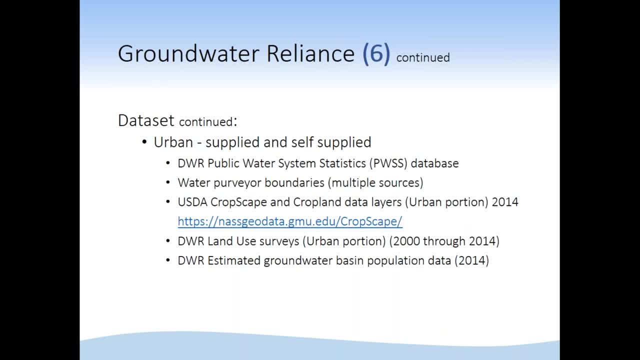 So if you have 20,000 people living in the basin and the urban providers are only supplying 10,000, that means there's roughly 10,000 people that are on self-supply. So we needed to be able to break that down in that fashion, because there are 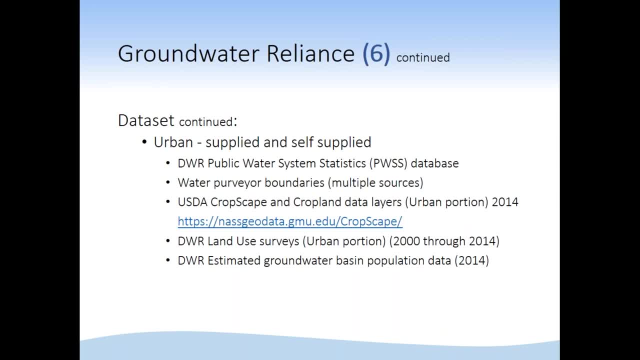 self-suppliers, in both domestic and commercial, that we had to take into consideration. So between that and the urban providers, we were able to determine how much water was being used and supplied for urban needs- groundwater Before I go. So anyway, these two data sets were basically the groundwater volume was. 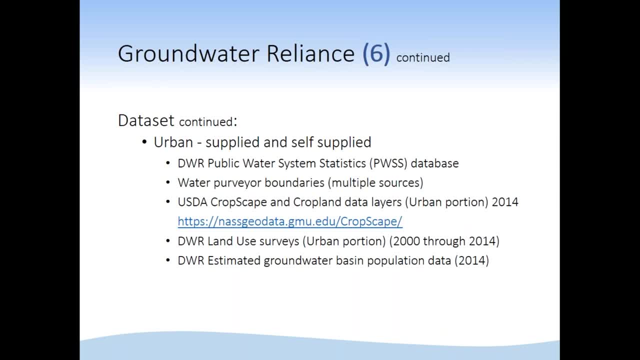 added together from both ag and urban and then we basically templated it up and we ran it through the breakpoints that were pretty standard and consistent with all the previous data, The previous basin prioritization, And then we took the total water demand for both ag and urban to come up with a 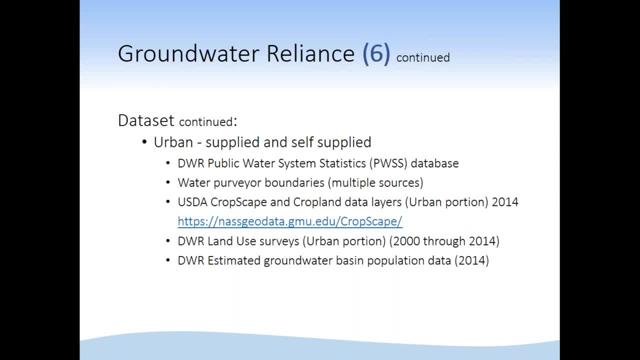 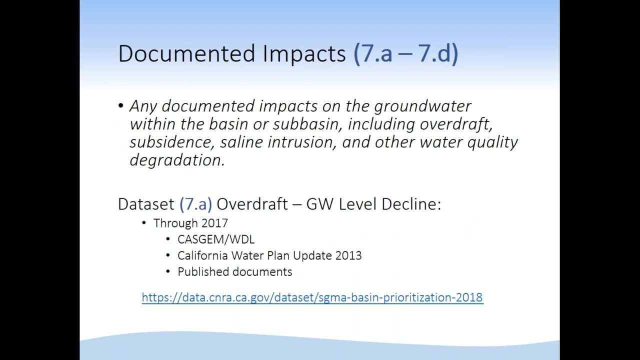 whole total water demand and then we just basically did the simple divide to come up with percent for groundwater volume Documented impacts. We broke that into four separate categories: A, B, C and D. Please excuse me if I keep referring to A, B, C. 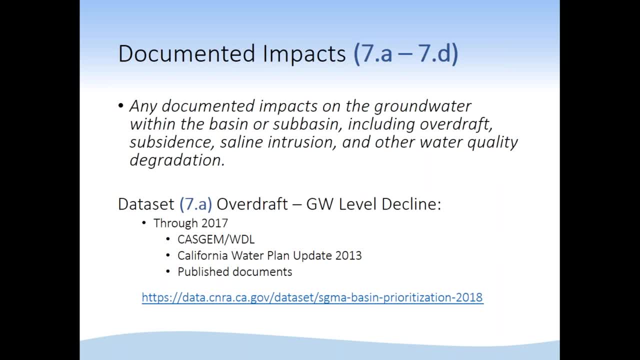 I'm sure you're not familiar with them as much as I am, But anyway, A is basically referencing overdraft in the water code. groundwater level. decline in hours. Excuse me, B would be the subsidence, C would be the saline intrusion. 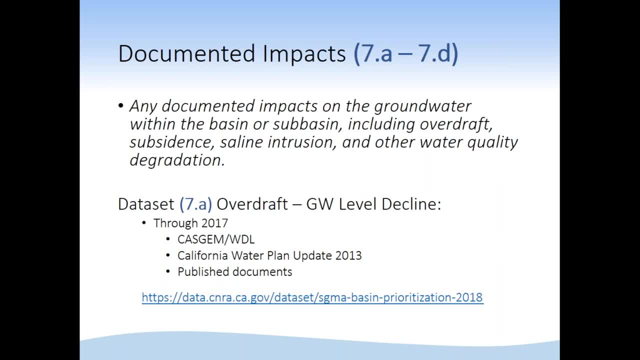 And D would cover the water quality degradation process, So I'll cover each one. A, B, C and D. Data sets for groundwater decline was a research project, Essentially looking through all the well logs that we have. excuse me, all the water. 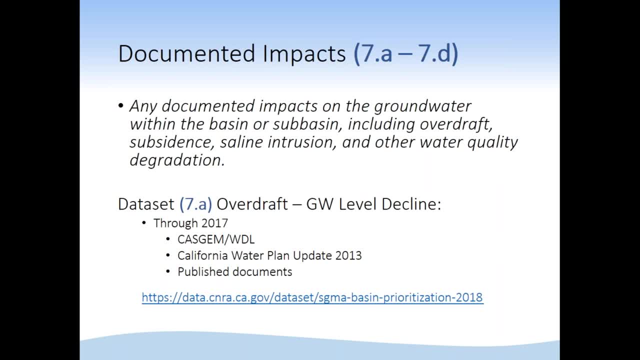 level data that we have both in CASGEM and Water Data Library. we looked at information that we could find with respect to the groundwater water plan update for 2013 that we worked on, as well as published documents, both regional and local. 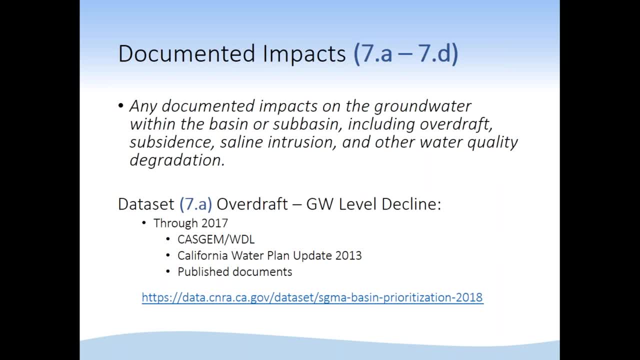 Right now there's just for all four of these categories. There's a downloadable spreadsheet with all the information concerning all the documented impacts. So it's either a document that we possess here or it's a document that is linked outside to an outside source. 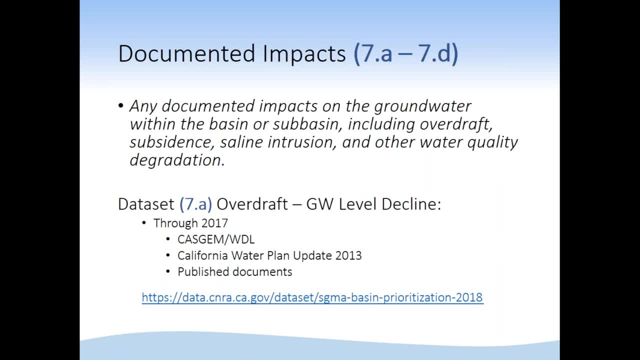 Currently, what we're doing is pulling all those documents, even those that are linked into a single data set that will also be put on the website, So you'll be able to download all the documents that were used, and not necessarily the only ones. 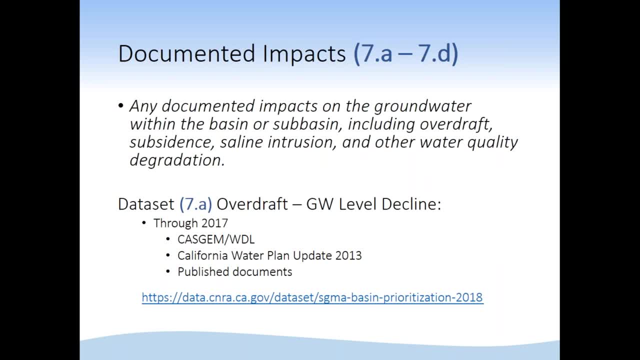 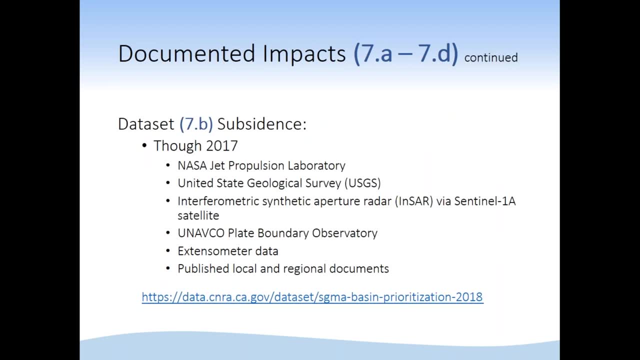 But we've also done some in-links and we've also done again, we've done some in-links with the data set for what comes in before this, but those are for what needs to come in And that's a way that we're able to rely on links that have a tendency to go stale. 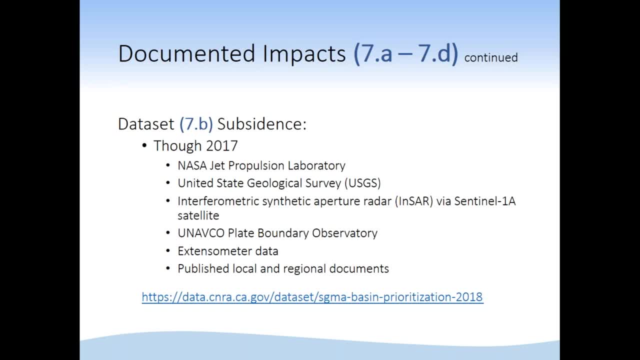 get broken over time, Which is very annoying. Okay, we're now on B subsidence. This is subsidence through 2017.. Primary data sets that we used: We used a lot of information from USGS, which is also part of that INSAR, with respect to 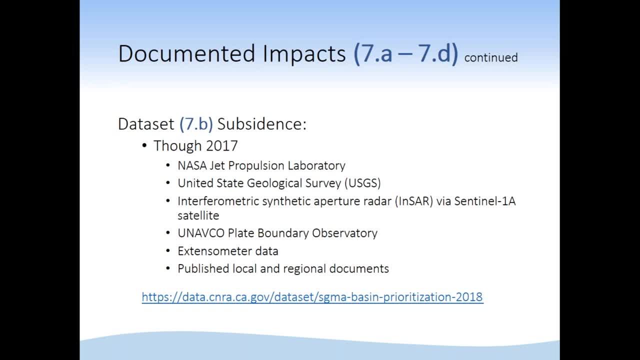 USGS But there's been INSAR, especially in the Central Valley and on the Central Coast. there was some INSAR data that we were using. The plate boundary observation was an excellent source, especially in Southern California, to look at various locations to try to fine-tune with what we're looking at to see if it. 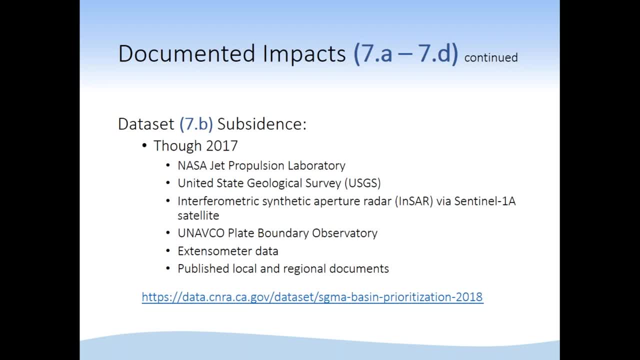 doesn't make any sense, things like that, So we tried to use those as much as possible. They're also located throughout the rest of the state- Central Valley For plate tectonics. California is a very active state. Things are moving. 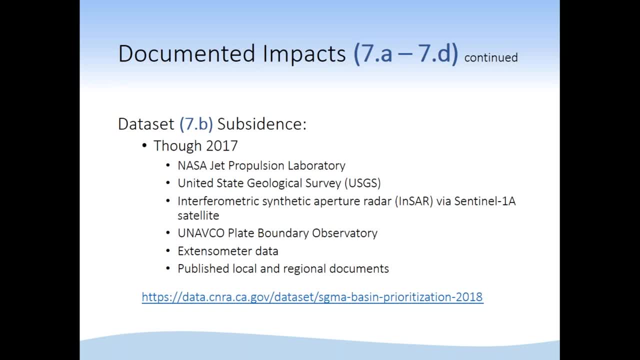 So it gives us the X, Y and Z axis in a lot of locations, But they are point data and they're situated in places where they're expecting to see plate movement And they're moving And we just try to piggyback on that information as well. 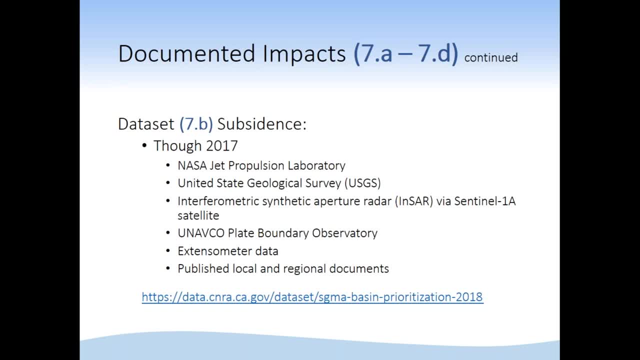 We also have extensometers, mostly throughout the Central Valley. We looked at that information as well and then published local and regional documents that we could find Again. all that will be shortly available as part of the documentation package that will be offered. Saline intrusion. this is another one where it was mostly published local and regional. 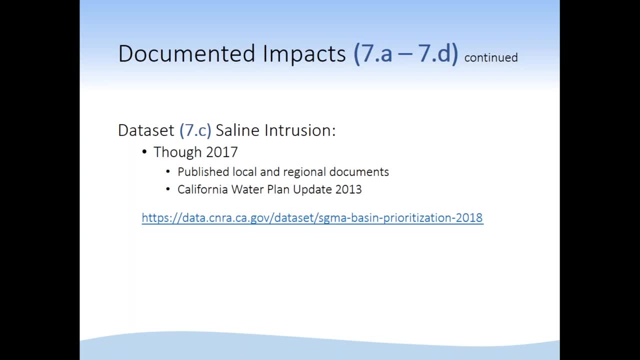 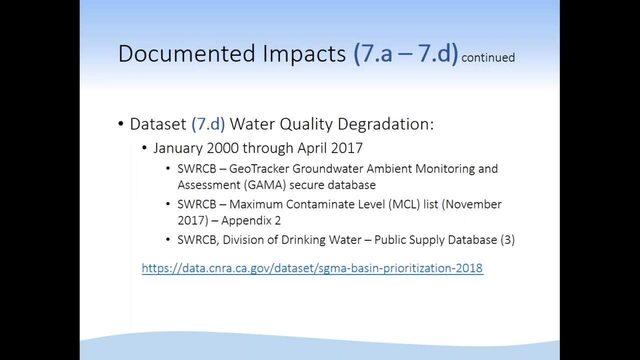 documents. We also looked at California: California Water Plan and groundwater update 2013.. This affects mostly not affects, but most of the places that were susceptible to saline intrusion were obviously coastal and then around the Bay, The Bay area has some interesting areas in it. 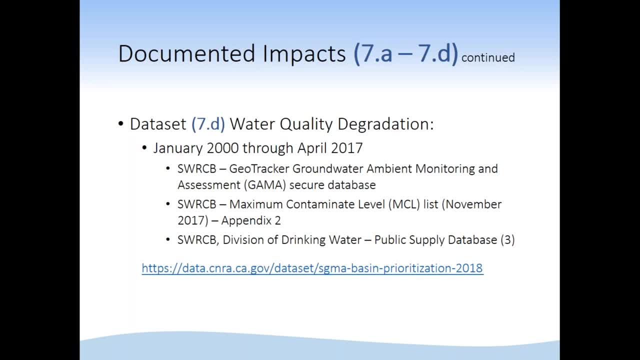 Water quality and degradation. This was the only one of the four. that wasn't the yes or no answer. Do you have some signs of yes or no? In this particular case, this was based off of data sets that we acquired through GeoTracker. 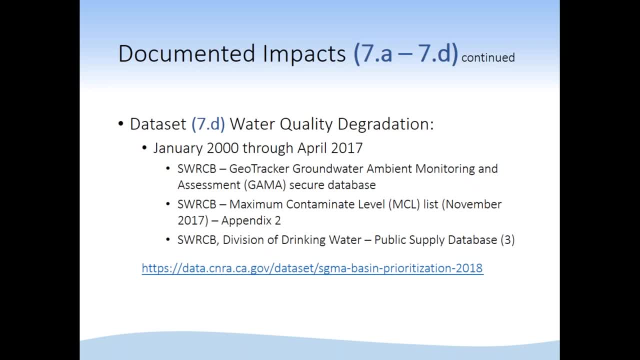 the Gamma system. We also used the contaminant level. We had two. We had one earlier and then we had to update it in November 2017 because our original data set also included chromium-6, but that has since been ruled in court to be not valid. 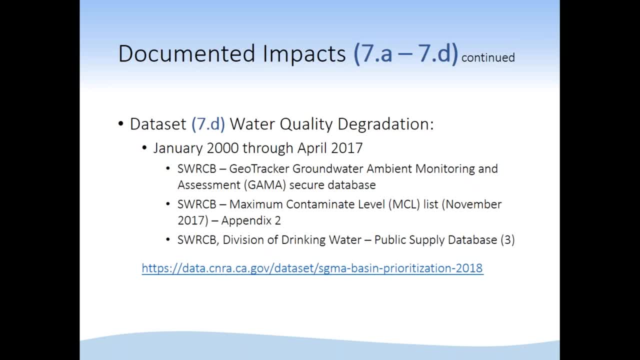 so we had to back that out. We had to use an updated version. It's also included in a document that we produced as Appendix 2, and it includes both primary and secondary MCL values. Then we also used the public supply well data set that we received which was used in Component. 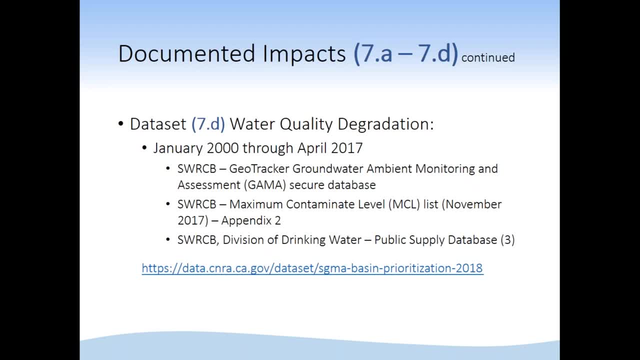 3. This too was broken into two categories. First part was basically to determine the magnitude or the MCL value. The first part was to determine the water quality. The second part was to determine the water quality. The third part was to determine the MCL exceedance number. so if MCL was 10 parts per million, 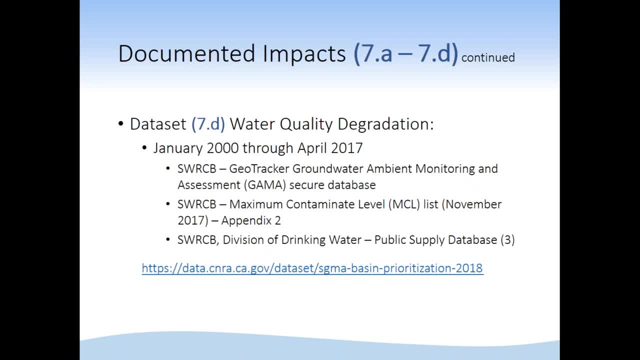 and you were at 100, that was a 10x exceedance. Basically all the different components that were detected in that basin that exceeded in that basin. we calculated that magnitude factor and then averaged them to come up with an average MCL exceedance and then we applied it to a breakpoint system. 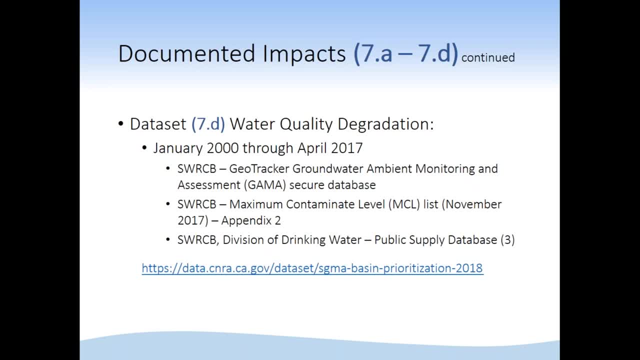 The second part of it relates to, more spatially, How many public supply wells within the basins, how many individual- excuse me, individual- wells throughout the basin. public supply wells have been impacted with some level of exceedances of different contaminants. 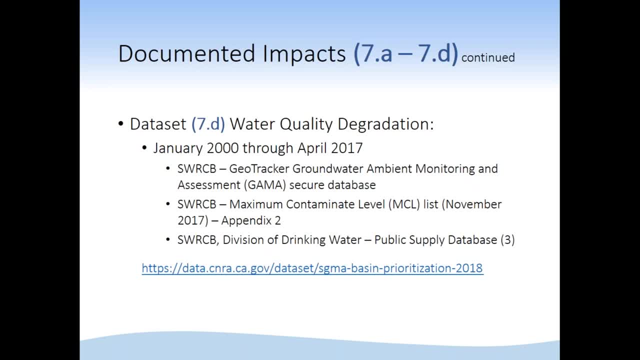 So we had more of a spatial. is it 50% of the wells? 10% of the wells? The one drawback that I didn't cover when I discussed the public supply well database is that we only looked at active wells within the basin. 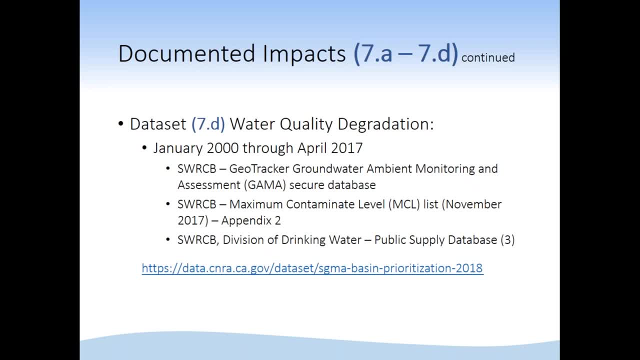 At a given snapshot in time back in 2017 or 16, whatever we called it. Wells come in and out of that data set as active or inactive, depending on its status. It could be taken offline due to water quality. it could be taken offline for maintenance. 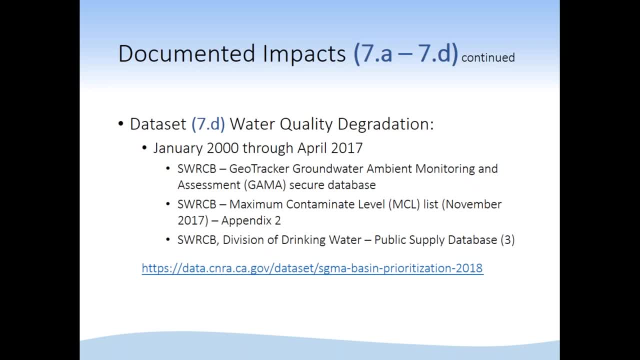 or it could be taken offline for demand or just simply destroyed. So there's a lot of factors that bring it in and out. so that's why we use that data set and we said only active wells. So sometimes there's a little disparity between how many wells have MCL exceedances versus 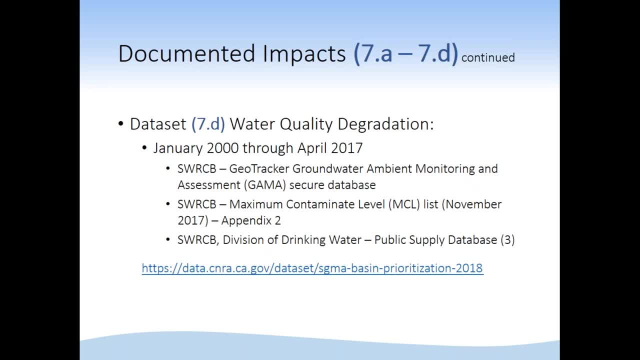 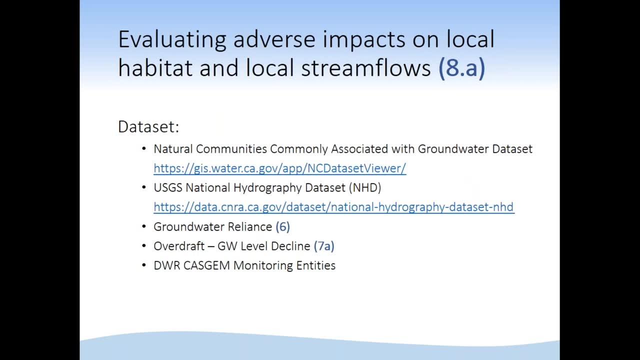 how many active wells. So we had to handle that as well in this process, which is also documented in the manual Evaluating impacts on local habitat and stream flow. Trevor talked about this a little earlier. This is new for basin prioritization. 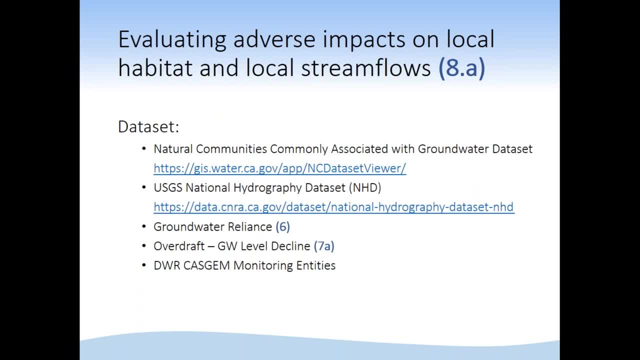 It was not part of the 2014.. This is a we had to create. We had to work. We had to work with different agencies and organizations to try to build a data set that would map where these natural communities are. These communities are associated with groundwater. 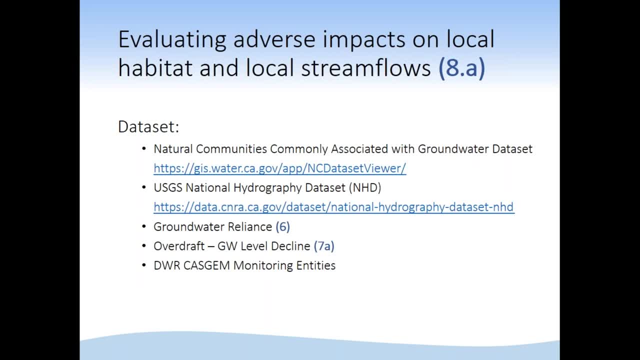 So we created this data set. This was work done by CDFW, the Nature Conservancy DWR, of course, and also there was some off and on conversations with US Fish and Wildlife and NOAA Fisheries concerning what would be in and what would be out and things like that. 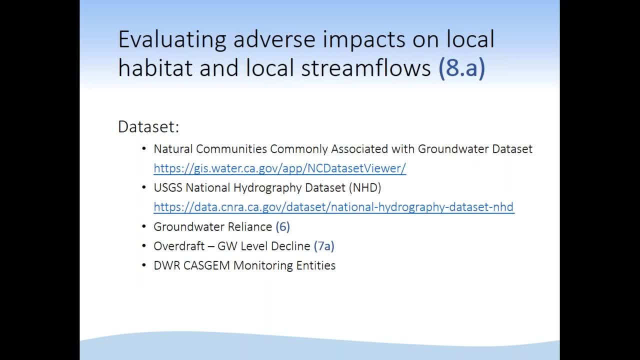 That data set has been online for roughly a month or so. It's also on the DWR website. You can access all the different layers that went into constructing that data set, as well as downloading and pulling information related to your basin. That took care of the habitat side of that equation, and then we used the National Hydrology. 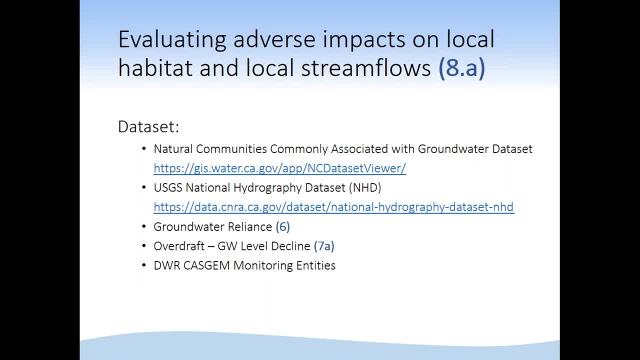 Data Set NHDA. That's the National Hydrology Data Set NHDA. That's the National Hydrology Data Set, NHDA. That data set is also available, as you can see on the website. We used that and only looked at the permanent and perennial streams and things that were. 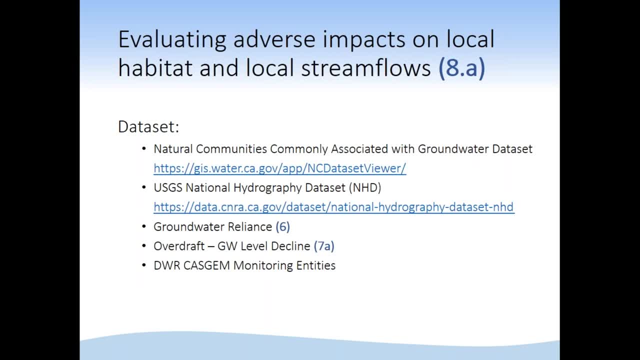 intermittent or things like that. We didn't necessarily use those. It was a little harder for us to justify using that. So pretty much anything that was permanent or perennial we flagged as being in that basin. This again is a yes or no kind of approach. 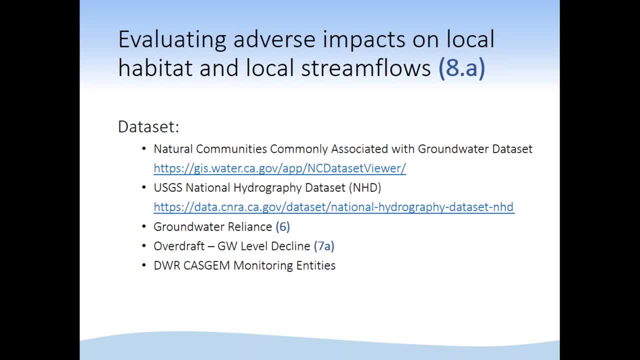 Both of these. Are there natural communities within the basin? Yes, The flag was set. Are there streams that are permanent and perennial in that basin or adjacent to that basin? And the answer is yes, Flag was set, And then we used both the groundwater, reliance information, which was pretty much the groundwater. 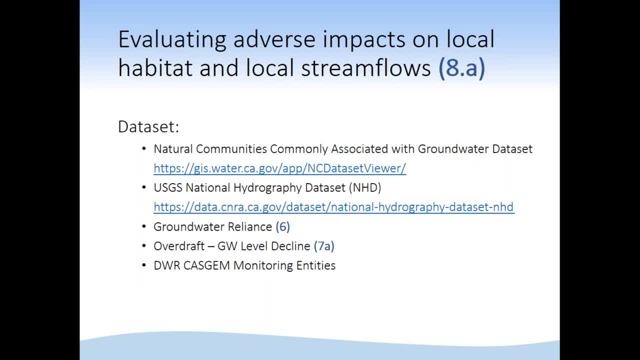 volume. that was normalized on the acreage of the basin, so it was groundwater acre-feet-per-acre value, As well as whether or not that there's groundwater level decline in the basin and then whether there are monitoring that is occurring. Obviously, in most cases, the last two go hand-in-hand. 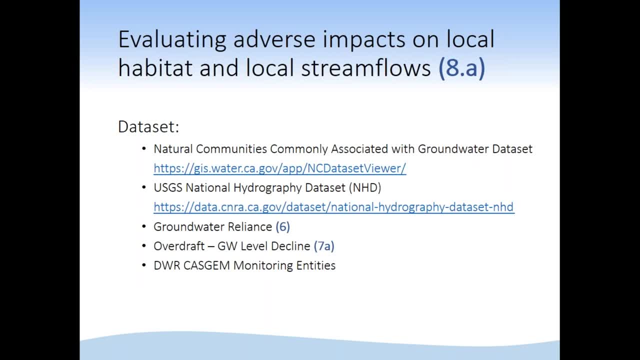 There's got to be monitoring to know. But there are places where groundwater level declines are going on, but they don't submit data to CASGEM. And the reason we had to do it this way was because there's roughly onlythere's, onlythere's. 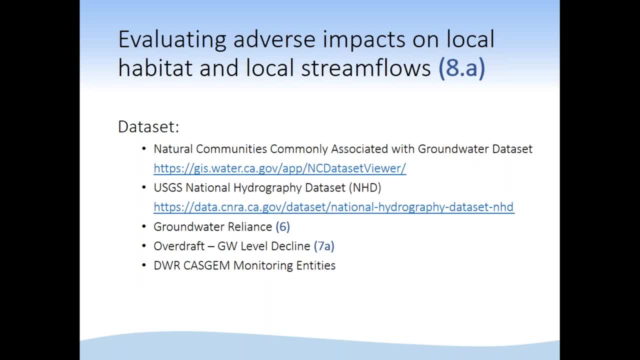 roughly. There's 282 basins out there that we know of that are monitoring groundwater levels and there's another 235 that are not monitoring. So we had to be able to process both of those kinds of scenarios to be able to answer the. 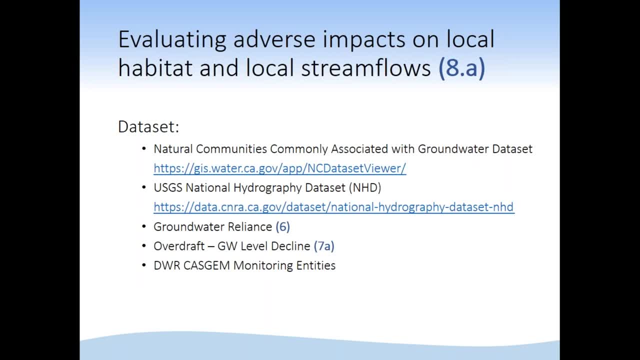 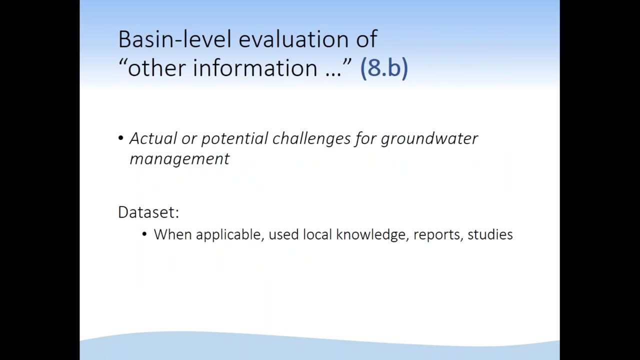 question: could natural communities, slash habitat and streamflow be impacted by groundwater activities? So that was the approach that we took for resolving this particular question. Okay, Then there's the other information, and this is basin level. after doing basin level evaluation, 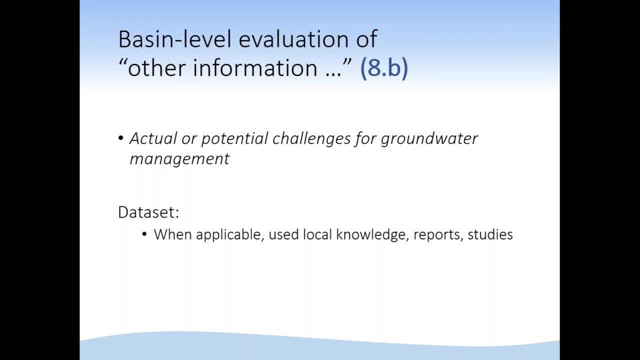 And this is actual potential challenges for groundwater management and challenges for sustainability, things like that. So the data set on this is what was applicable. It was local knowledge reports, regional studies and studies. There's a lot of research that goes on in a lot of places, so we relied a lot on that. 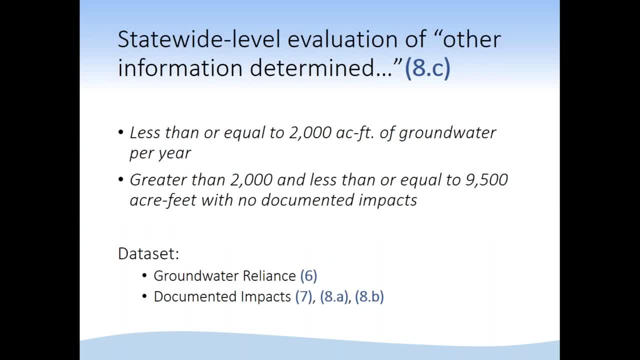 to be able to answer some of these questions. Okay, Now we're into 8C, 8D and 8E, which are analysis that we performed in order to determine the likelihood whether the basin was going to be a very low priority or a high priority. 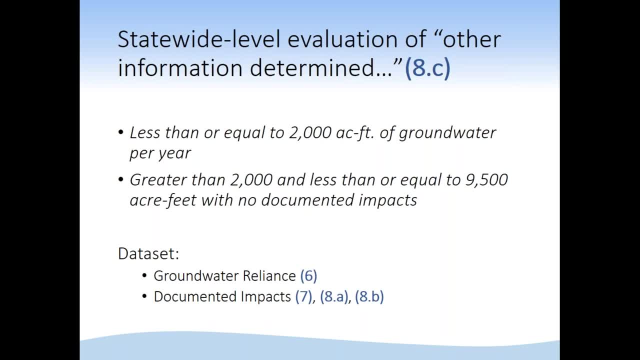 or, in a case, a sigma priority. Okay, So the first analysis we did involved with groundwater level or groundwater volume, If the basin was less than 2,000 acre-feet of groundwater per year, and the second one was greater than 2,000, but less than or equal to 9,500 and had no documented impacts. 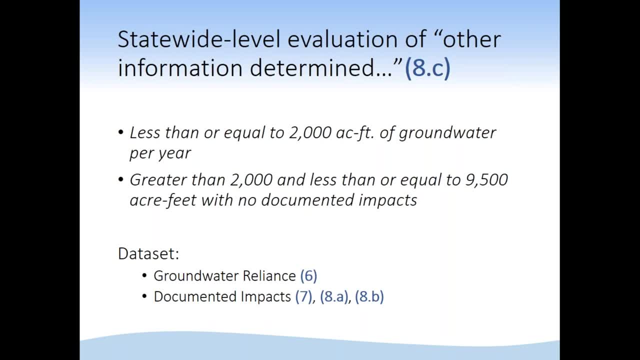 In order to answer those two questions, of course we had to use groundwater reliance. It was the groundwater volumes associated with component 6A and it was the document and impacts identified in 7, so any one of those four- A, B, C or D- but only if they. 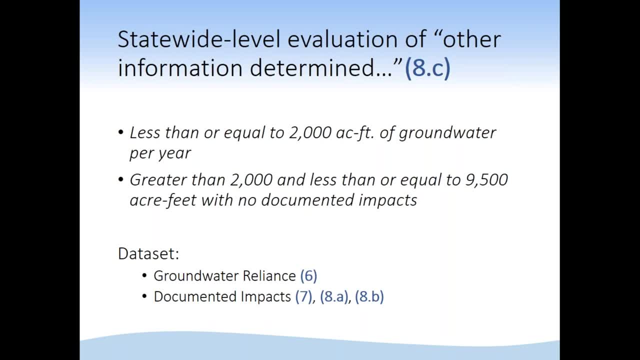 had documented impacts points. So each one of those four- A, B, C and D- calculate their own individual points, which are then added up and run through a break point and depending on where those points total up and where they show up in that break point is how many documented impact points? 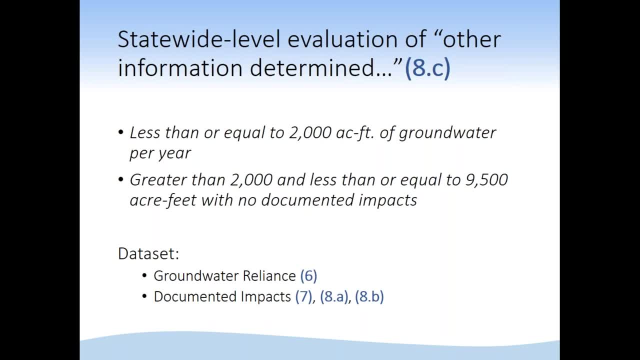 they give for number 7.. Okay, So there's the possibility that it takes at least three to get one documented impact point. I have to say that because you can have one point, say for water quality, and not get any documented impact points. 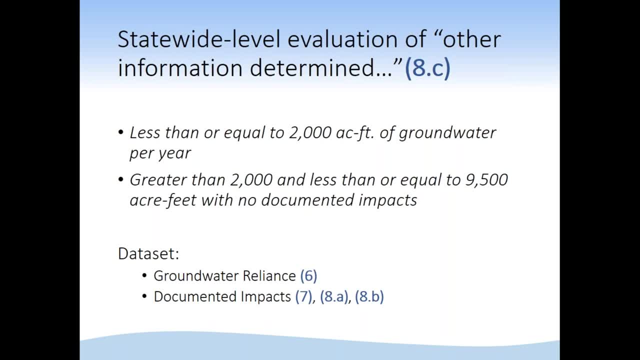 The second is if there was documented impacts associated with the habitat and stream flow. that was component 8.A, and the second one was: is there documented impacts that potentially could be impacted? Okay, Okay, So that was component 8.A. 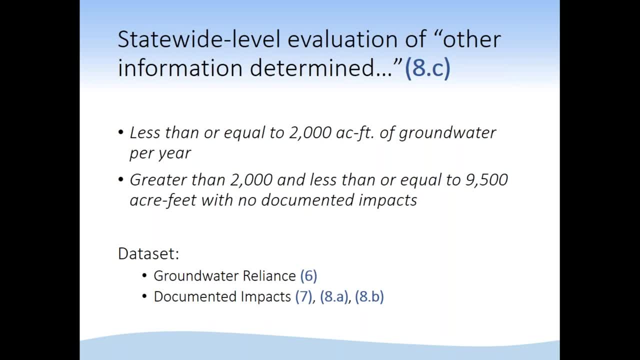 So there was a very clear data set that we had to look at to see if there was a problem with the way that this was impacting the groundwater management or sustainability of the basin. So those are the three that we looked at, those two data sets, three, four different. 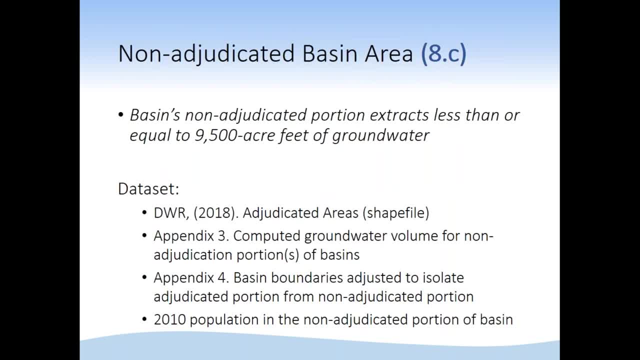 sections that we used to answer this question And it affected quite a few basins one way or the other. Then the next test, that analysis we did, that Trevor mentioned earlier, was had to do with the non-adjudicated basin area in relation to the adjudication throughout the state, the statement that 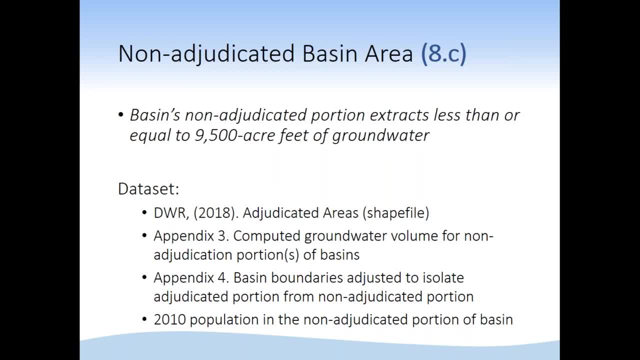 we the analysis that we did to answer this question: basins, non adjudicated portion strikes less than or equal to 9,500 acre-feet of ground wire. now, to do that, we have used several different data sets. we had to build a data set which. 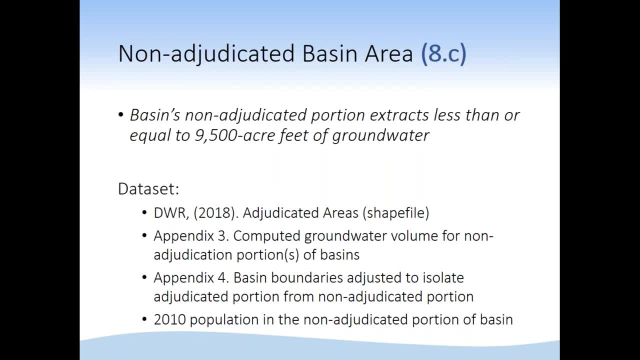 basically takes the adjudicated shapefile that's online on DWR and our basin boundaries and basically create two shapefiles, two basin boundaries, one that shows this basin is adjudicated in this portion and non adjudicated in the second portion. and then we had to compute the groundwater volume for the 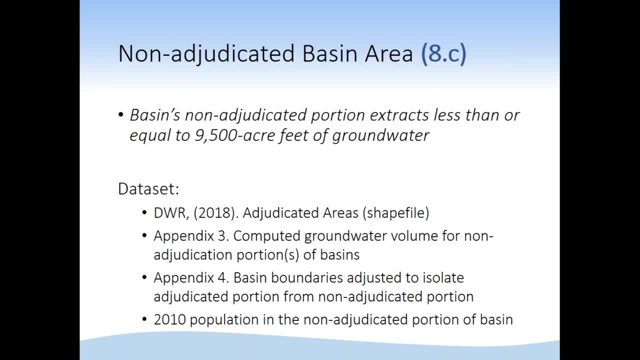 non adjudicated portion of that basin and we, excuse me, we just basically went back to basically 6a and redid that process for the non adjudicated portion and I and that's all that. information associated with the volumes is provided in appendix three and the details associated with the basin boundaries. 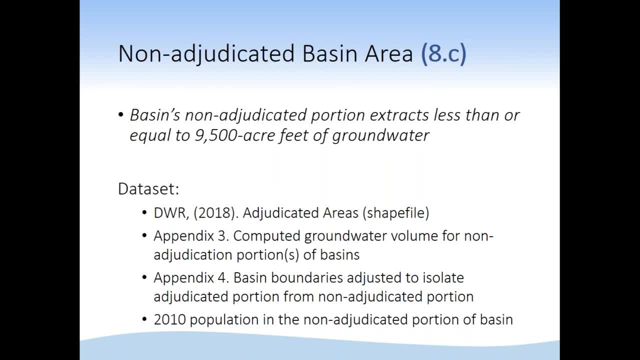 being adjusted for. the non adjudication portion is also provided in appendix four, and then we just simply use the to calculate earlier the main population. right here, and for those of you who are familiar with the turbine, we needed a population, so we use the 2010 population for the non. 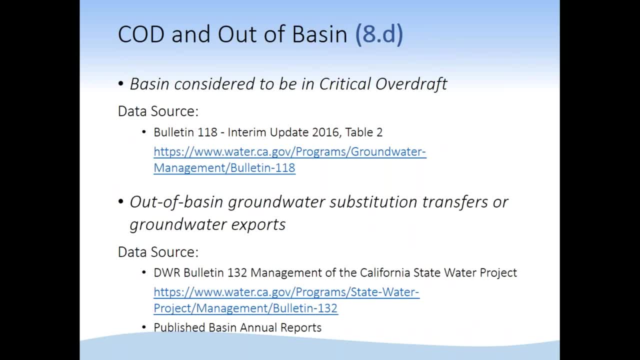 adjudicated portion of the basin critically at critically overdrafted basins and out of basin groundwater substitution transfers and groundwater exports. again, these are new for 2018 Bulletin 118, Interim, Update 2016,. we identified 21 basins to be subject or in critical overdraft. 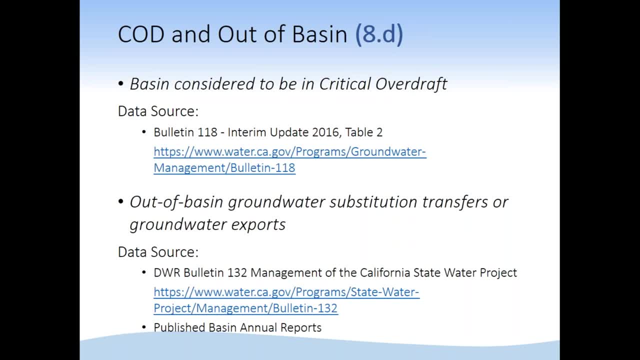 Those basins were then flagged in Basin Prioritization for critically overdrafted and then for the out-of-basin groundwater substitution transfers or groundwater exports. we relied on DWR Bulletin 132, which is the management of California State Water Project, where they track the 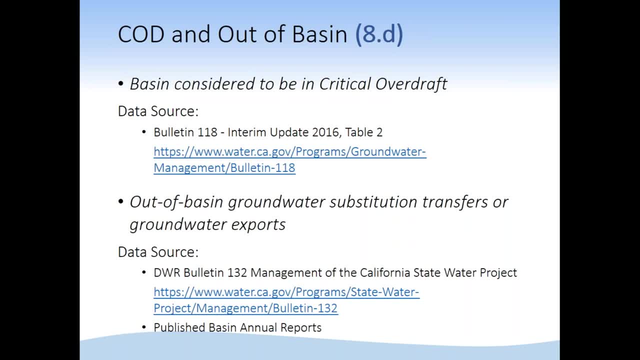 arranged or coordinated substitution, transfers, conveyance, things of that nature, as well as published annual reports for basins to get a sense of what was going on with respect to that, Anyway. so that was also flagged for special consideration within Basin Prioritization. 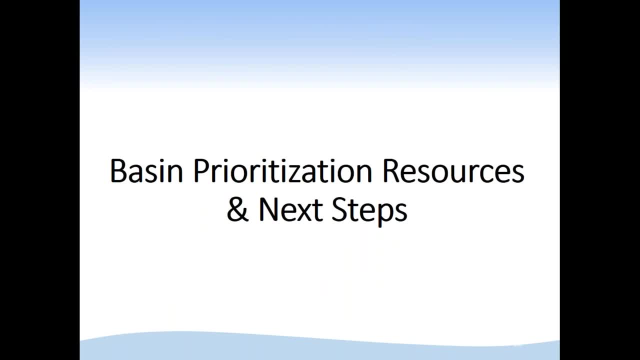 I reached the end. Steven will now cover the resources and next steps: Steven Springhorn. All right, thank you, Roy. Good afternoon everyone. So my name is Steven Springhorn and, as Roy mentioned, I'll be covering the Basin Prioritization. 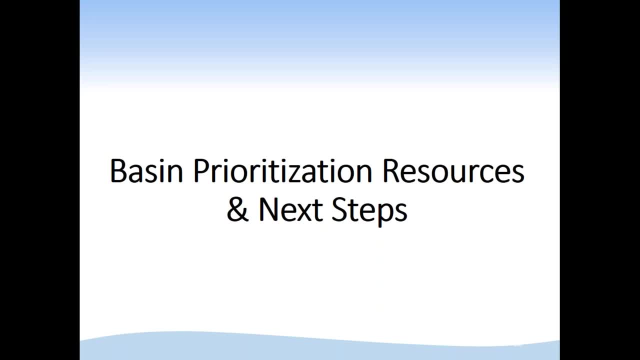 resources that our team has put together to make the 2018 Basin Prioritization results available, As well as some related data sets and information, and also talk about the next steps, which includes the timeline from here on out for the rest of the Basin Prioritization process. 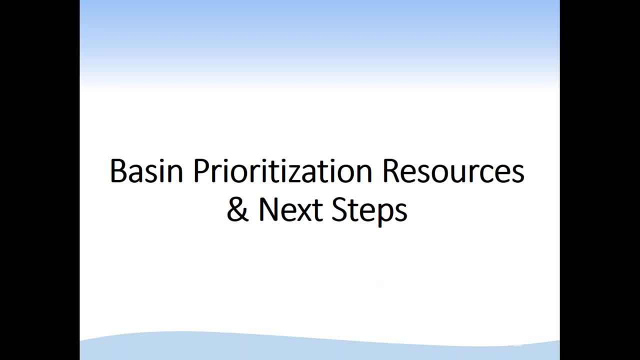 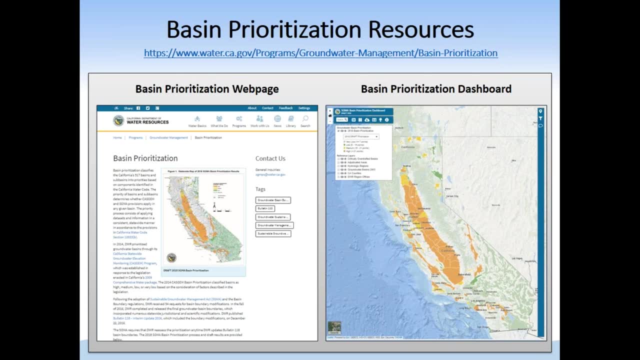 and some information on how to provide public comments related to this Basin Prioritization. So I'll start with the Basin Prioritization resources, and there's two key resources that are available. They're available at this website. That's on the top of the slide here. 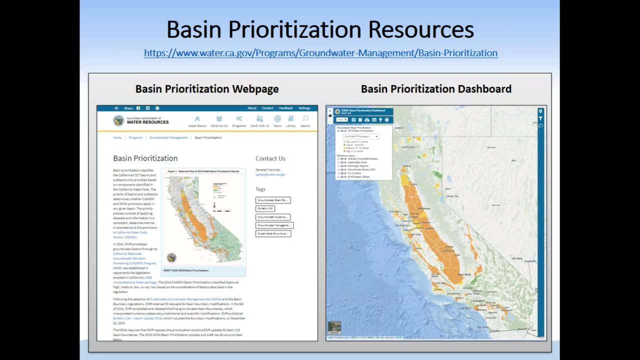 The first is the Basin Prioritization webpage. This is the hub for all things Basin Prioritization and where you can access the variety of other related data sets that are here On this website. Basin Prioritization website. there's also a Basin Prioritization dashboard. 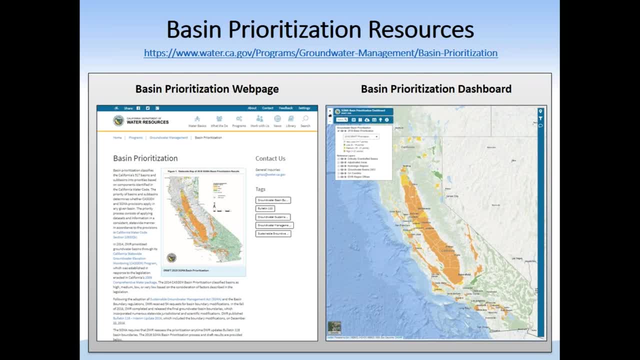 that allows you to look at the draft 2018 results across the state on an interactive map and look at the components that Roy mentioned for each individual basin. So I'll do a quick demo for each one of these resources so you get a better feel of what. 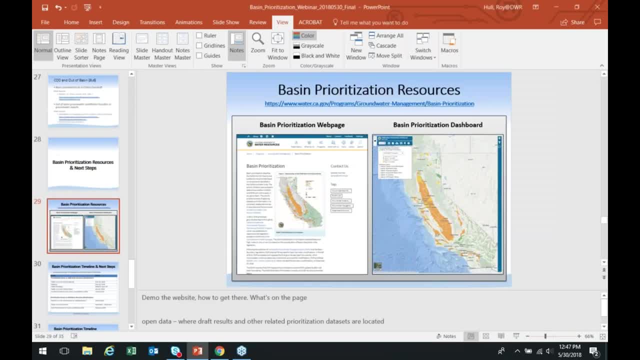 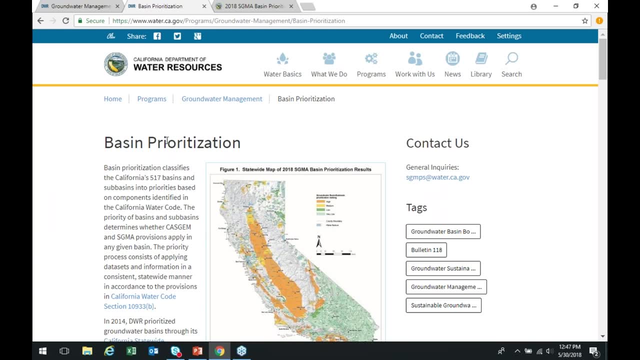 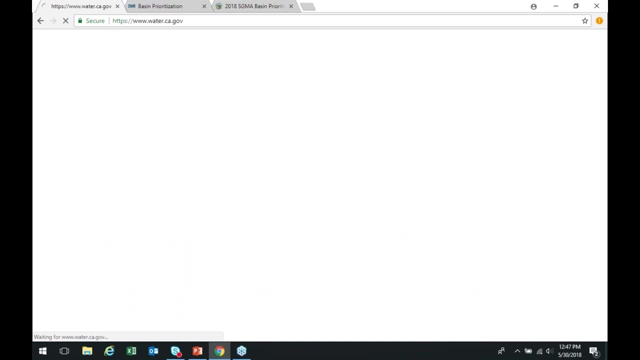 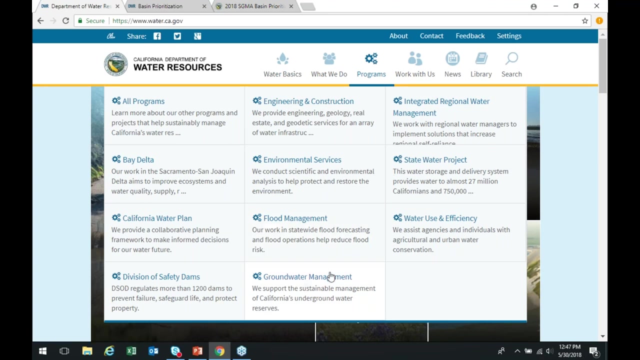 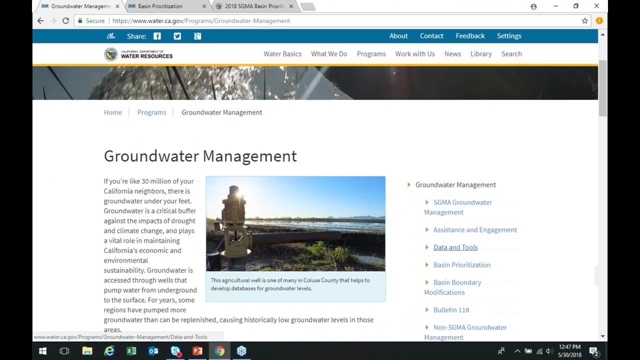 is available on these sites. So this is a view of the Basin Prioritization webpage. I want to start with just how to access it. You can access this information on this webpage starting from the Department of Water Resources homepage. You go to Programs, Groundwater Management and on the main Groundwater Management webpage. 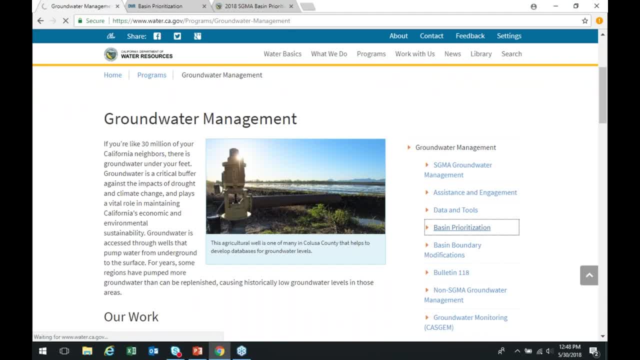 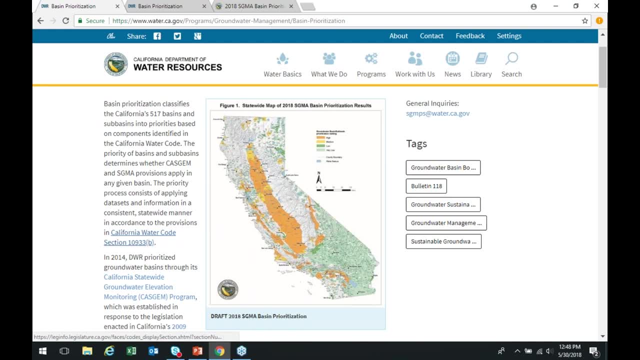 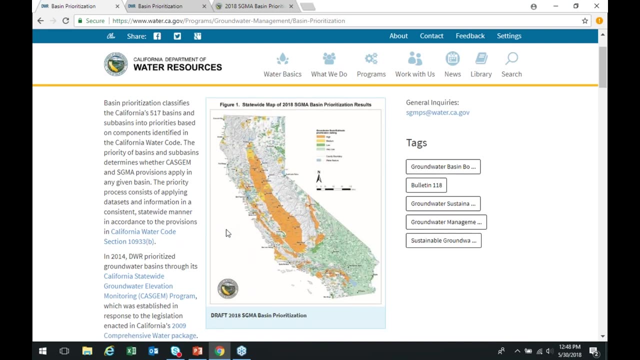 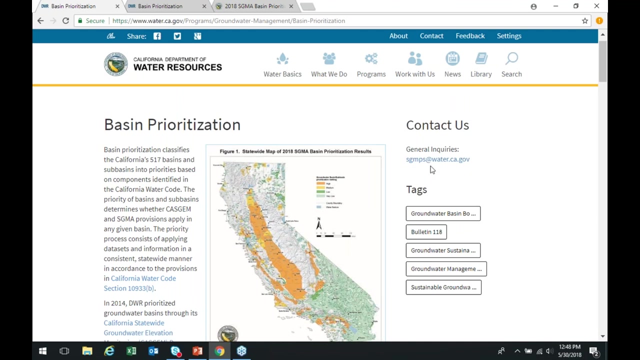 there is a link for Basin Prioritization. So on the Basin Prioritization website there's some introductory information that Trevor covered. There's a summary of this process and past prioritization processes, a map of the draft results, as well as, on the top right here, a link to a SIGMA, a dedicated SIGMA email. 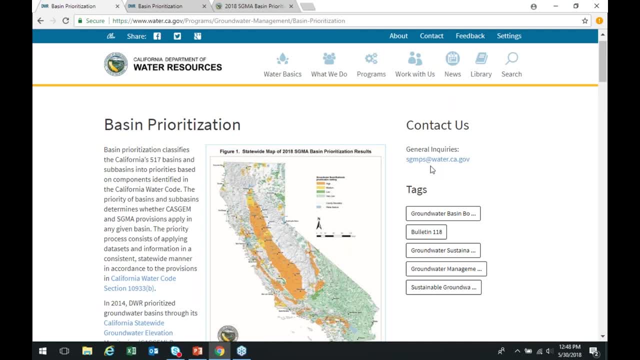 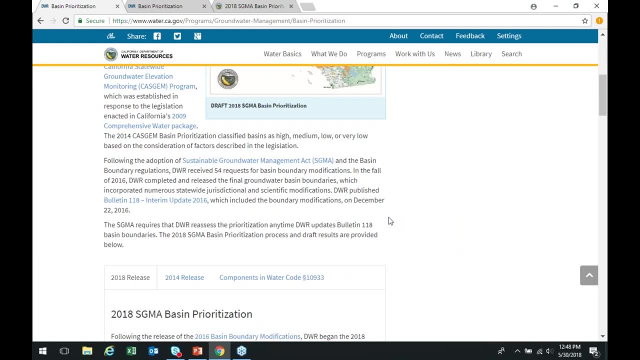 that you can send comments or send questions for clarification, and we'll touch on this in subsequent slides. Also on this site is additional information on the Basin Prioritization website. There's a link to the Basin Prioritization website. There's a link to the Basin Prioritization website. 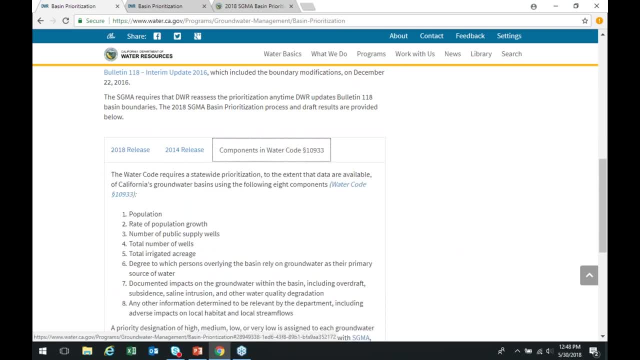 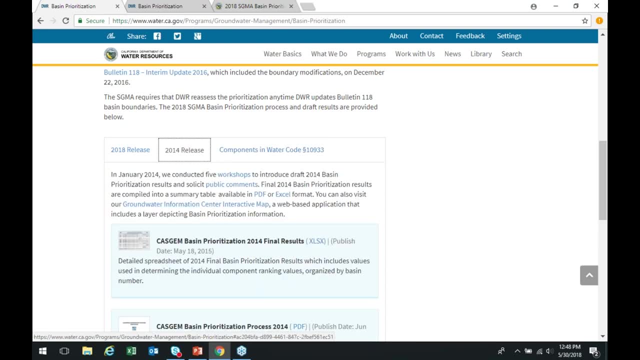 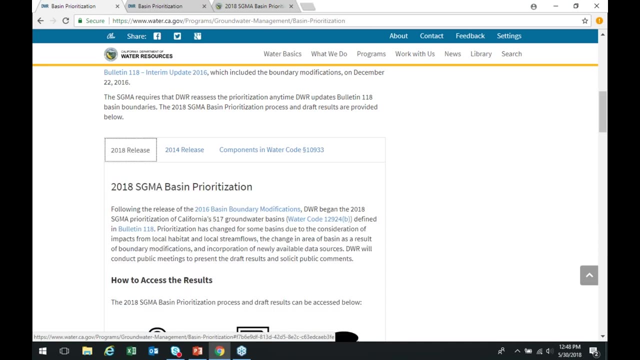 There's also some background information on the water code requirements that we are following for Basin Prioritization that Trevor touched on, Some historical information on the 2014 Basin Prioritization website and then the 2018 release of Basin Prioritization, which includes three main areas or components. 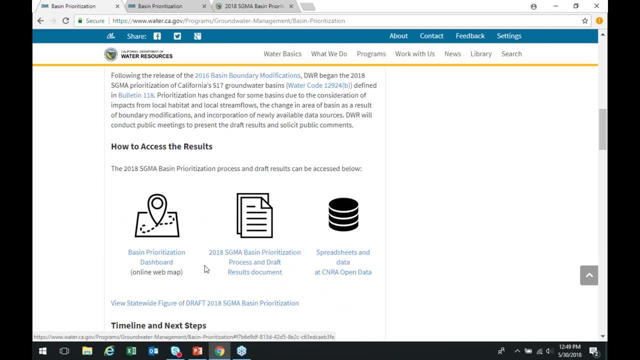 The first is the dashboard, which I'll demo in a second. The second is the Basin Prioritization product. The second is the Basin Prioritization tool. We're using the Basin Prioritization tool. We're using the Basin Prioritization tool. 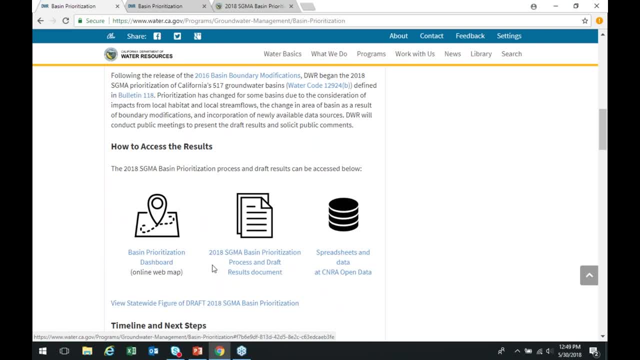 And then we use the Basin Prioritization tool to help people understand what they're doing. So I want to start right away. process document that Roy went over. This is a draft document and it has the process or an explanation of the process and results and other related information in this document. The third: 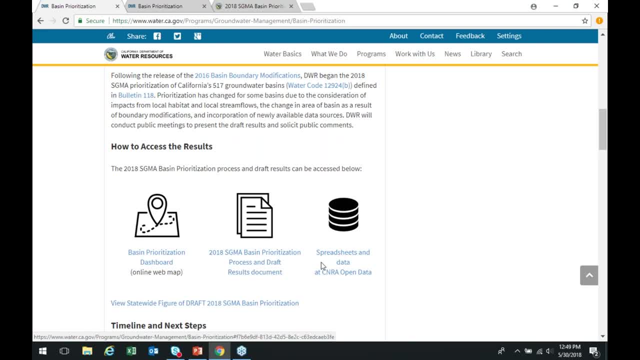 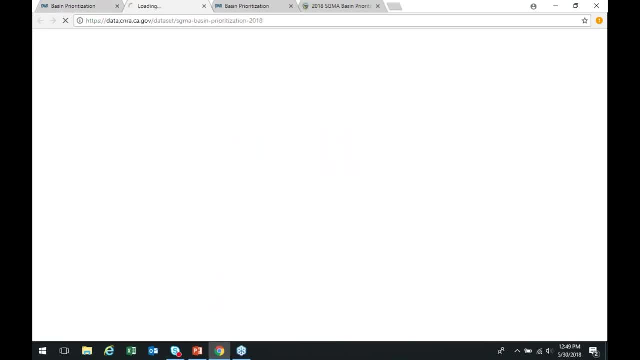 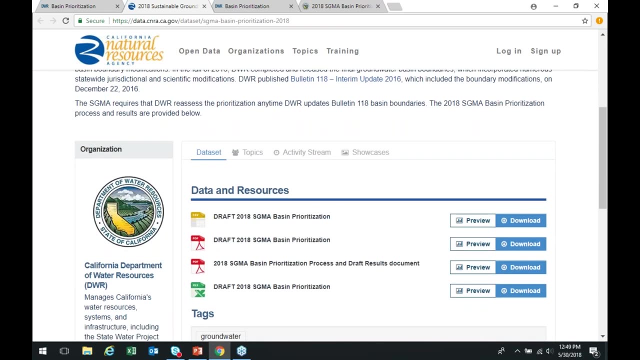 component. there are the spreadsheets and related data sets that are posted on our California Natural Resources Association open data platform. I'll quickly open this so you can see. there's some explanation on what this information is, and these data sets are available in a variety of formats. 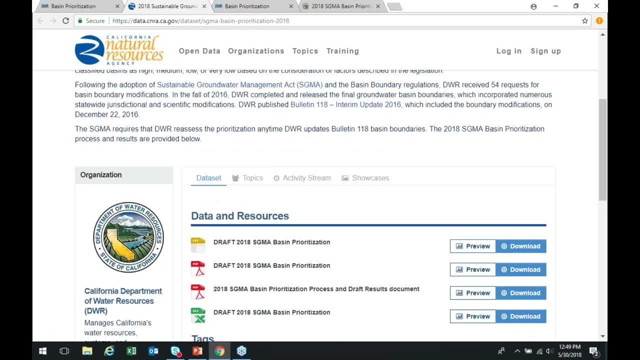 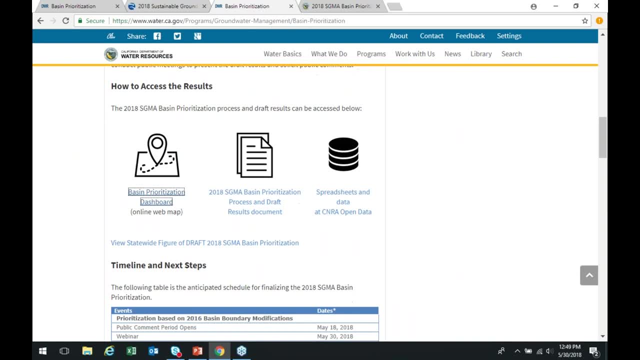 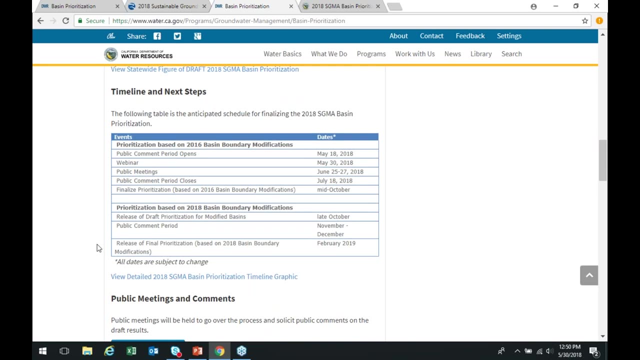 for you to access and review as needed. The next component on the website is the timeline and next steps. I'll go into a little bit more detail on this, but this information is here on the web page. Just stepping back quickly, there is a 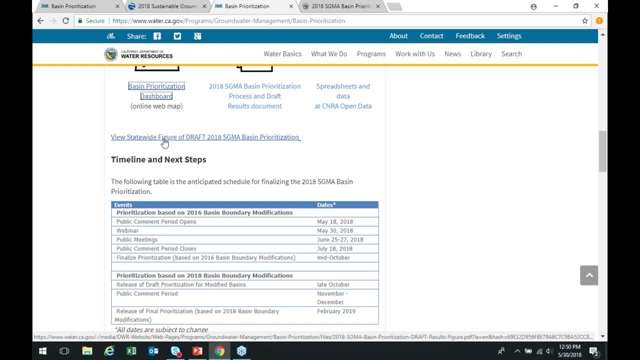 link in the description to the website where you can find all of the information on the website. There is a link in the description to the website where you can find all of the information on the website. There is a link to a figure that Trevor showed earlier of the draft results from. 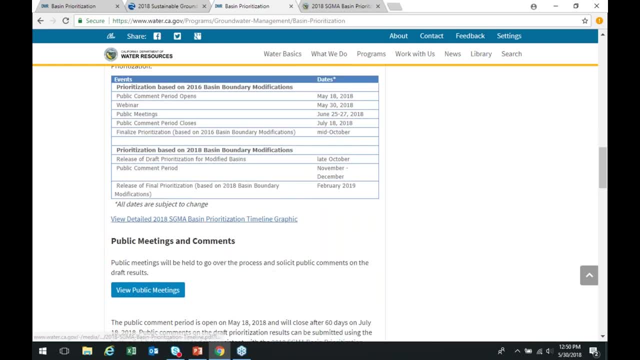 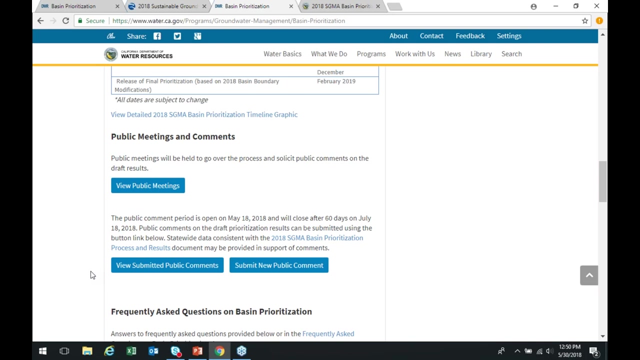 2018.. There is also a timeline graphic that shows how this prioritization process is related to some other existing activities- SGMA related activities. We'll touch on more of that in a second. Also, this is where to provide or submit public comments related to basement prioritization, so information. 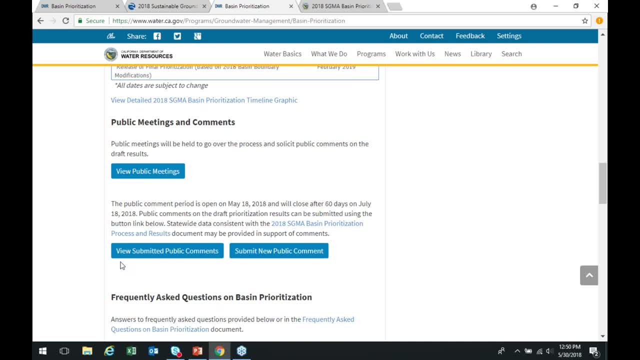 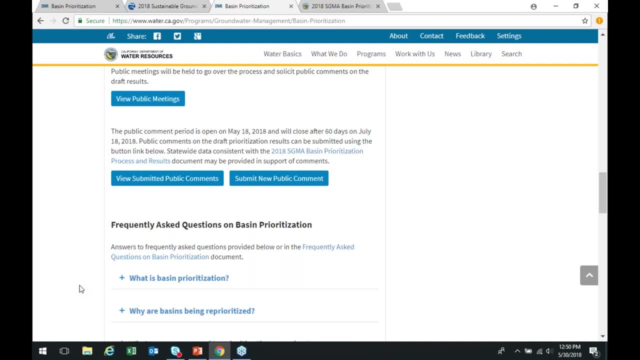 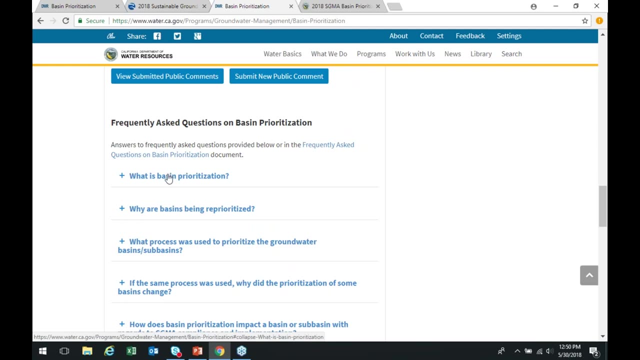 on the public meetings, you can view submitted public comments as well, as this is where you submit your public comments. we also have a number of frequently asked questions related to prioritization, and so you can click on a link to download all of them in a PDF form, or you can click on an individual. 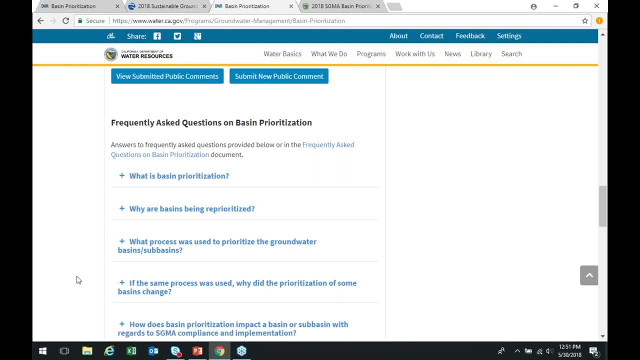 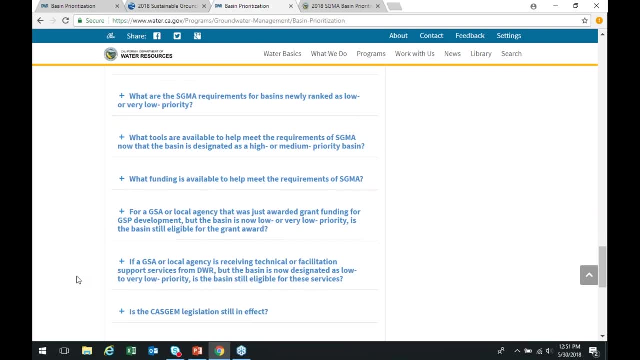 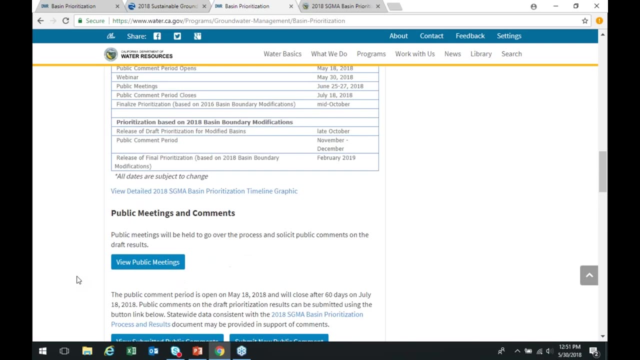 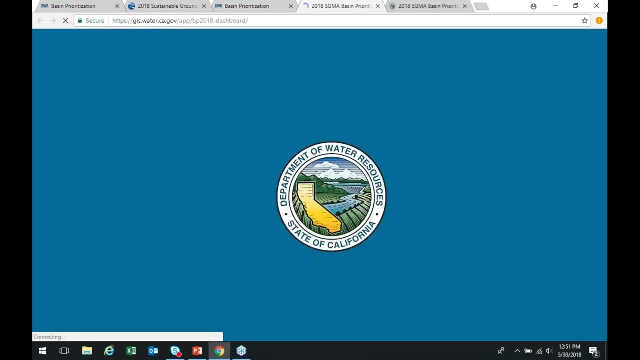 question that you're interested in and get more information here, and so there's a number of related questions on on this page, so now what I'll do is I'll quickly demo the basin prioritization dashboard that our team has developed. so again, that's the first link on the webpage and it opens up an interactive 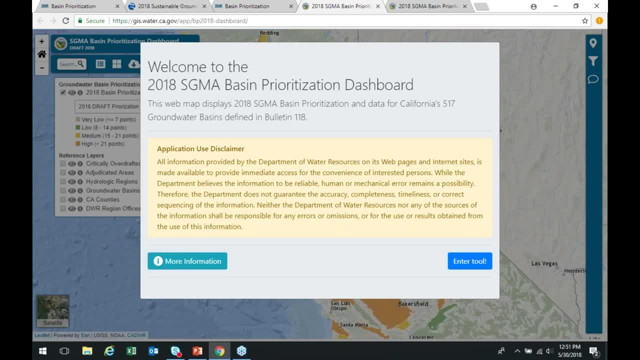 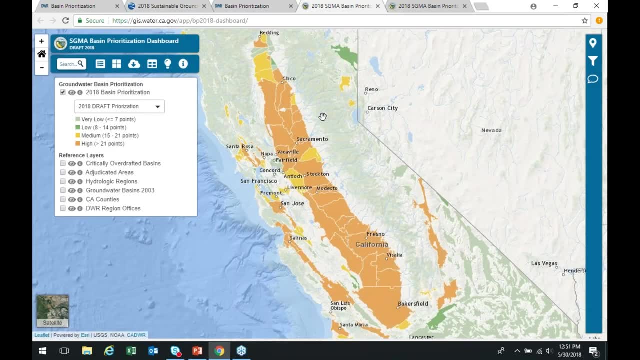 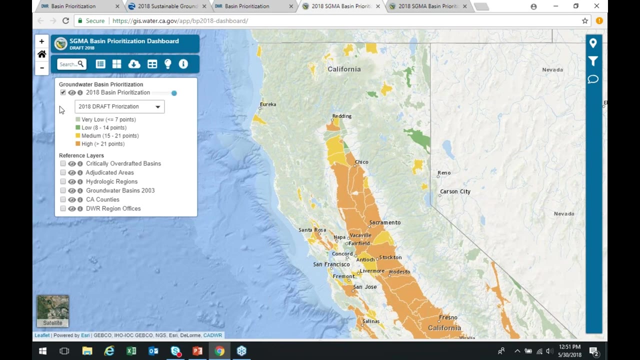 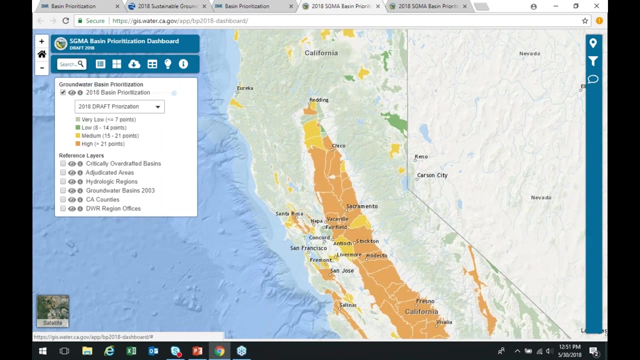 map viewer that has some introductory information here, and so what opens up is an interactive map where you can zoom in. you can search by a particular address or location here in the search bar. the other key features here are the map layers. there's the asin prioritization information for 2018 and 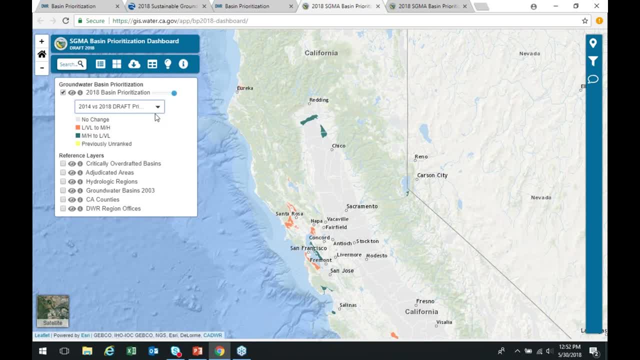 you can compare 2014- 2018 and she's a change. there's also a reference line. There's critically overdrafted basins that Roy mentioned. adjudicated areas, hydrologic regions, prior version of basin boundaries, counties and regional offices. 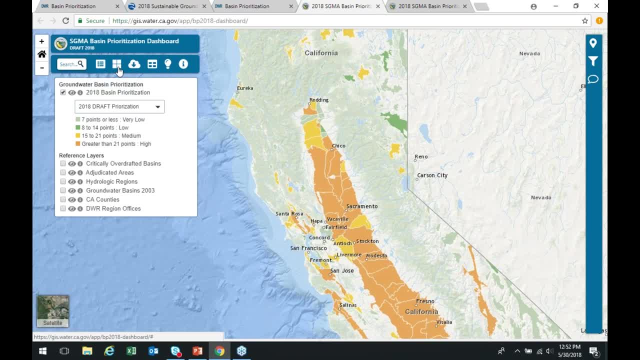 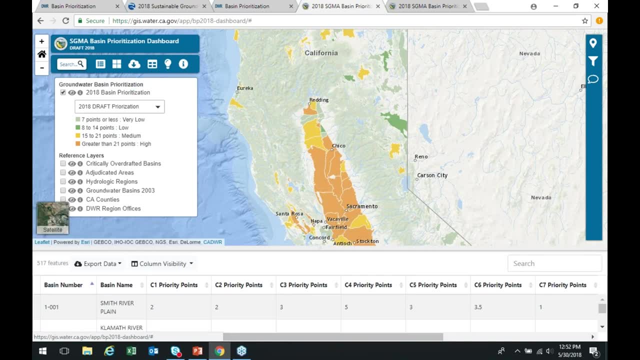 Another tool here is you can change the base map. if you're interested in looking at satellite imagery, You can download data and you can look at information in a tab format, and we'll go into these features in a second. There's also tutorials. 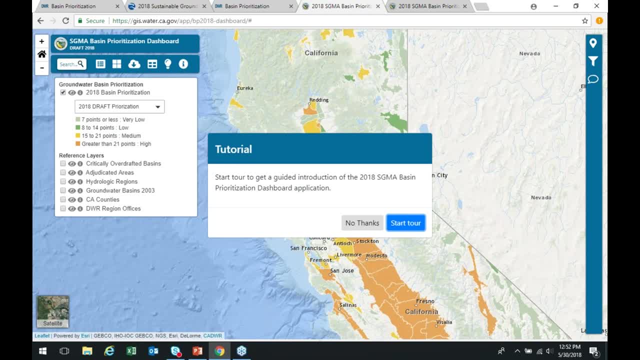 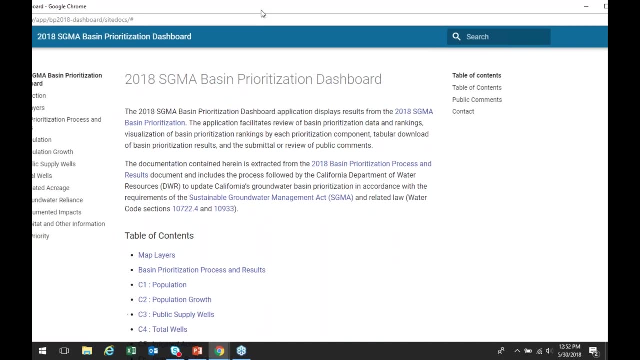 So if you're brand new to this site, you can step through a tutorial that gives you the general feel of the various features on this map, if that's needed, And then there is an information window that has the content that Roy described the process. 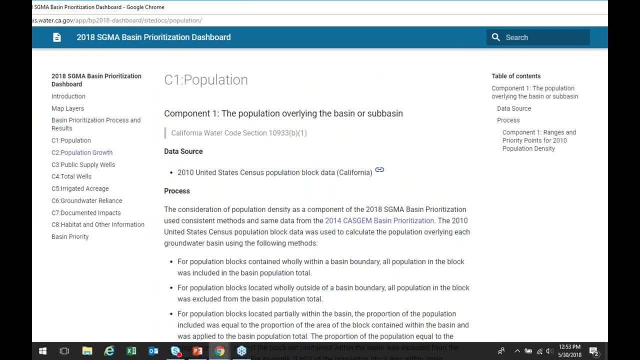 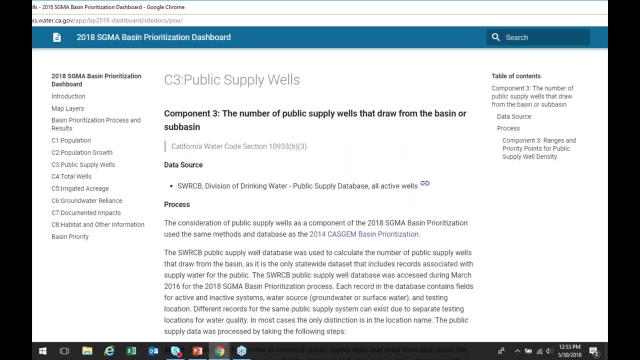 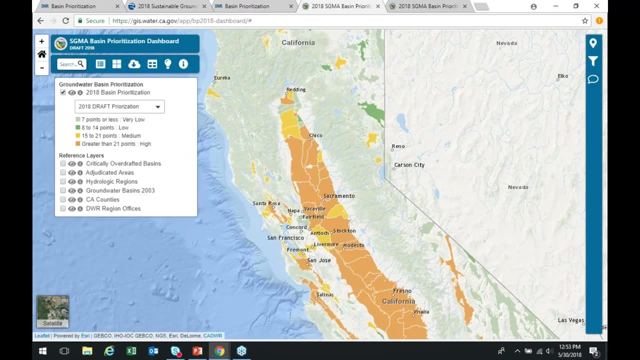 and data sets for each component. So it's essentially some background information and content, And then there's a little bit of context for each one of these components that were used for prioritization. So now let's look at some of the basin-specific information. 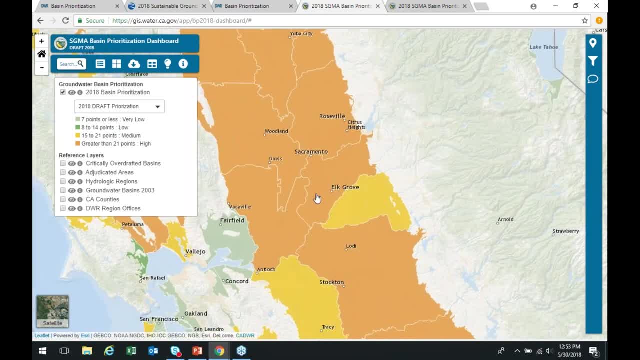 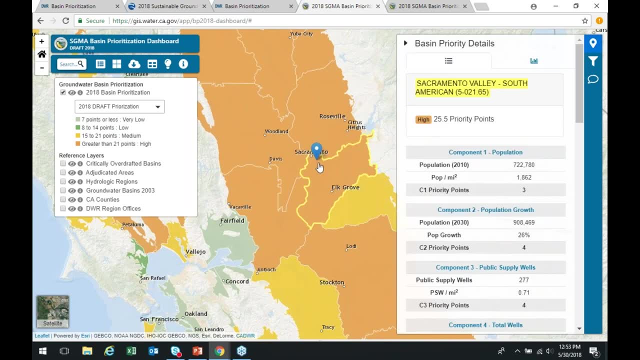 So we can zoom in here into the location where we are at here today in Sacramento, our home basin, the South American groundwater basin. When you click on a basin you're able to see the priority and the points And then information for each component that Roy described that we used for this particular. 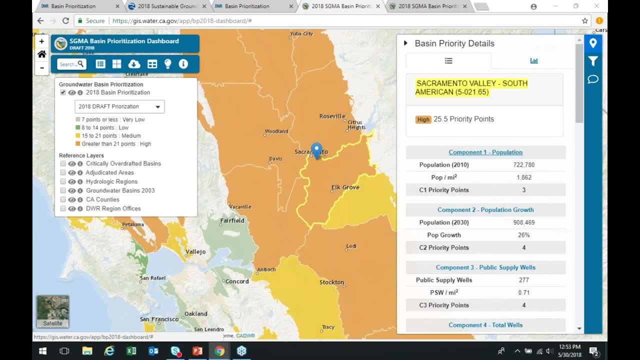 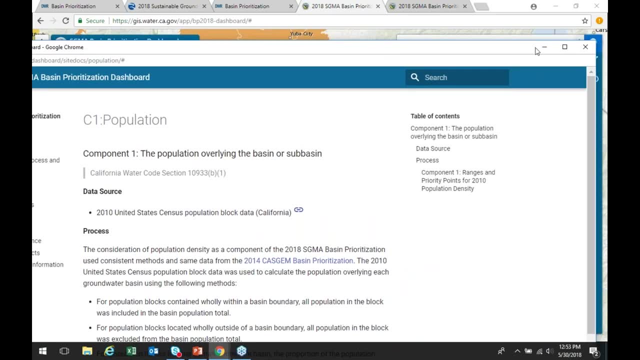 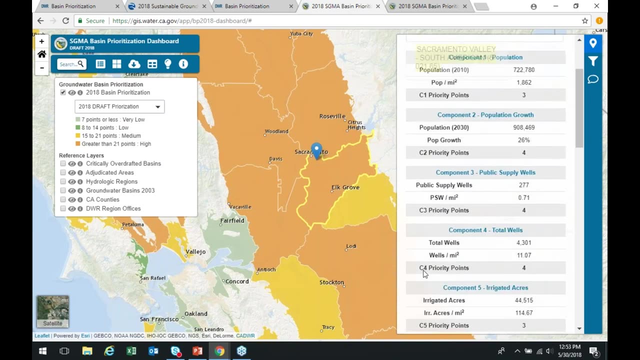 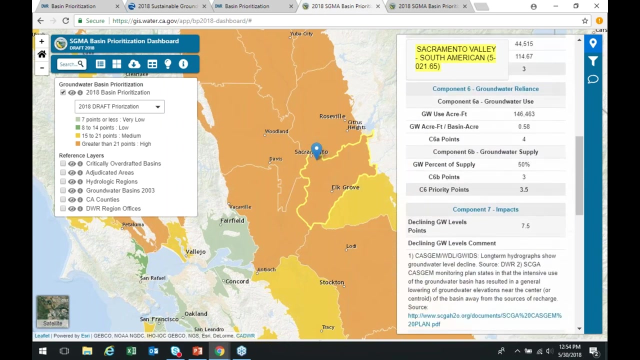 basin And if you're interested in what that component is, you can click on the component title there and it gives you the information related to that specific component. So components 1 through 8, all this information is here for every basin in the state. so all 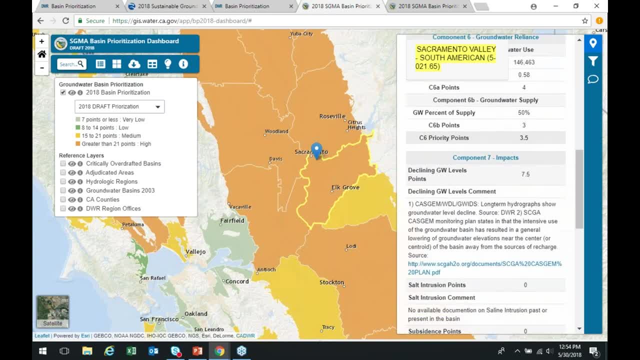 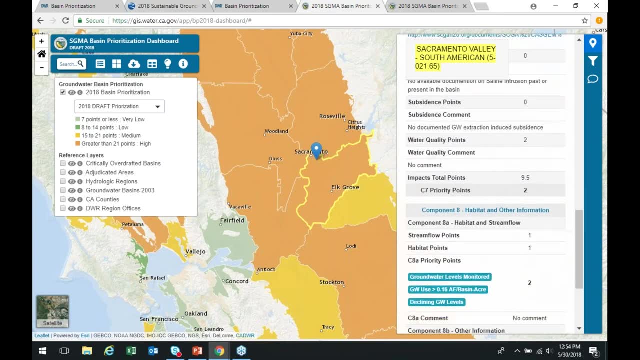 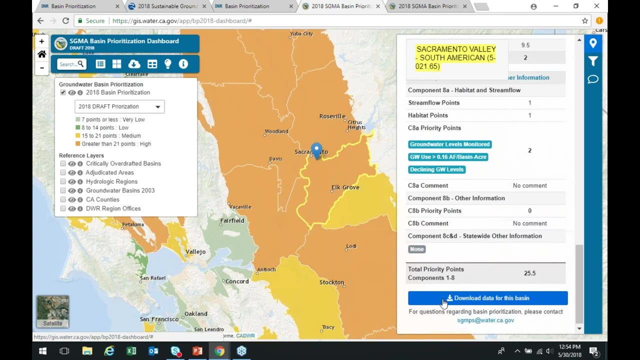 the 517.. It also provides links to additional information that Roy described And then you're able to download the data for your particular basin that's highlighted or provide questions or ask questions for clarification at this SGMA program email address. As you can see, if we select other basins, 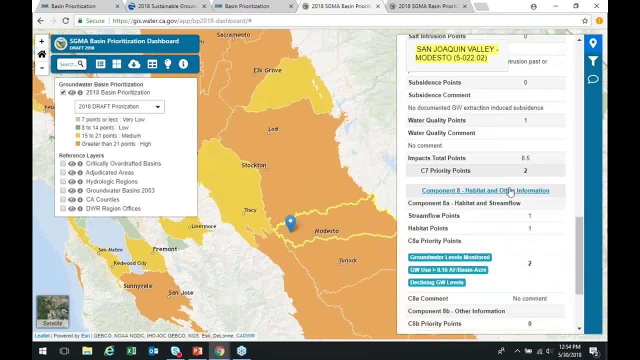 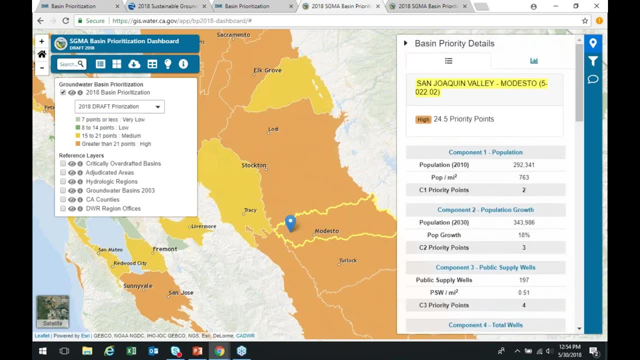 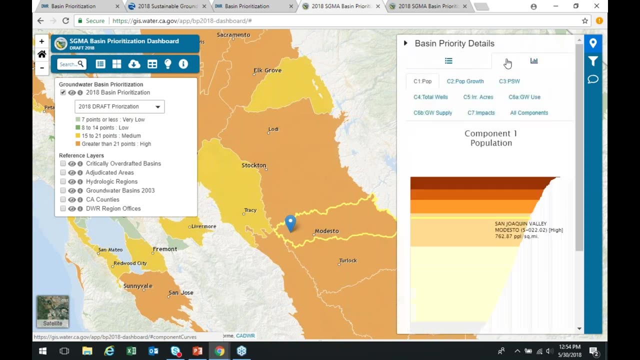 We're going to be able to see that. Okay, You can see the information changes and so it is specific to the individual basin. So one other thing that's on this panel for each individual basin is individual graphs of the components. each component: population, population growth. that Roy went over and 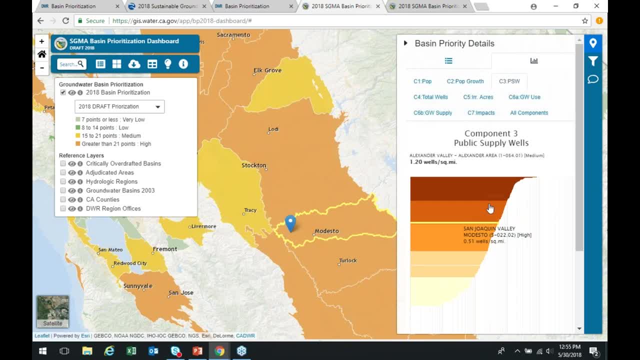 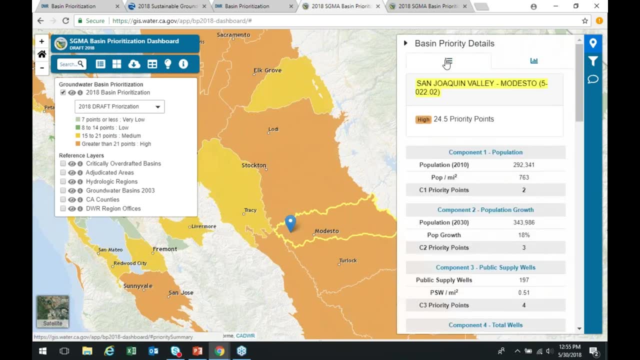 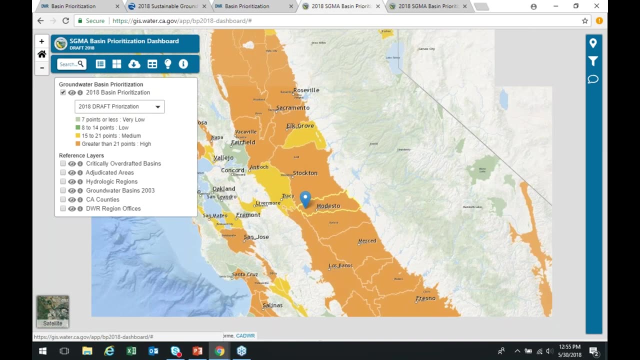 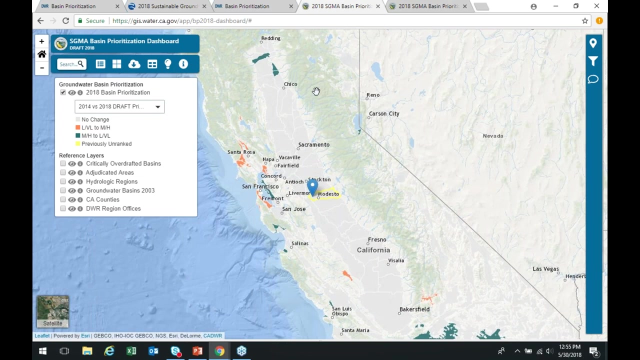 where that particular basin ranks within all the basins in the state. In addition, another way to look at the information, As I mentioned, if we zoom back out here to a statewide look, you can see the difference between the 2014 prioritization and this draft 2018 prioritization results and you can see. 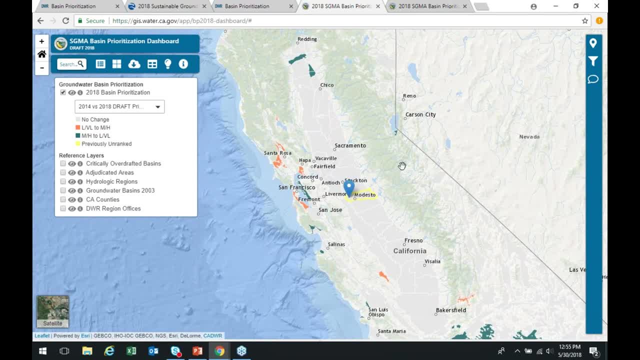 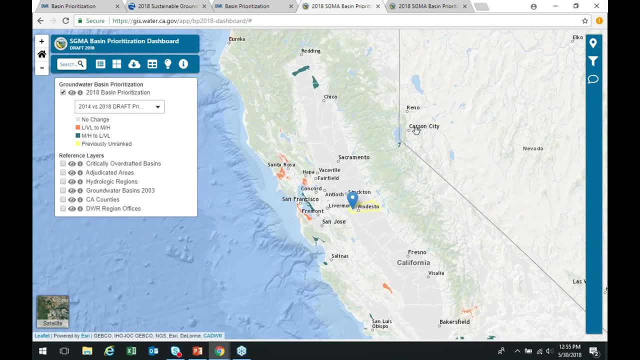 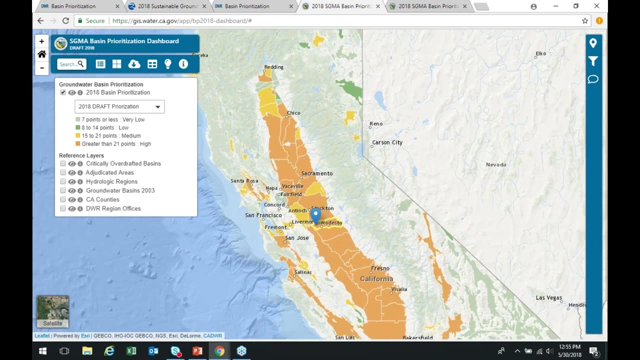 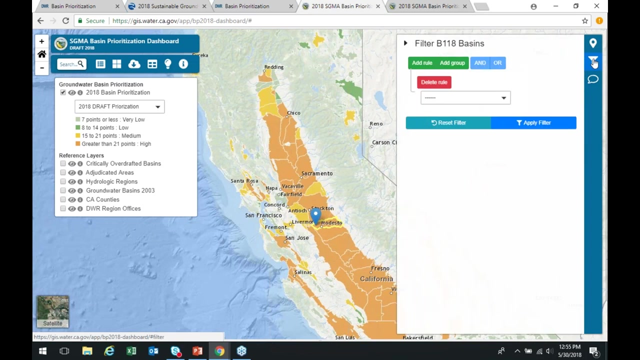 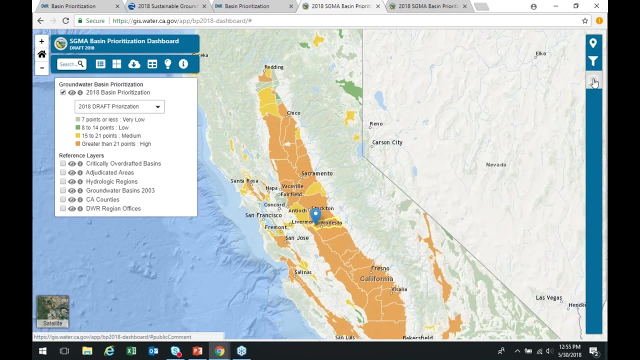 which basins went from low or very low to medium or high, or from medium or high to low. Some additional tools here that are also on this are again the basin-specific information. There's a filter function here where you can filter the results by particular queries or user-defined 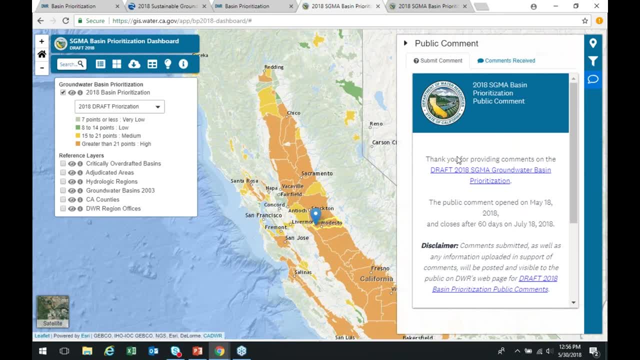 queries, And then you can also This links in our Our website or where you can comment, so you can actually submit comments from the tool. but this is utilizing that same public comment feature that's on our Basin Prioritization webpage. 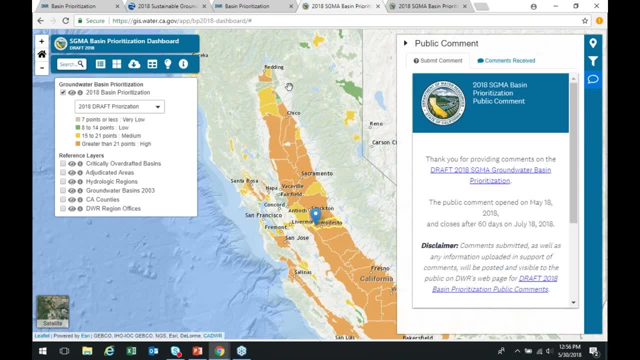 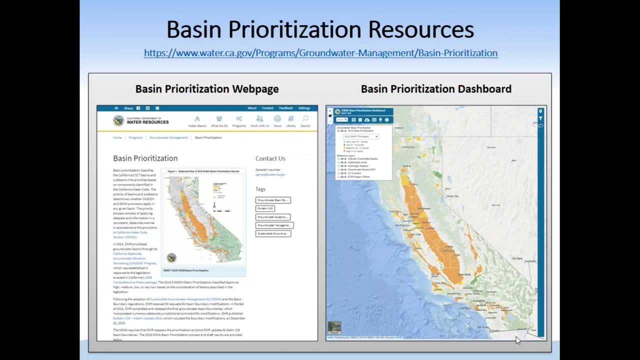 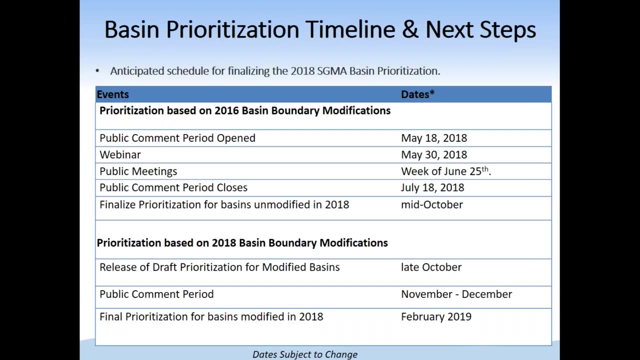 Okay, So now we'll go back to the presentation and move on to the Basin Prioritization Timeline and Next Steps. So this is the anticipated baseline. This is the updated schedule and sequence of steps that we plan to use to finalize the 2014 SGMA prioritization. 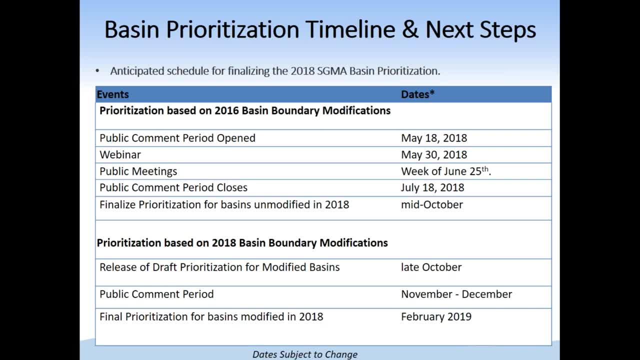 Again, these dates are subject to change, but this is what we're currently working under. So the public comment period opened May 18th. That's when the draft results were released. We're having a webinar today and we plan to have a series of public meetings the week. 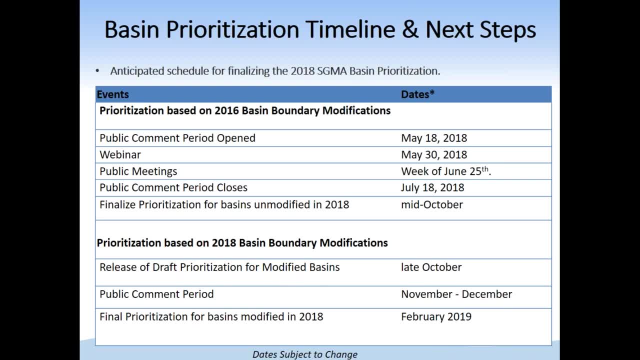 of June 25th And there'll be some additional information or details on the specific locations and dates for those venues in the very near future and those will be posted on our Basin Prioritization webpage. The public comment period closes. It's a 60-day public comment period. 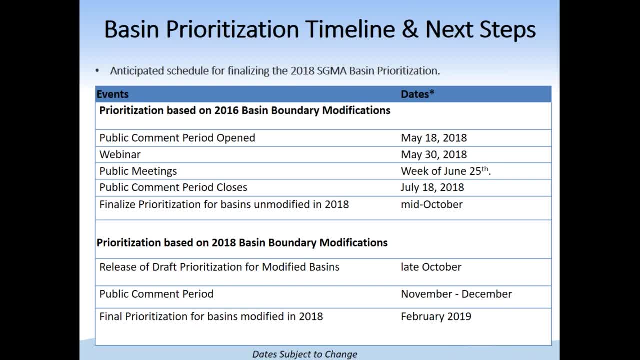 It closes on July 18th. The goal is to finalize the prioritization for basins that are unmodified as part of the 2018 Basin Boundary Modification, And we'll touch on that In a second In the mid-October timeframe. 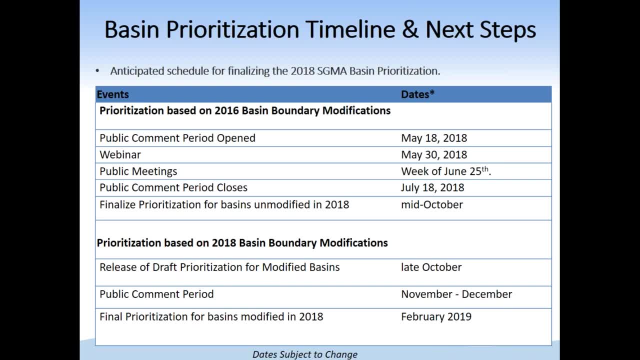 So there is, as I mentioned earlier, there are, a couple of different related SGMA activities going on: Basin prioritization, which, as Trevor mentioned, is a result of the 2016 Basin Boundary Modification. There is a current Basin Boundary Modification window open right now and there'll be – these: 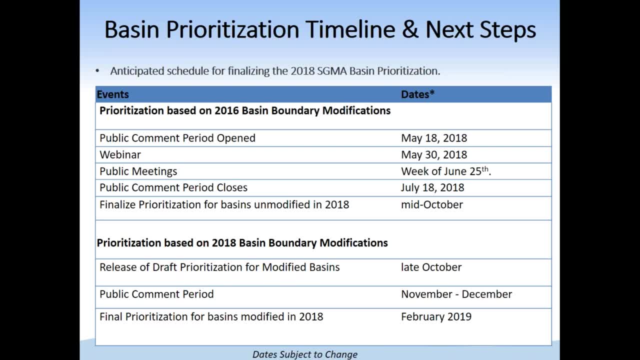 multiple projects will be aligned and I'll show that On the next slide. but the prioritization based on the 2018 Basin Boundary Modification. the plan is to release draft prioritizations for the modified basins- if there are basins that are modified as part of that Basin Boundary process- in late October. 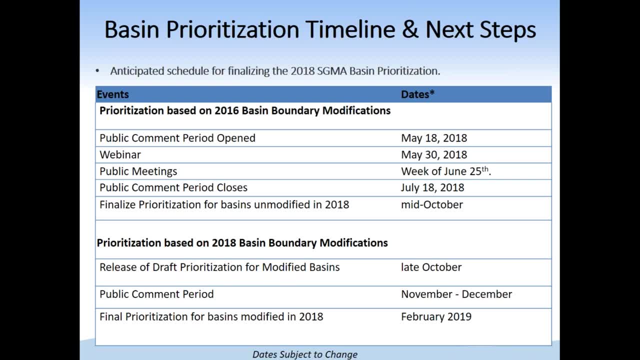 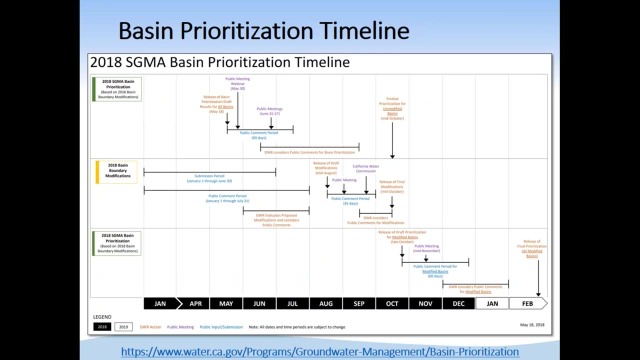 There will be a public comment period for that reprioritization and then final prioritization for those modified basins. Modified basins would be in the early 2019 timeframe. So, as I mentioned, this timeline of these various related activities is available on. 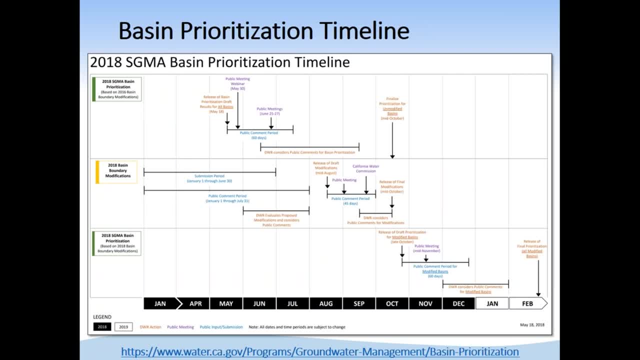 the website. They're on the screen on our Basin Prioritization website. It's hard to see here on the screen, but you can see these three distinct and related projects: the 2018 SGMA Basin Prioritization that we're talking about today. the 2018. 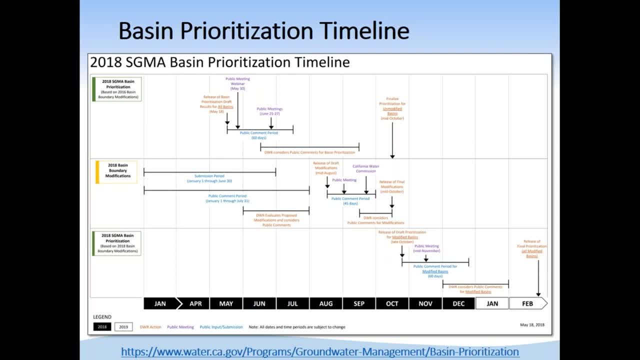 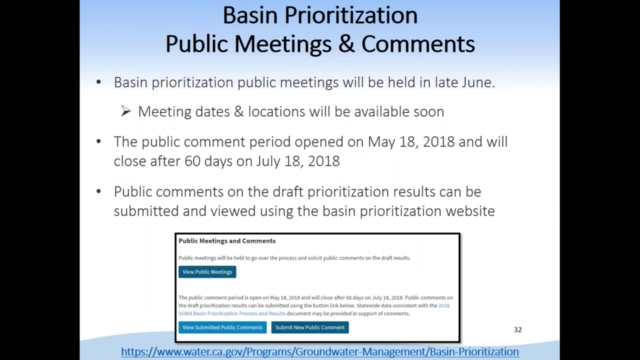 Basin Boundary Modification process that's currently underway, with a submission period that ends June 30th, and then the 2018 Basin Prioritization related to any basins that change as a result of this next round of Basin Boundary Modification. So how to provide public comments? 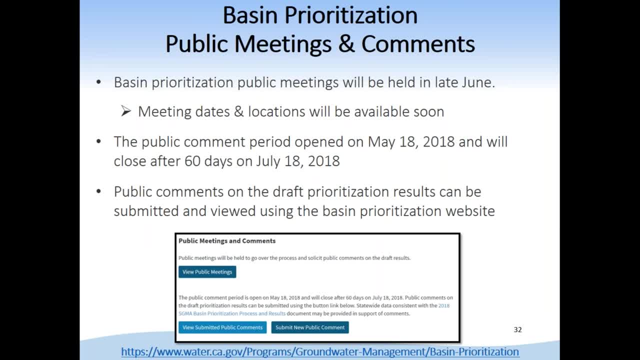 And then where, And some additional information on the public meetings. On the public meetings, I mentioned that those will be held in late June, the week of June 25th, and more details on those dates and locations will be available soon. The public comment period opens the 18th and will run for 60 days and close on the July. 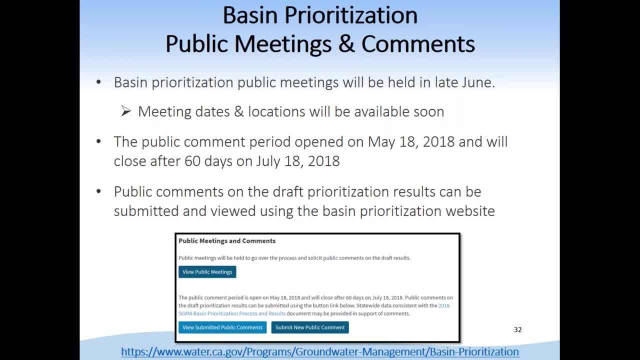 18th. Public comments on the draft prioritization results can be submitted and viewed using the Basin Prioritization website. Here's a screenshot of that part of the website where you can view the public meeting information, as well as view submitted public comments and submit new public comments here. 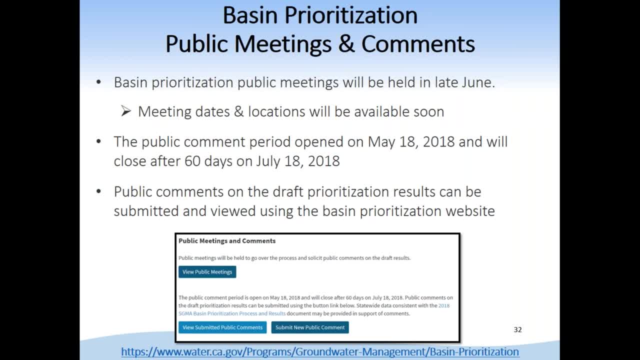 There is an important distinction between providing questions for clarification to that email that I mentioned earlier and official public comments. So those we're requesting all official public comments on prioritization be submitted, And any related data sets that accompany those public comments need to be submitted to this. 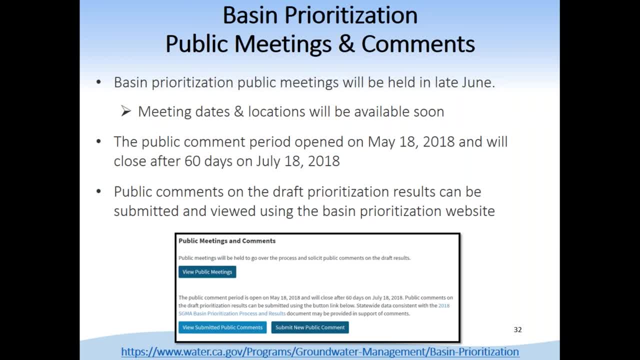 website as well, if you are planning to submit additional data. So some highlights on how to provide effective comments on prioritization: We're looking for comments that focus directly on the draft 2018 SGMA Basin Prioritization results, And also comments that identify the specific water code components that Roy touched on. 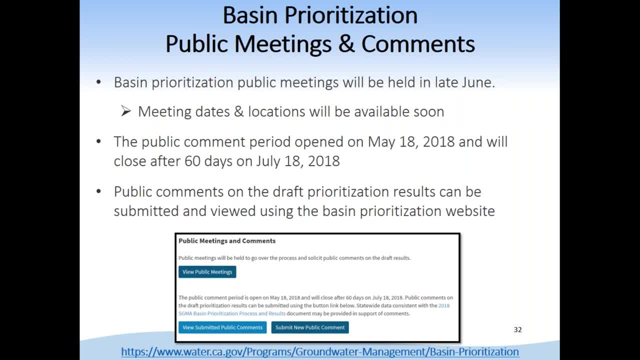 that are being commented on or specific references or citations that are being provided related to those various components of Basin Prioritization. As I just briefly mentioned, the supporting data that are submitted as part of a comment or with comments, should be consistent with the 2018 SGMA Basin Prioritization results. 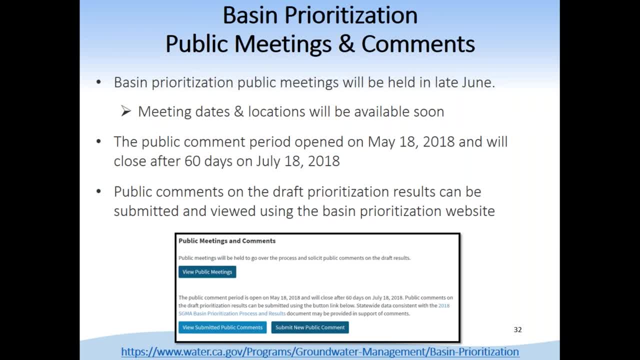 So we're looking for comments that focus directly on the draft 2018 SGMA Basin Prioritization process and results document that I showed on the screen and that Roy went over, And so there are some different avenues here, as I just mentioned. 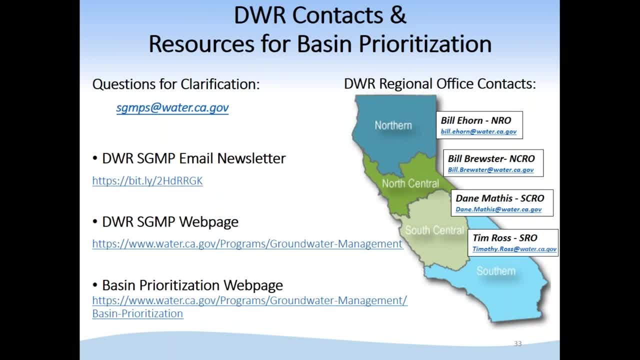 So future questions for clarification- so again, not public comments- can be submitted. We want to centralize those questions for clarification that aren't addressed today to that SGMA program email And we're looking for comments that focus directly on the draft 2018 SGMA Basin Prioritization. 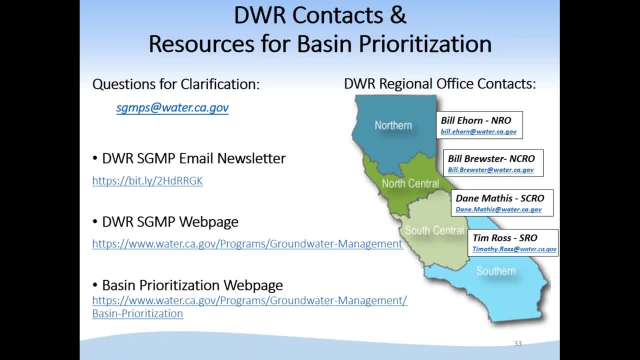 process and results document that I showed on the screen and that Roy went over. The next thing they're looking for is the: is the contact there? our north central regional office in west sacramento, bill brewster, is the contact there, and then our south central regional office is dane mathis and that's in the fresno. 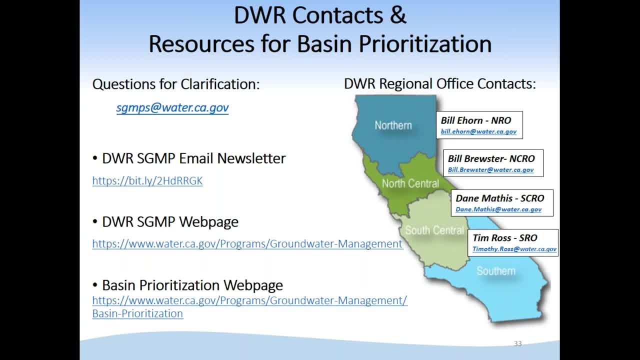 office and then our southern regional office is in glendale and that's timothy ross. so, as trevor mentioned, those basins that moved from lower, very low, to medium or high and are starting their new path into sigma. after these results are finalized, there are a number of services and 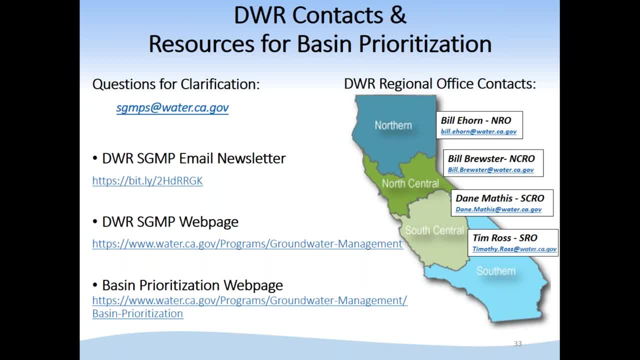 support that DWR provides, planning technical and financial support- and we are planning to to continue those services and we are planning to continue those services and we are planning to continue those services and we are planning to continue those services. and there's additional services and there's additional information on those variety of services on our main DWR. 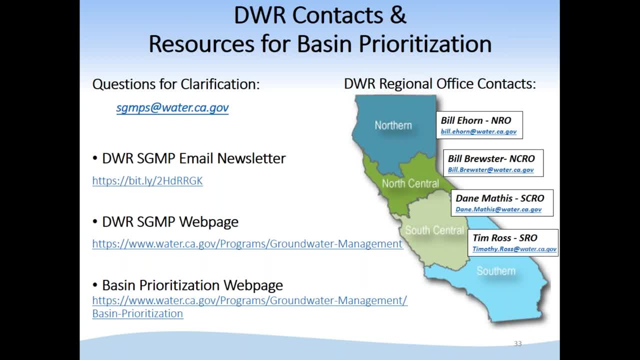 sustainable ground water management program website, which is a link is there on screen, and another good source of information on the latest info and updates on the DWR Sigma program if you sign up for the email newsletter that goes out- the bike bi-weekly newsletter. that has a link to the newsletter. that has a link to the newsletter. that has a link to the newsletter. 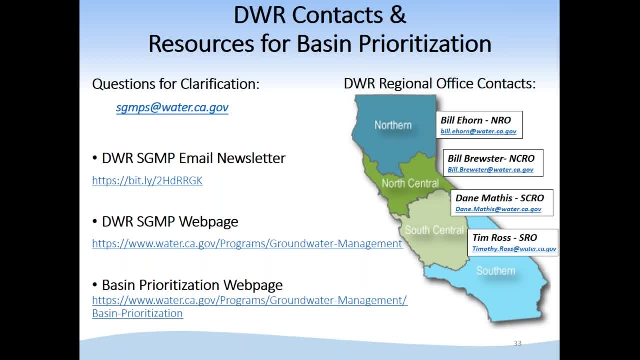 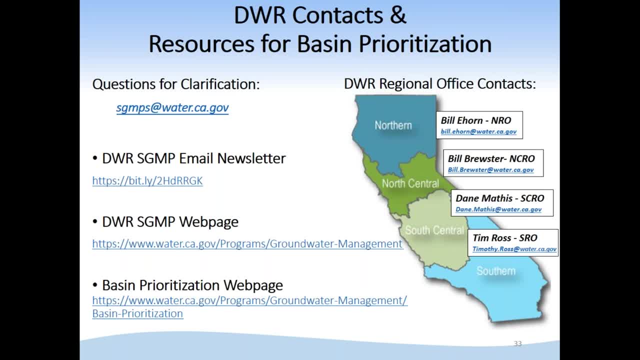 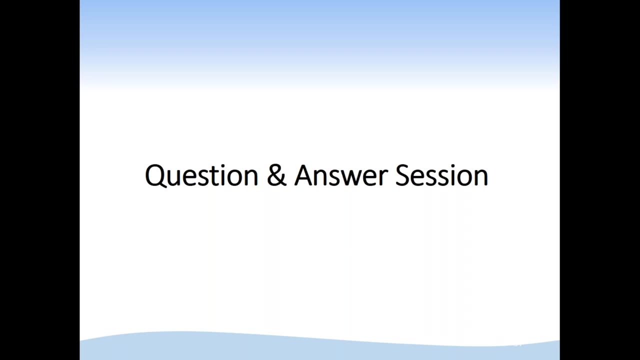 variety of services and data tools that we have available for for the Basin, for those stakeholders, and GSA is in the basement throughout the st. almost so, with that all, I turn it over now to definitely and she'll walk through the question and answer session. great, thank you, Steven. so this: 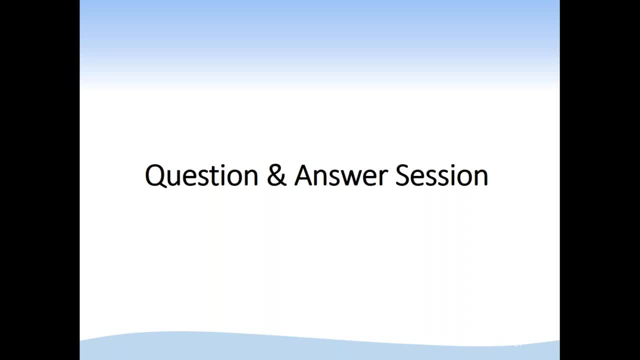 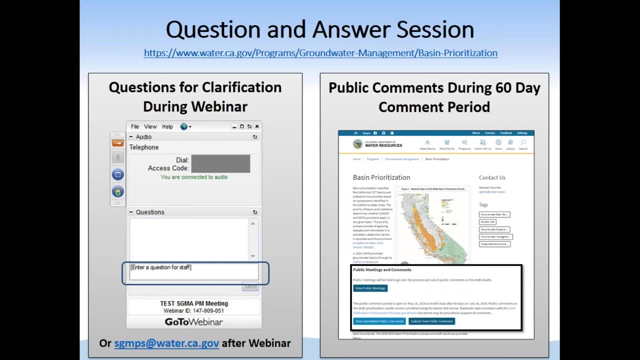 is the time for clarifying questions. we receive, in a minimum, Yetman of artist with a solution. that means we have tent奇怪 ask you over the course of this webinar, which is wonderful, to remind you all of how you can submit those clarifying questions. use that questions box on your 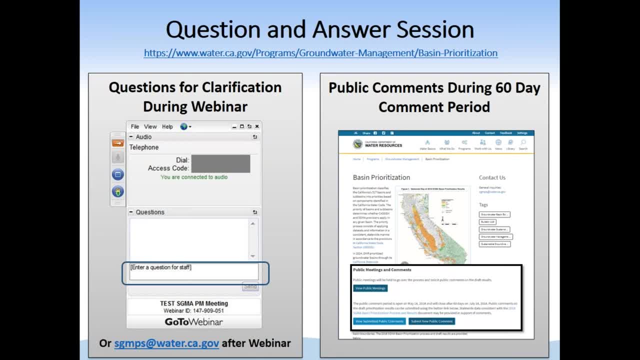 control panel and remember that this is for clarifying questions on the presentations that you've heard today. if you want to provide a formal public comment again, as Stephen indicated, you would go to the basin prioritization web page on DWR's website for those official public comments. that will be. 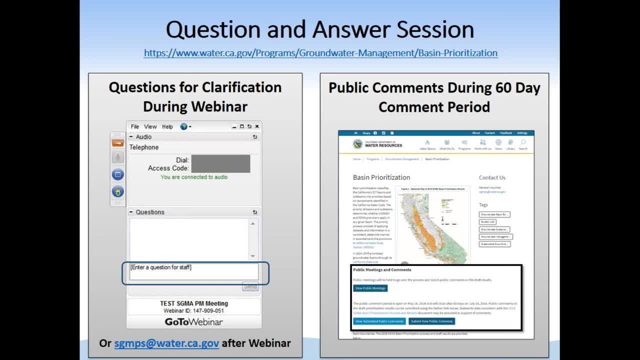 posted publicly. so with that, I'll turn over back to Stephen to moderate the questions. we've received all right. Thank You, Stephanie. so we do have a number of questions here, so we'll be. we have our colleagues from the Sigma program, Simra Denoda and Tim Godwin, that are helping us stage the questions, and Tim will be. 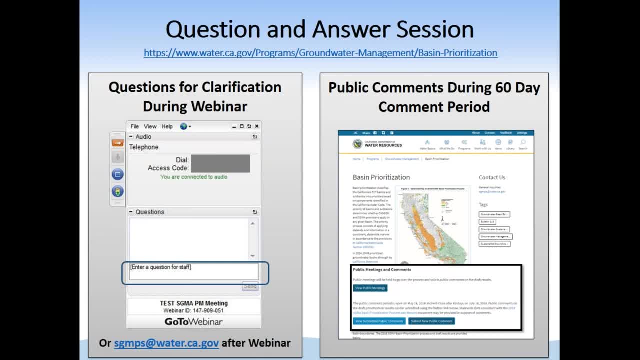 reading out the questions and our team here will be answering the questions. so go ahead. thanks, Stephen. so let's start off. we've been talking a bit about the comments, but I'll dive right in that one, because I think it's a strong one. is DWR accepting comments on the priorities for all basins, including? 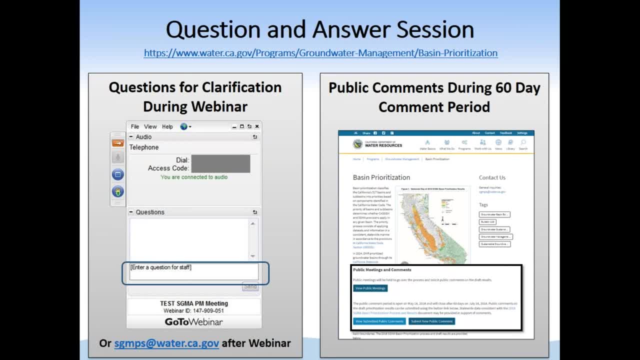 those for which the priority did not change. yes, real short answer. yes, I mean, we accept comments on all the basins, regardless of the changing and priority, even regardless of whether it changes from low or very low to medium or high or vice versa. great, I'm going to simplify this one a little bit so it can. 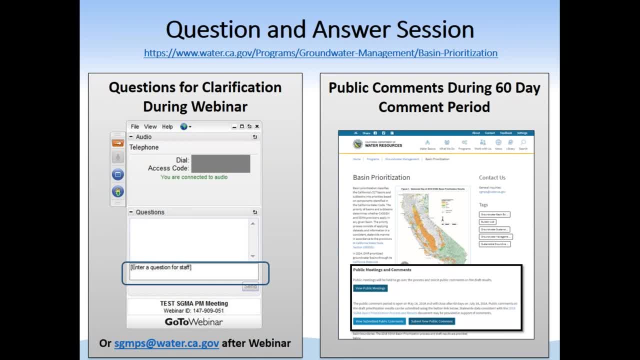 be applied across the state. but why are the out of basin groundwater substitution transfers selected for the Sacramento Valley, you know what, where where basins are considered healthy? why? why is this component added in this? yeah, this is a really good question. that kind of gets at. another point we perhaps failed to mention is what prioritization really? 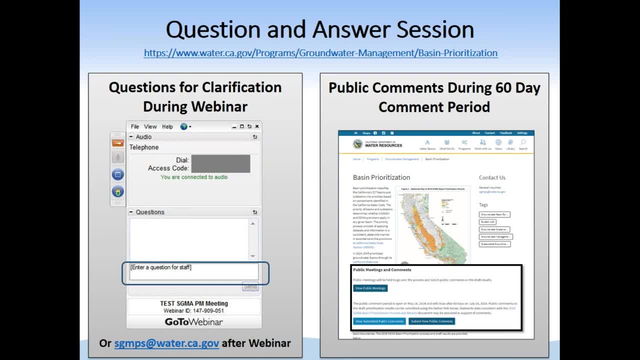 means prioritization is not a judgment by the Department of Sustainability, or even a judgment as it relates to whether there's groundwater management or sufficient groundwater management, or sustainable groundwater management, and it's really just a characterization, that identification, I should say, of the importance of groundwater management as it relates to the sustainable groundwater. 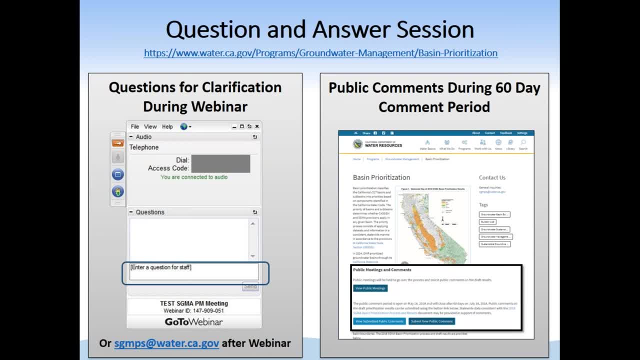 management act. so whether there are basins that are medium or high, or even if those have changed priority from medium to high, it doesn't indicate at all a statement by the department that they are unsustainable in any way. it just recognizes the importance of the management of those basins, for them to be managed in accordance with the 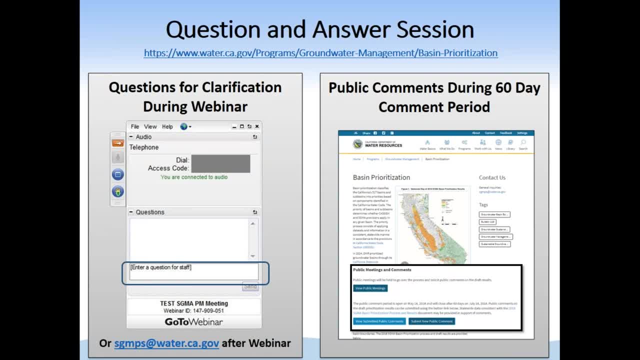 sustainable groundwater management act. we've had a pretty limited list of questions. however, some are still flowing in, and give me just a moment here see if we can pull another one in. you know, I do see a question, Tim. maybe if I could just add a couple of things that I want to. 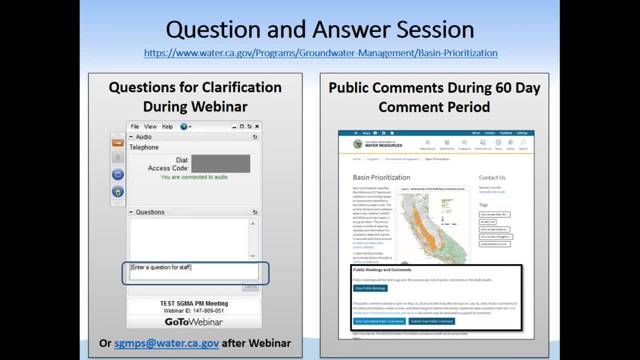 add, there seems to be a question related to groundwater substitution transfers, and I want to make a statement here that you know: the state does not in any way feel that groundwater substitution transfers are important, in fact, quite the opposite. this is something that we encourage, is one of. 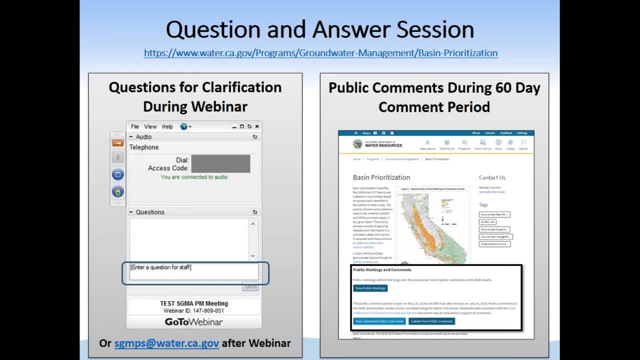 the tools to reach statewide water management, and so groundwater substitution transfers back to the state. these are not just these are not just the to my prior point- potentially have a risk of greater significant impacts, and so should be done in accordance with the Sustainable Groundwater Management Act. 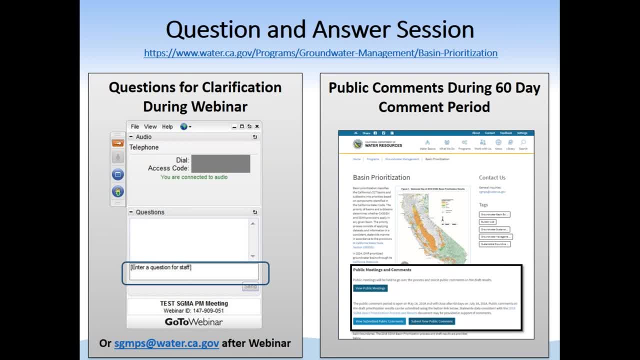 So again, it's not a judgment in any way that they are not achieving their goals related to those programs, but should be done in accordance with the Sustainable Groundwater Management Act. So this question in regards to the priority point ranges and how these components 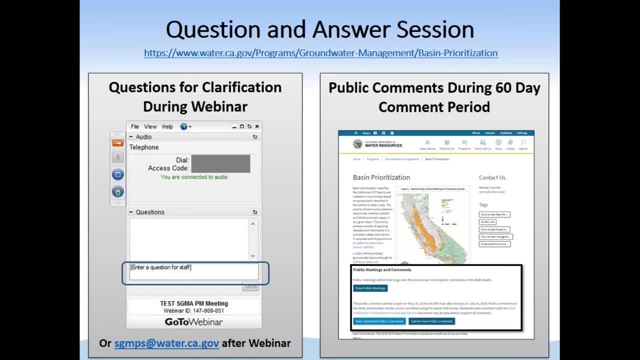 were broken down and characterized. What was there? Was there a new methodology applied that changed these ranges and the minimums and maximums? How did these components roll up to defining the priority? I think is what we're really after in this question. There's a couple of pieces to that. 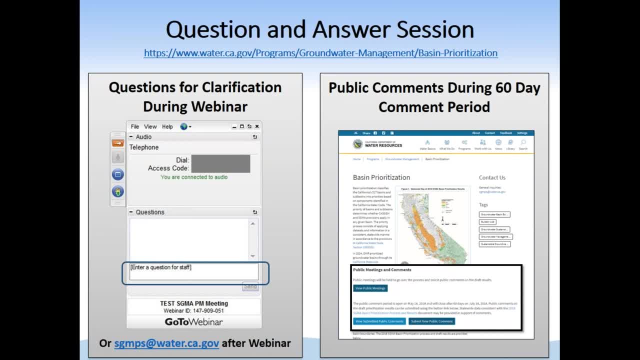 Number one: we wanted to try to maintain as much consistency between 2014 and 2018 and not have a lot of… Uncertainty with respect to people understanding where they kind of reside. They would be able to look at that and be able to predict if there's changes occurring. 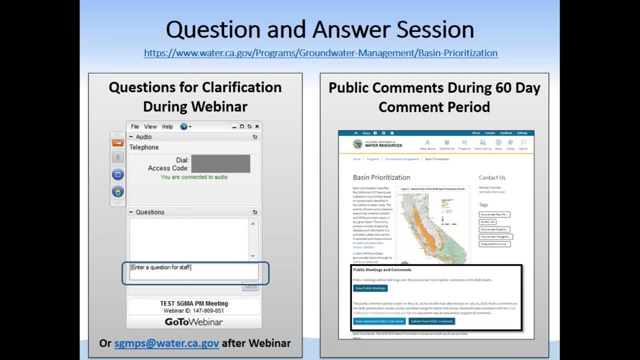 in their basin, where they would actually…how that would impact their prioritization Number two. another factor is that the previous prioritization did not consider all the factors that are in 2018, such as ground. That's a good point. 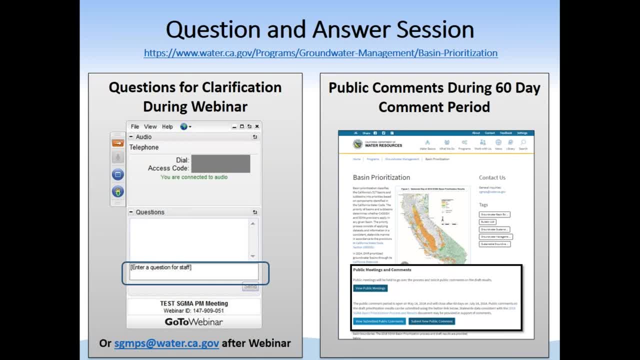 Yeah, So the previous prioritization, the previous prioritization was around the habitat and stream flow. So we increased the number of points from 40 to 42. So we had to make some allowances for that increase. So that's why we went from like 13.42 for a medium to greater than 14 was for a better. 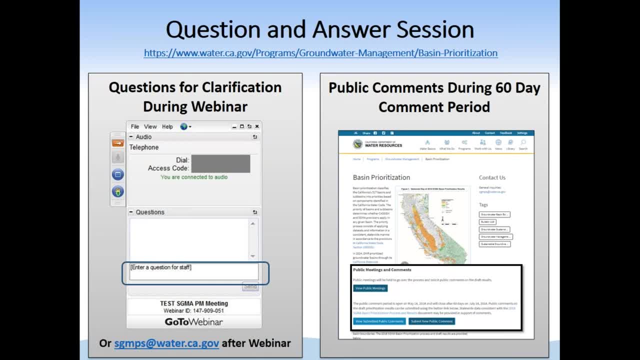 distribution, taking into consideration those extra points. So we didn't change the points to maintain consistency and public understanding of what we're looking for. And then we also had to allow for some changes due to the new requirements on the prioritization. Thanks, Roy. 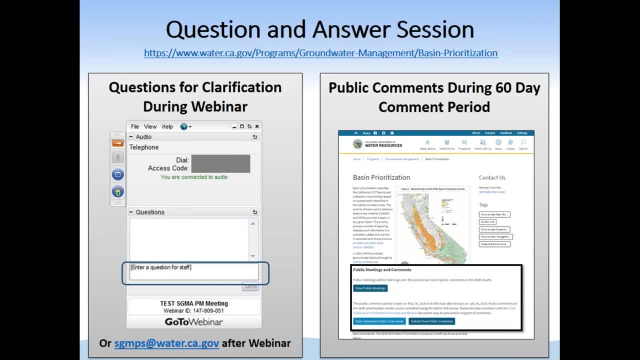 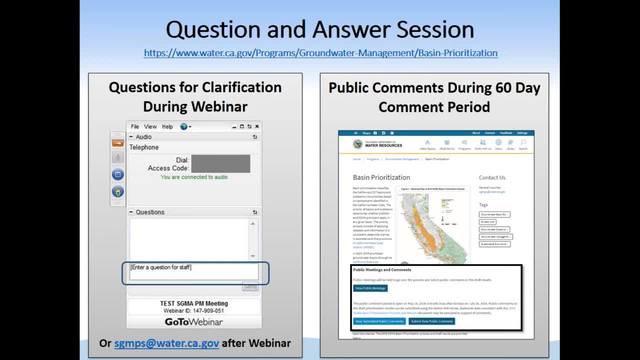 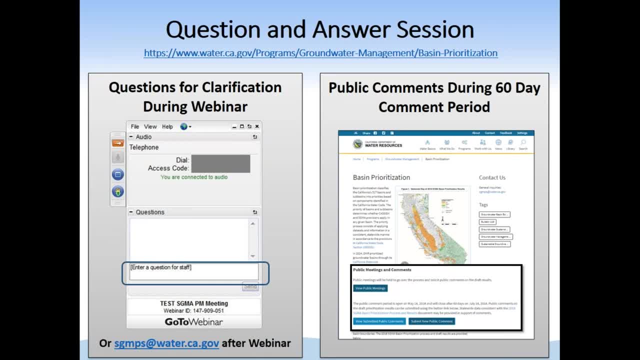 like that. It was really hard for us to make any kind of assessment to say that this was more important or more of an impact infrastructure than another place, that there's just no easy way to determine that in the scope of basin prioritization. So we treated subsidence essentially. 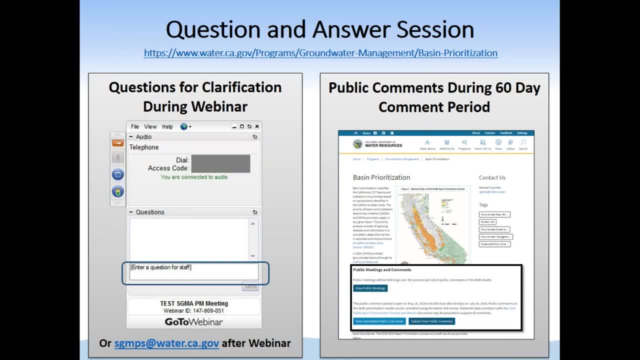 it was a yes, sir, and now is there prior. is there some sites occurring in that basin due to groundwater activities? great then, I guess, to drill in a little further on the public supply. well, there is question regarding the timing of the querying of the database. is there any significance to us pulling the data from? 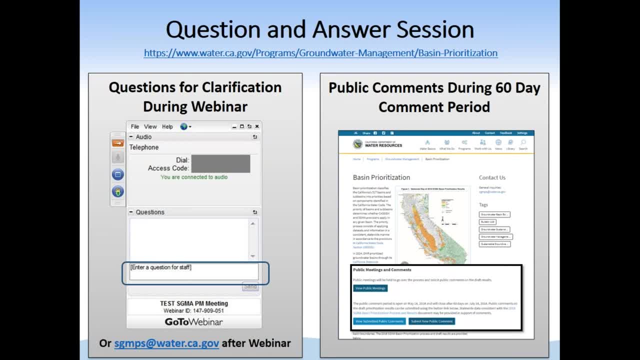 March 2016. why didn't we update it for early 2018? hmm well, we pulled the data when we, back in March in 2016- remember this was there's a lot of different components to this thing and it was a snapshot in time to give us an idea of. 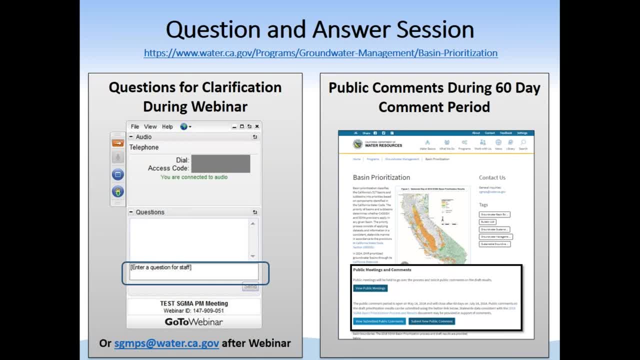 what was what was being used in that basin. if we probably pulled it today we might get a slightly different number, but it would be different wells, so there really wasn't a whole lot of importance in trying to upkeep that data set: update, updated. plus there's a rather 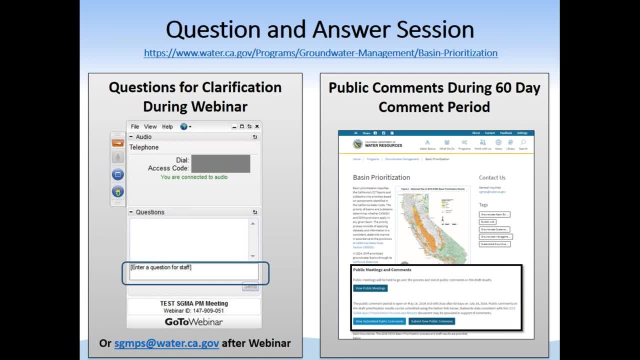 you know, rather long process for getting true to final approval to be able to release this. so at the time when we started that process it was a rather young data set. great, we'll jump back kind of on the topic you touched on earlier: Trevor. are there any additional or? 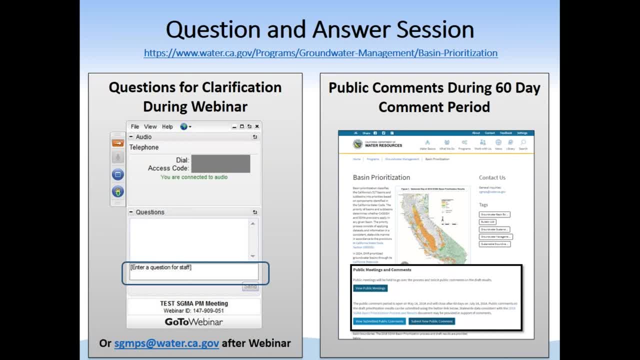 Stephen, are there any additional requirements from Sigma when you consider high priority versus medium priority? so in the short answer there is: Sigma treats these two priorities the same way and so therefore there's really no difference in the requirements for high or medium priority basins. so that 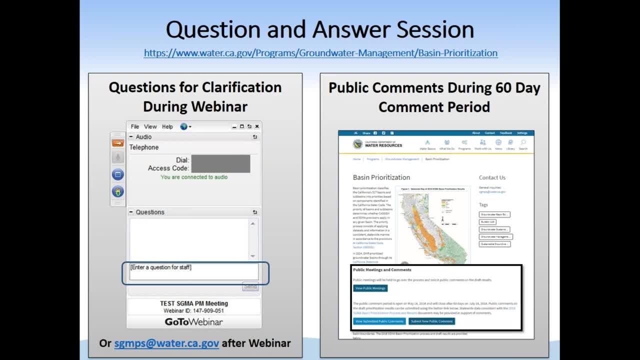 being said, Sigma applies to all groundwater basins identified in Bolton 118 and, but Sigma requires that all high and medium priority basins be managed under a GSP or alternative. so for those low and very low basins, Sigma encourages and authorizes the development of a GSP or alternative but not does not require it. 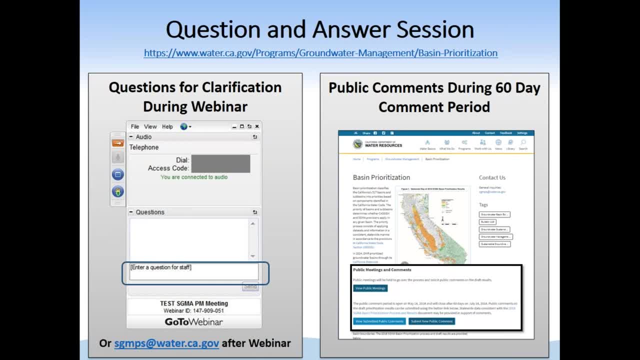 great looking forward the future other than they've been. the basin boundary modification should occur coming up. is there any other mechanism to trigger basin prioritization moving forward? this way to answer that is, we have no plans to further evaluate prioritization. the foreseeable future, meaning the next. I. 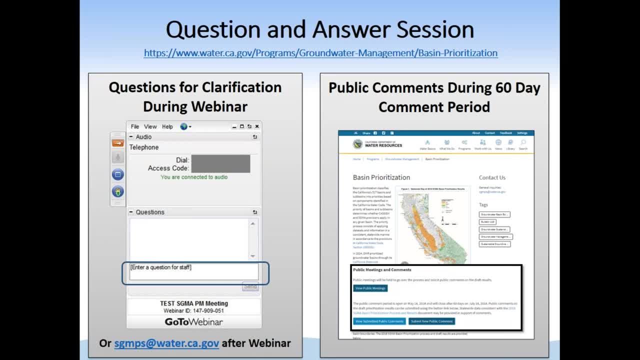 would say three to five years. that's the current plan. it's always possible that that could be subject to change but, as you point out to him, he's going to have to try to find a way to solve some of the gaps later with the, with the exception of basins that are modified as part of the second round of 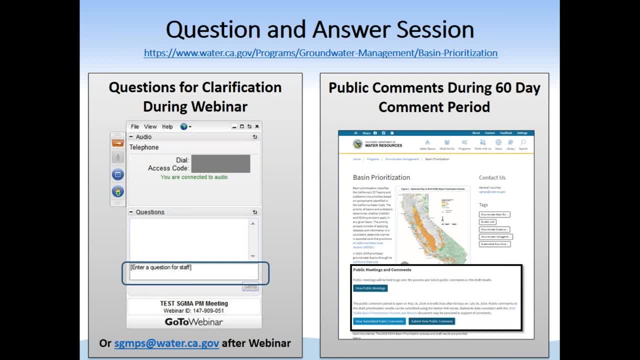 based in boundary modifications, those basins that are modified. we have an obligation to look at late this year and hopefully finalize that prioritization of just those basins, as Steven mentioned in his portion of the presentation. right again, some more technical information regarding how we the base data sets here in looking at the Oscar database. how did we, did we? 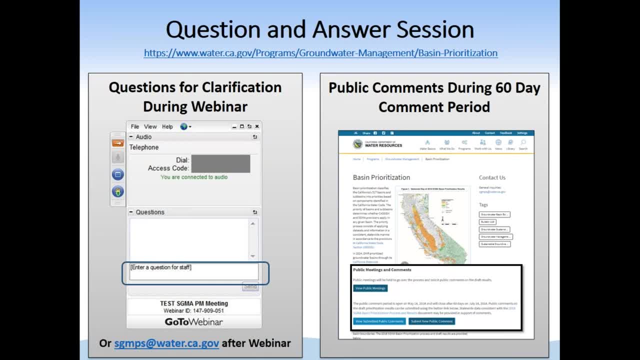 take into account that there are destroyed or inactive wells in our data set, getting those total well counts for these basins? well, the short answer is no, but the long answer is: is that currently, the the data set from Oscar is is essentially an accumulation of all the wells and they and we're not tracking or 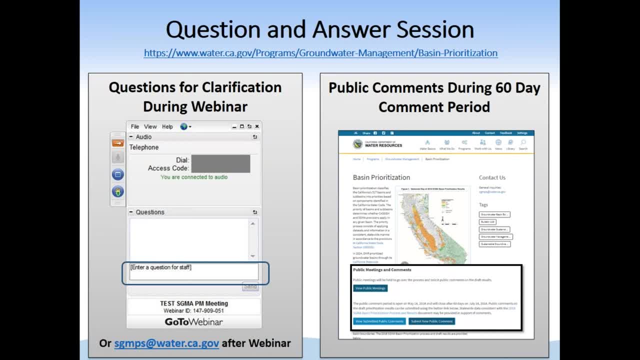 matching destroyed wells versus installed wells, which is unfortunate. but that's a lot of that's a lot of work to go back and try to figure out all that. but no, we didn't. but the other downside to that is that not all well logs are submitted to DWR, so we don't receive all the logs, whether it's destroyed or 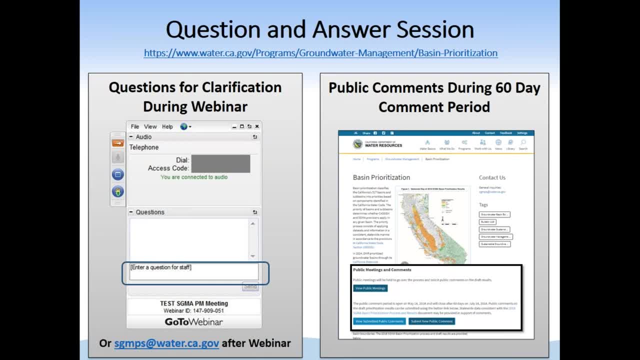 whether it's it's a new well log. so the right answer is no, but the long answer is no. but the long answer is no, but the right answer is no, but the wrong answer is no, but the wrong answer is no. but the reconciliation of that is probably next impossible at this point. okay, thanks, 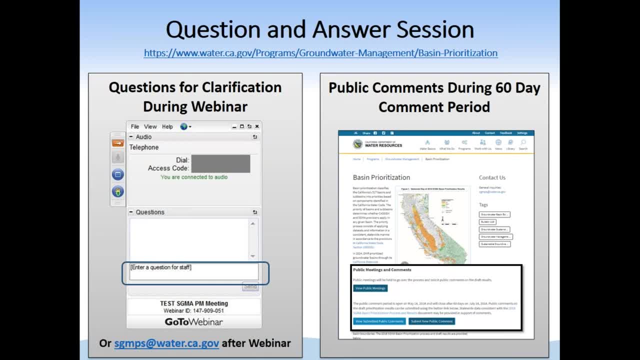 right um, looking at component 8, C, C 1 and C 2, those those being, I believe, the type on stream flow and habitat. those those being, I believe, the type on stream flow and habitat. those those being, I believe, the type on stream flow and habitat. that correctly, sorry, I'm probably drawing. 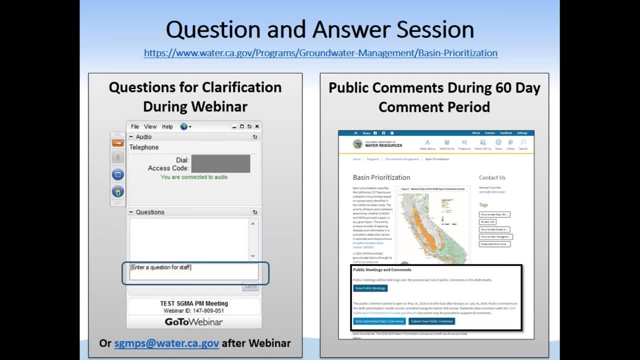 that correctly. sorry, I'm probably drawing that correctly. sorry, I'm probably drawing it wrong. it wrong, it wrong. those are the the two thousand and ninety five hundred eight oh one, and those are the the two thousand and ninety five hundred eight oh one. and those are the the two thousand and ninety five hundred eight oh one and eight C two right are. well, so are those. 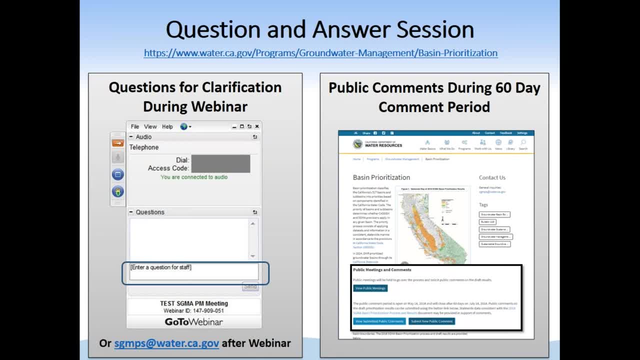 eight C, two right are well, so are those. eight C, two right are well, so are those. are those components, those, those metrics, are those components, those, those metrics, are those components, those, those metrics, are they always the overriding? are they always the overriding? are they always the overriding consideration? 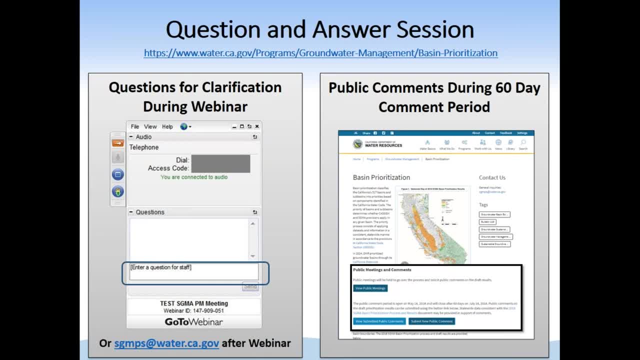 consideration, consideration regardless of point, I mean. how do those regardless of point? I mean. how do those regardless of point? I mean, how do those fit into where these things get ranked? fit into where these things get ranked fit into where these things get ranked with regards to the other component. 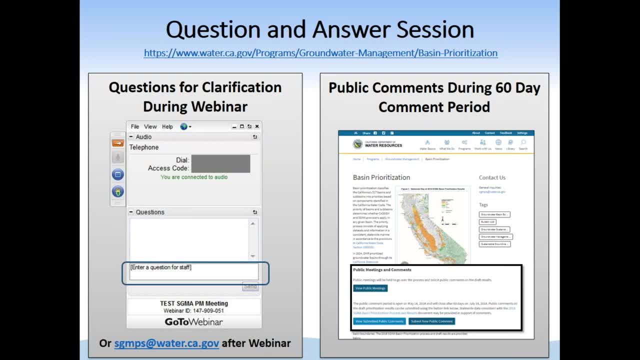 with regards to the other component. with regards to the other component: point totals- that's a test analysis. point totals: that's a test analysis. point totals: that's a test analysis. that's done. I mean the whole point of that's done. I mean the whole point of. 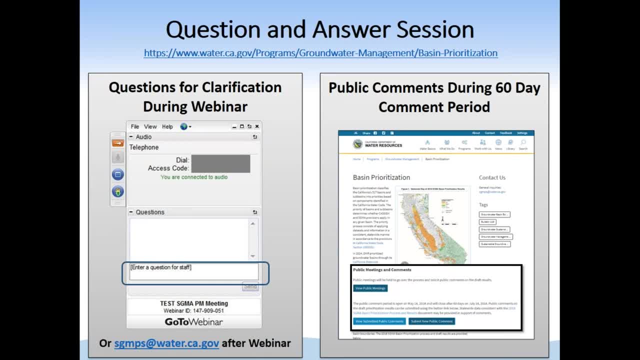 that's done. I mean the whole point of basin prioritization and all points of basin prioritization and all points of basin prioritization and all points of Sigma is related to groundwater and its Sigma is related to groundwater and its Sigma is related to groundwater and its and its groundwater use that the basin is. 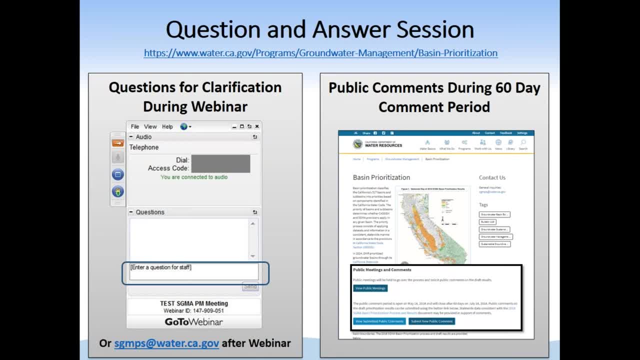 and its groundwater use, that the basin is and its groundwater use, that the basin is nobody's pumping any groundwater in, nobody's pumping any groundwater in, nobody's pumping any groundwater in that basin. you know at some point you that basin. you know at some point you that basin. you know at some point you have to be reasonable and say, well, you. 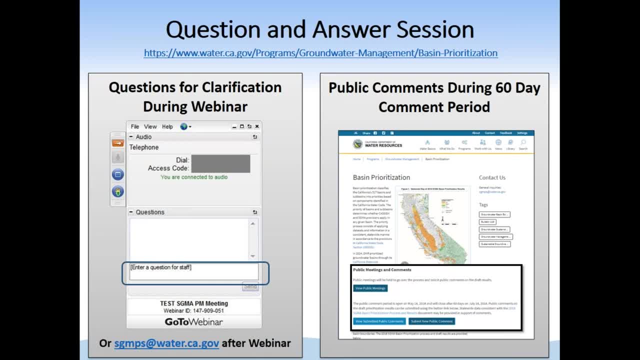 have to be reasonable and say, well, you have to be reasonable and say, well, you know, should they develop a groundwater? know should they develop a groundwater, know should they develop a groundwater management plan. if they're not doing management plan, if they're not doing management plan, if they're not doing pumping any groundwater, so that same. 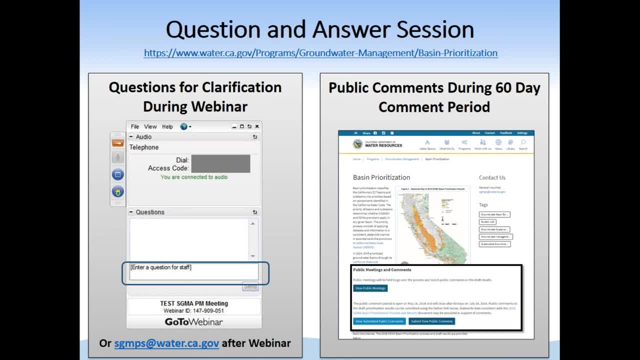 pumping any groundwater, so that same. pumping any groundwater, so that same. those same numbers were used in 2014. we those same numbers were used in 2014. we those same numbers were used in 2014. we also used them in 2018, in a way to 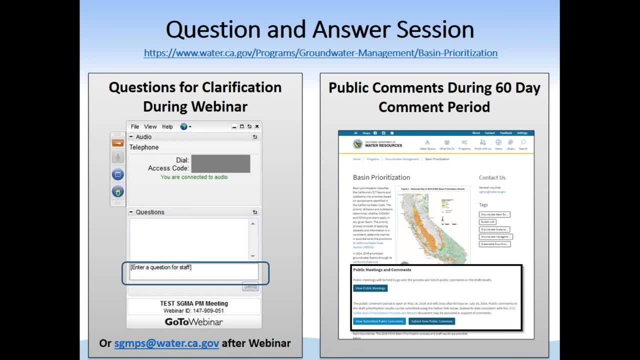 also used them in 2018 in a way to also used them in 2018, in a way to basically say you know there's no. basically say you know there's no. basically say you know there's no groundwater volume and it's amazing that groundwater volume and it's amazing that. 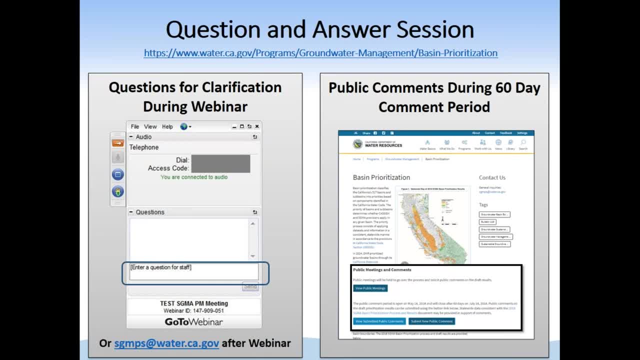 groundwater volume and it's amazing that there's are- there are a lot of basins there's are. there are a lot of basins there's are. there are a lot of basins out there that do not pump any, out there that do not pump any. 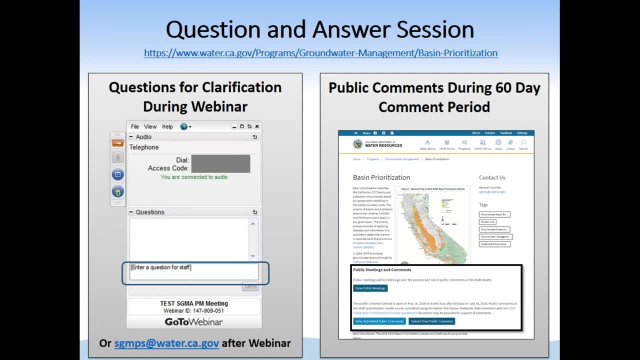 out there that do not pump any groundwater. so we wanted to be able to groundwater. so we wanted to be able to groundwater, so we wanted to be able to capture that and basically identify, capture that and basically identify, capture that and basically identify that there are some basins because of 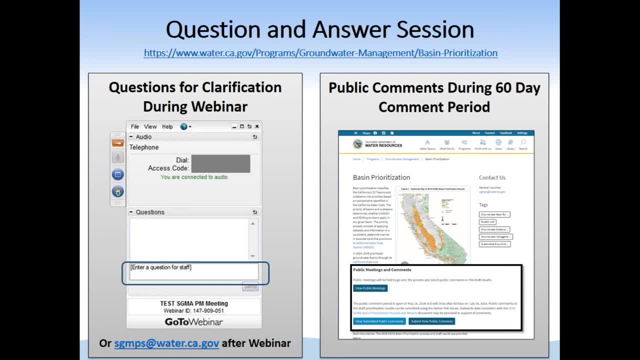 that there are some basins. because of that there are some basins. because of some of the other criteria, because of some of the other criteria, because of some of the other criteria, because of population and other circumstances. they population and other circumstances, they population and other circumstances. they could be all irrigated acreage. however, 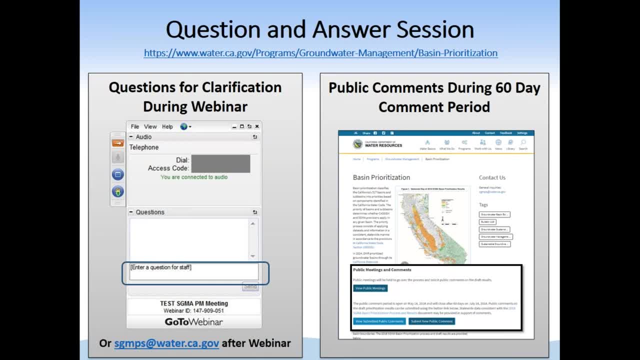 could be all irrigated acreage, however, could be all irrigated acreage. however, it's all surface water is the source, so it's all surface water is the source, so it's all surface water is the source, so they can end up having very high, very 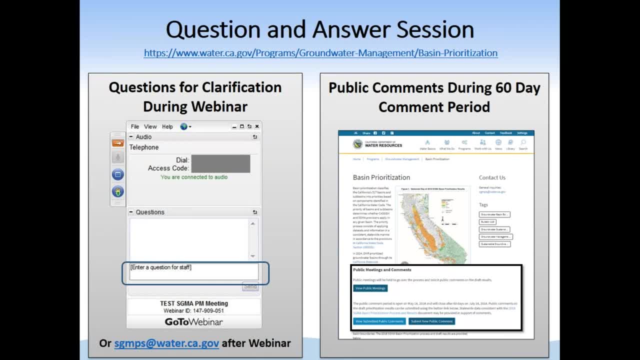 they can end up having very high, very. they can end up having very high, very large number of points, but in the end, large number of points but in the end large number of points, but in the end they don't pump any groundwater or not a. they don't pump any groundwater or not a. 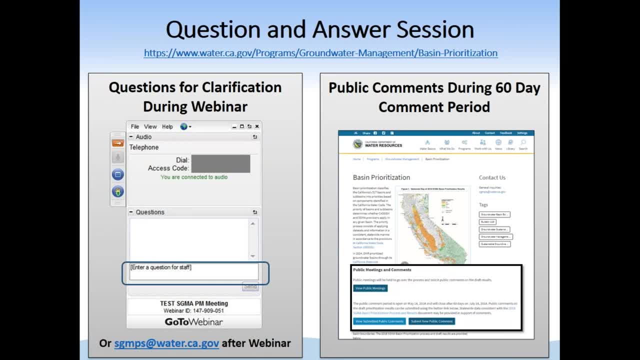 they don't pump any groundwater, or not a sufficient amount of ground in order to sufficient amount of ground in order to sufficient amount of ground in order to make, make, make. sorry, the questions keep trickling in. sorry, the questions keep trickling in. sorry, the questions keep trickling in. we're trying to get them canned, we're. 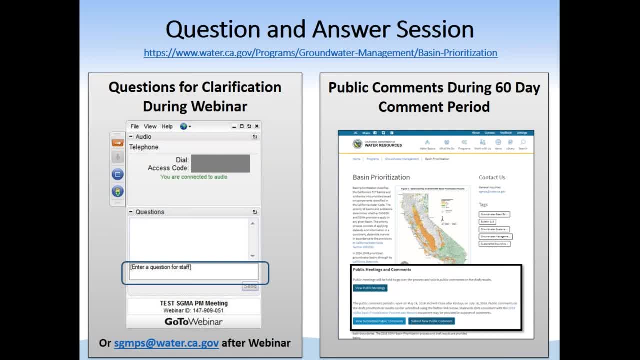 we're trying to get them canned. we're we're trying to get them canned. we're going to try and respond to as many as going to try and respond to as many as going to try and respond to as many as we can. there are some very specific. 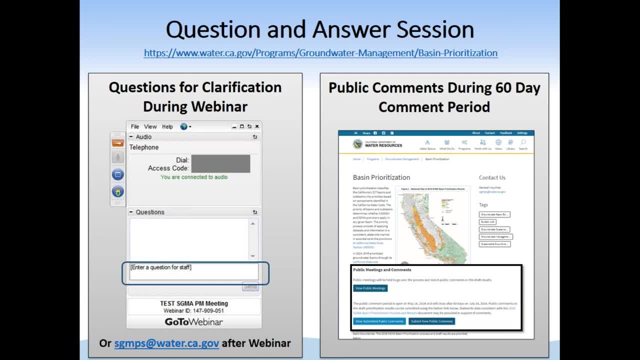 we can. there are some very specific we can. there are some very specific questions that you know be happy to, to questions that you know be happy to, to questions that you know be happy to. to drill down a little bit deeper on in. drill down a little bit deeper on in. 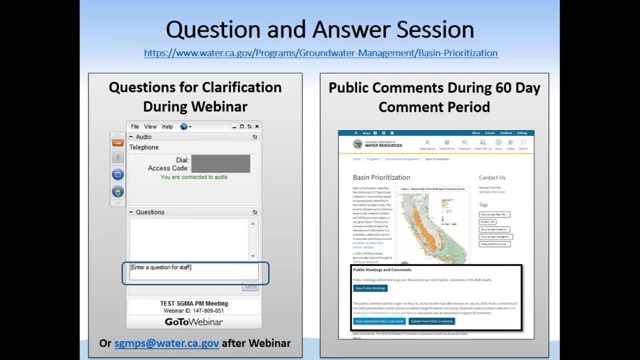 drill down a little bit deeper on, in person, or with specific basins or person, or with specific basins or person, or with specific basins or prioritizations in mind. yes, this one prioritizations in mind. yes, this one prioritizations in mind. yes, this one here, the the process results documented. 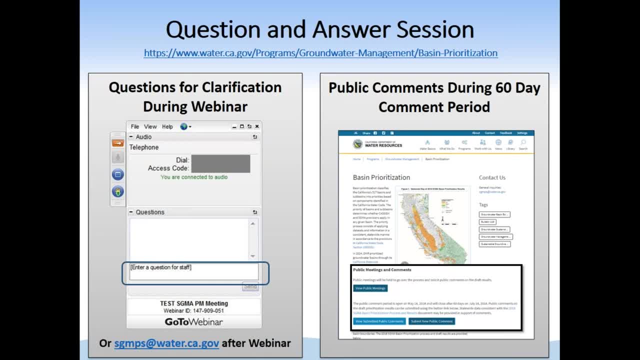 here: the the process results documented here: the the process results documented notes that all agriculture mapped in. the notes that all agriculture mapped in. the notes that all agriculture mapped in the 2014 data set was assumed to be. 2014 data set was assumed to be. 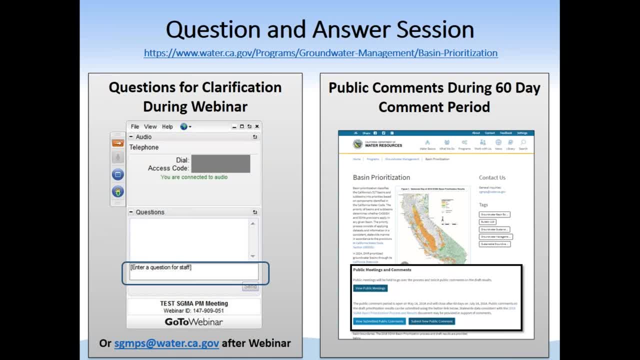 2014 data set was assumed to be irrigated unless a field had been irrigated. unless a field had been irrigated unless a field had been previously identified by DWR is dry. previously identified by DWR is dry. previously identified by DWR is dry farm. does that include prior? 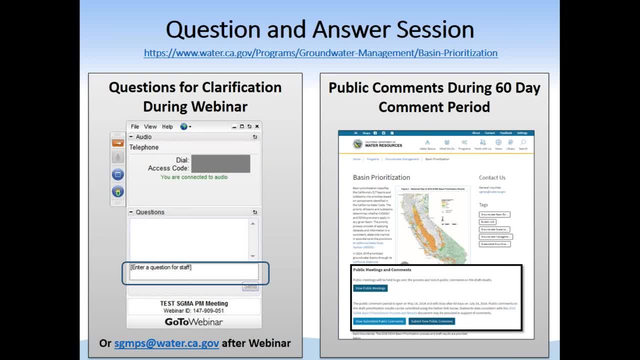 farm. does that include prior farm? does that include prior designations made in earlier DWR land use designations made in earlier DWR land use designations made in earlier DWR land use maps- not specifically. we worked with maps, not specifically. we worked with maps, not specifically. we worked with the land use folks in the different 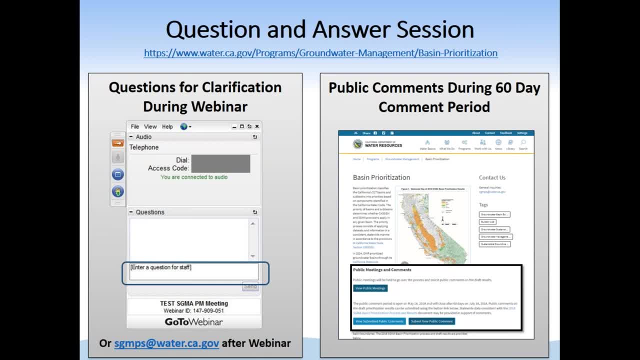 the land use folks in the different the land use folks in the different regional offices. they used current regional offices. they used current regional offices. they used current knowledge of what was going on, in knowledge of what was going on, in knowledge of what was going on in particular, the year 2014. so, if it was, 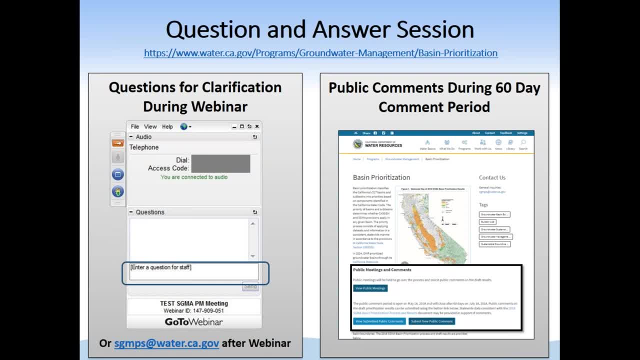 particular the year 2014, so if it was particular the year 2014, so if it was dry farmed in, you know 2008 that wasn't dry farmed in. you know 2008 that wasn't dry farmed in. you know 2008. that wasn't what our criteria was. what was its? 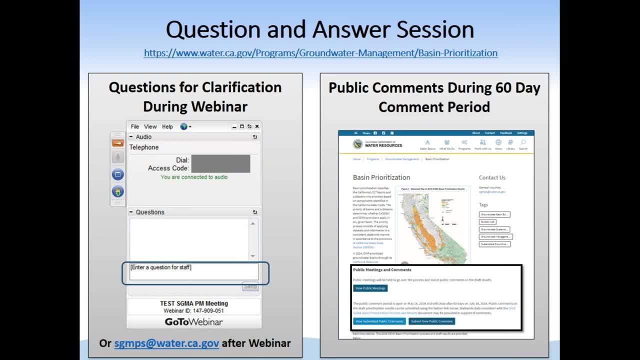 what our criteria was. what was its? what our criteria was. what was its condition? what was its irrigation source condition? what was its irrigation source condition? what was its irrigation source or not? and it had to do with 2014, so we. or not. and it had to do with 2014, so we. 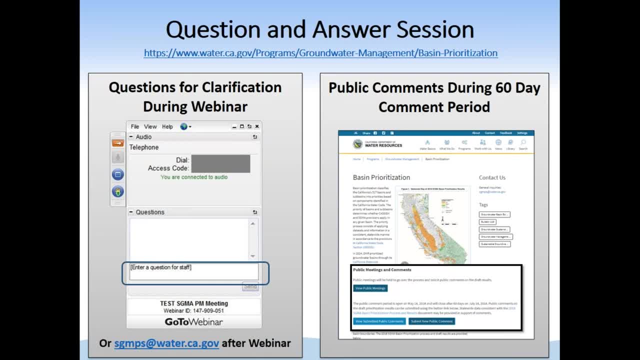 or not, and it had to do with 2014. so we might use the older DWR land use, might use the older DWR land use, might use the older DWR land use surveys to try to identify some of those surveys, to try to identify some of those. 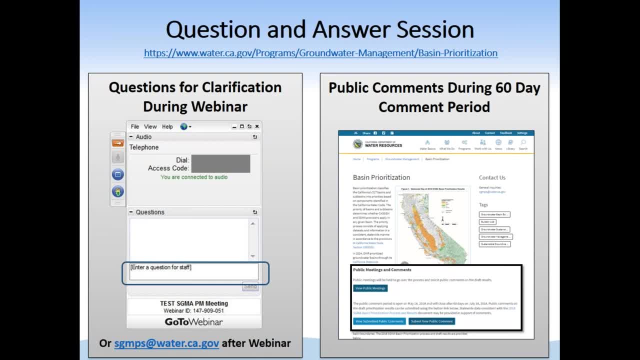 surveys to try to identify some of those, but then we apply 2014 knowledge to it. but then we apply 2014 knowledge to it, but then we apply 2014 knowledge to it. okay, all right, so it looks like we're okay. all right, so it looks like we're. 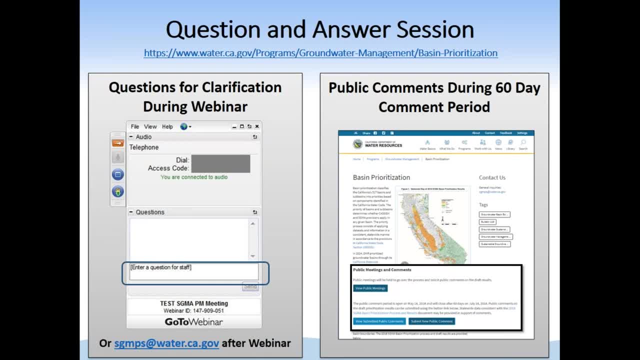 okay, all right, so it looks like we're. we might take a short break, our pause. we might take a short break, our pause. we might take a short break, our pause, just to compile, if there's any other, just to compile, if there's any other, just to compile, if there's any other questions that come in. so again you, 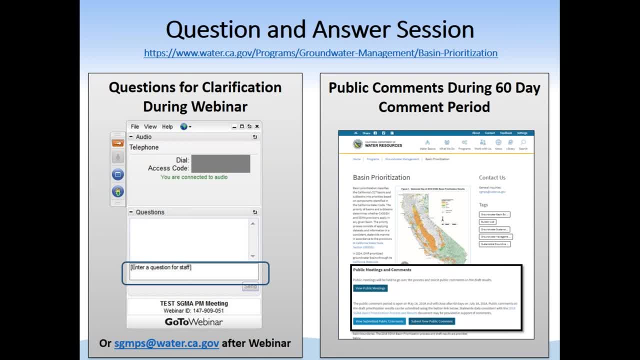 questions that come in. so again you questions that come in. so again you have any questions for clarification. what have any questions for clarification? what have any questions for clarification? what was presented today? please submit those was presented today. please submit those was presented today. please submit those. so we'll we'll look for those and 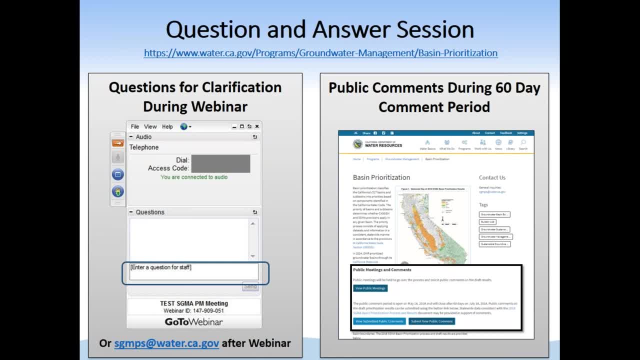 so we'll, we'll look for those, and so we'll, we'll look for those and compile them. so just a quick pause here, compile them. so just a quick pause here, compile them. so just a quick pause here to do that, to do that. so just a quick pause here to do that. 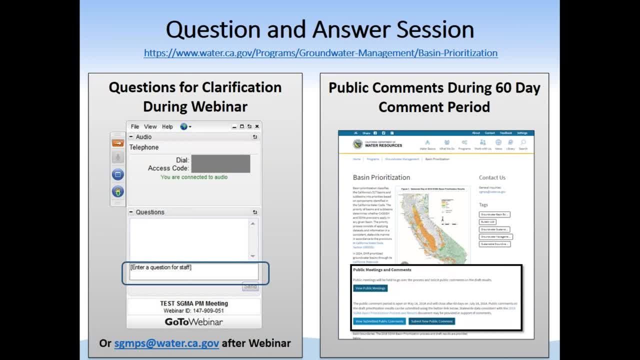 to do that. all right, looks like we have a few. all right, looks like we have a few. all right, looks like we have a few additional questions. go ahead then yep. additional questions go ahead then yep. additional questions go ahead then yep. so a question here on on how subsidence 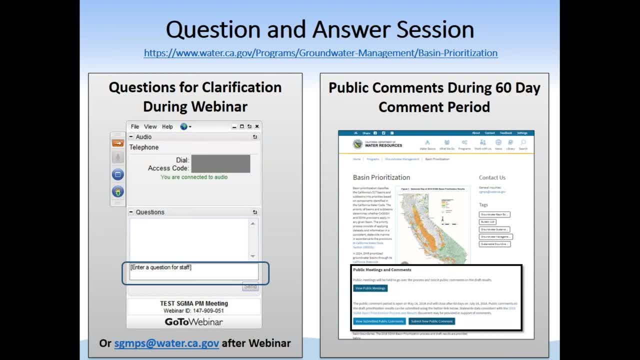 so a question here on on how subsidence. so a question here on on how subsidence was applied. why don't you talk a little was applied? why don't you talk a little was applied? why don't you talk a little about that? when I went through that one, 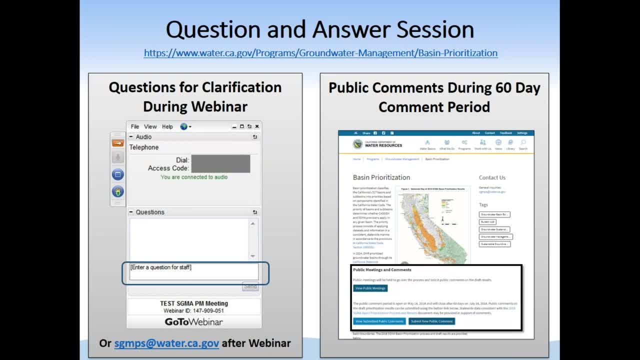 about that when I went through that one. about that, when I went through that one slide where we talked about the slide, where we talked about the slide, where we talked about the subsidence, I talked about all the subsidence. I talked about all the subsidence. I talked about all the different documents and data sets, USGS. 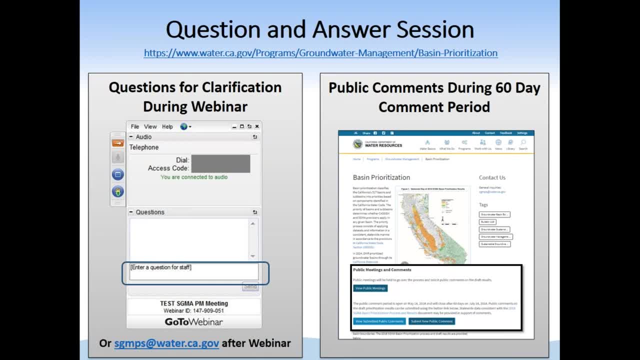 different documents and data sets USGS. different documents and data sets USGS: propulsion laboratories and documents. propulsion laboratories and documents. propulsion laboratories and documents. we and I also said that we looked at we and I also said that we looked at we and I also said that we looked at subsidence only in terms of if they are. 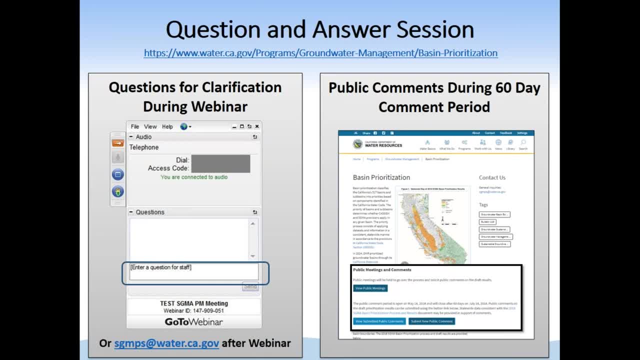 subsidence only in terms of if they are subsidence, only in terms of if they are currently having subsidence, then then currently having subsidence, then then currently having subsidence, then then the flag was established. meaning it was the flag was established, meaning it was the flag was established, meaning it was said: yes, you have current subsidence. 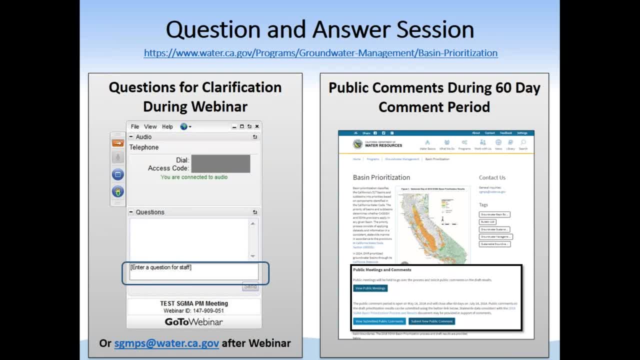 said: yes, you have current subsidence. said yes, you have current subsidence that had its own point value, the other that had its own point value, the other that had its own point value. the other aspect of subsidence we looked at was: aspect of subsidence we looked at was: 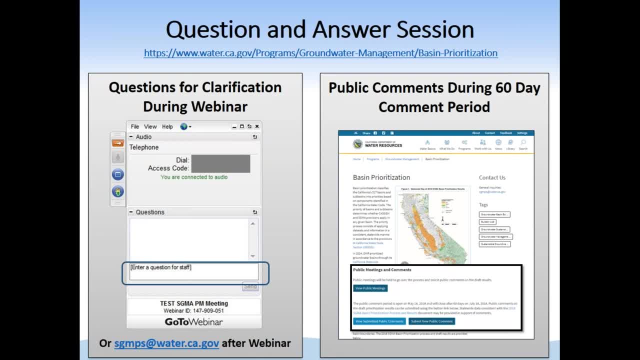 aspect of subsidence we looked at was whether or not it occurred in the past. whether or not it occurred in the past. whether or not it occurred in the past or for concerns that if the basin is not, or for concerns that if the basin is not, or for concerns that if the basin is not managed, that it could potentially happen. 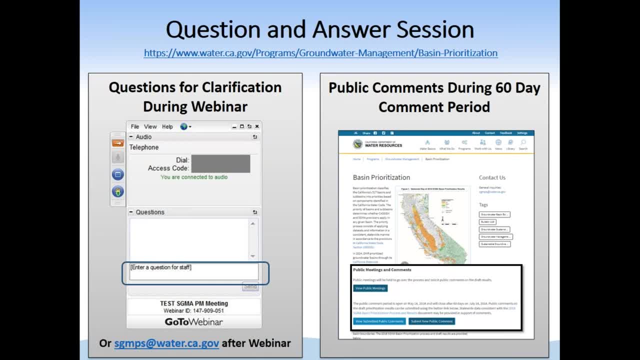 managed that it could potentially happen, managed that it could potentially happen again. so we wanted to make sure that that again. so we wanted to make sure that that again. so we wanted to make sure that that was on. the identified was identified was on: the identified was identified. 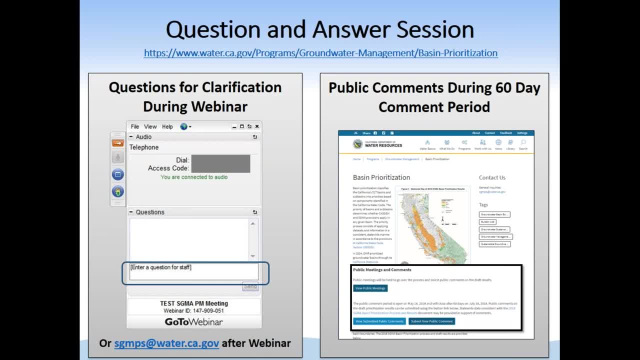 was on the identified was identified invasive prioritization, but certainly invasive prioritization, but certainly invasive prioritization, but certainly got less points for that. but those were got less points for that. but those were got less points for that. but those were the only two criteria we use, is it? 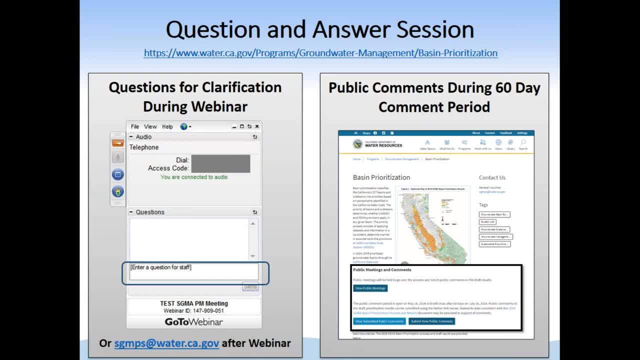 the only two criteria we use. is it the only two criteria we use? is it occurring today or did it occur in the occurring today? or did it occur in the occurring today or did it occur in the past? we did not make any determination past. we did not make any determination. 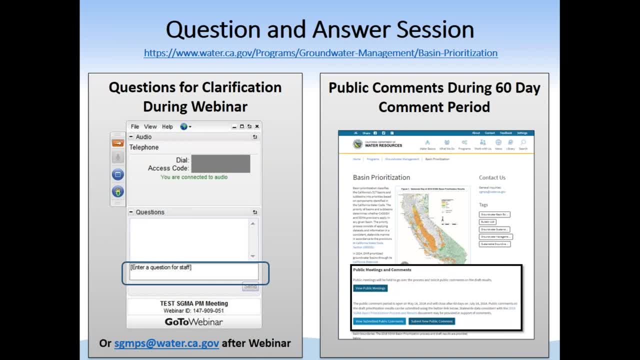 past, we did not make any determination: whether it is significant, insignificant. whether it is significant, insignificant. whether it is significant, insignificant, greater than or less than, or more. greater than or less than, or more, greater than or less than or more, damaging or less damaging: there was no. damaging or less damaging: there was no. 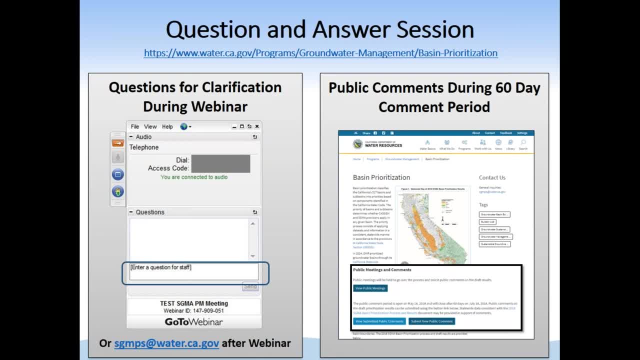 damaging or less damaging. there was no comparison between them. great, I guess. comparison between them, great, I guess, comparison between them, great, I guess. another question on speaking of details. another question on speaking of details. another question on speaking of details of these components: how population was of these components, how population was. 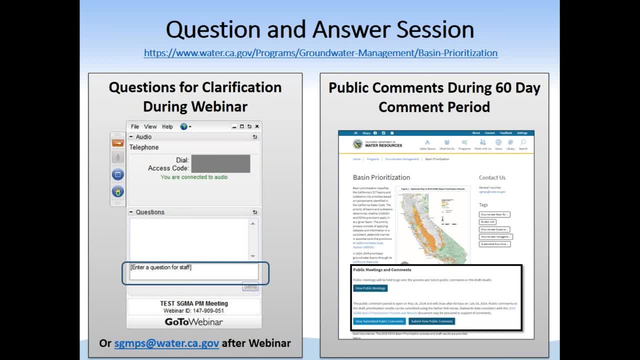 of these components, how population was applied in component six versus applied in component six versus applied in component six versus component one. you know what. what were component one? you know what. what were component one. you know what? what were those data sets, those data sets, those data sets that you relied upon for those? well, this, 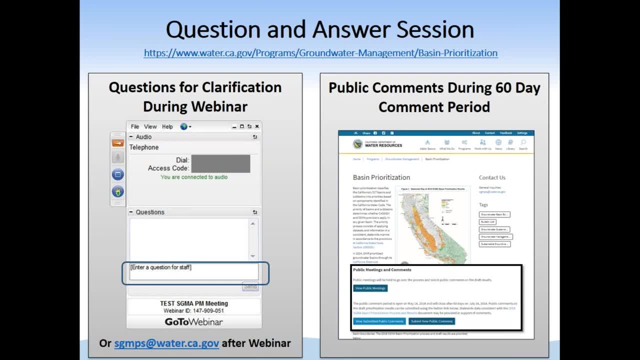 that you relied upon for those. well, this that you relied upon for those. well this. well, the data set that I used for 2018, well, the data set that I used for 2018, well, the data set that I used for 2018 was purely came from Oscar the new. 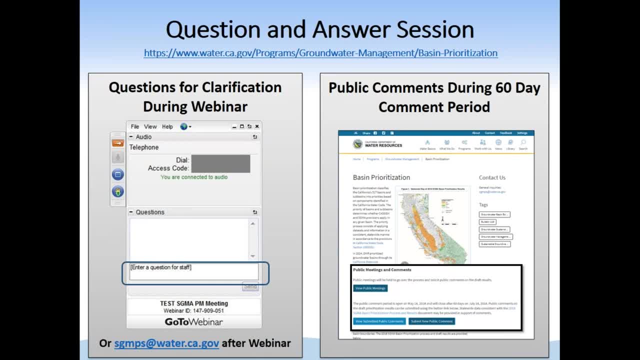 was purely came from Oscar. the new was purely came from Oscar. the new system that we currently had, the data system that we currently had, the data system that we currently had, the data set that was used in 2014 came from. set that was used in 2014 came from. 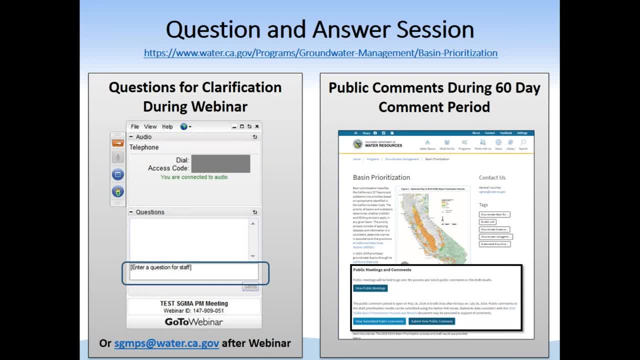 set that was used in 2014 came from several different data sets and the several different data sets and the several different data sets and the significant difference between the two, significant difference between the two, significant difference between the two and reason why we gave a 25% waiting. 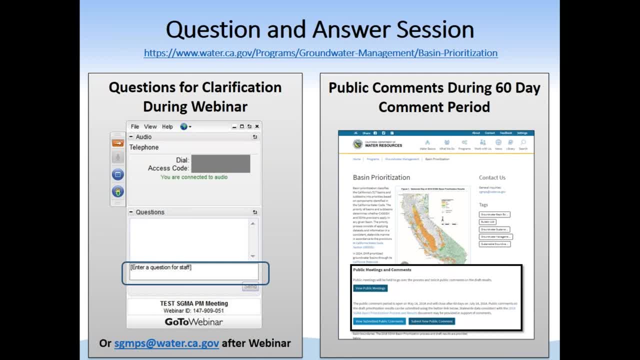 and reason why we gave a 25% waiting, and reason why we gave a 25% waiting had to do with the fact that earlier I had to do with the fact that earlier I had to do with the fact that earlier I said that I was waiting for the data set. 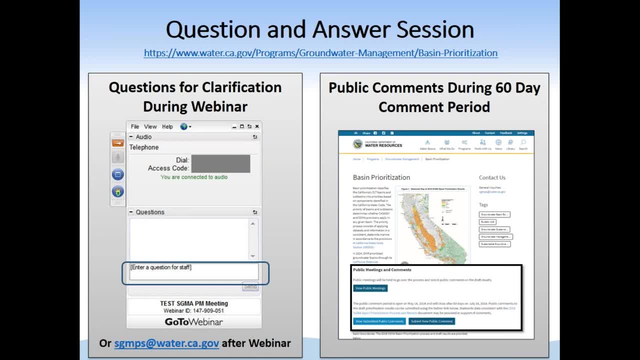 said that I was waiting for the data set, said that I was waiting for the data set because we were scanning and keying, because we were scanning and keying, because we were scanning and keying several hundred thousand my locks, so the several hundred thousand my locks, so the. 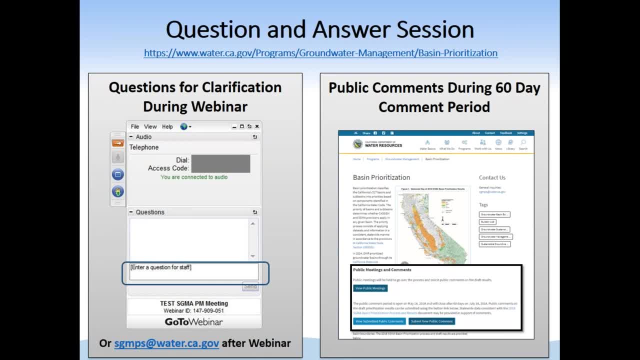 several hundred thousand my locks. so the data set today is a more accurate data set. today is a more accurate data set. today is a more accurate reflection of what we know and what we reflection of what we know and what we reflection of what we know and what we have. and the last one was, was was based 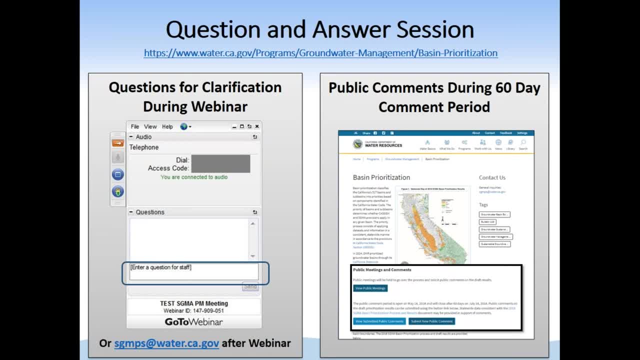 have, and the last one was: was was based have, and the last one was was was based on what we knew and what we had at the, on what we knew and what we had at the, on what we knew and what we had at the time, but we knew we were missing logs. 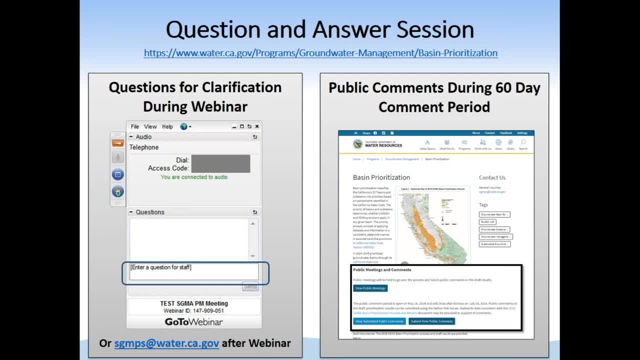 time. but we knew we were missing logs time. but we knew we were missing logs out of the system. so we discounted it by out of the system. so we discounted it by out of the system. so we discounted it by 25%. so that was the reason for the. 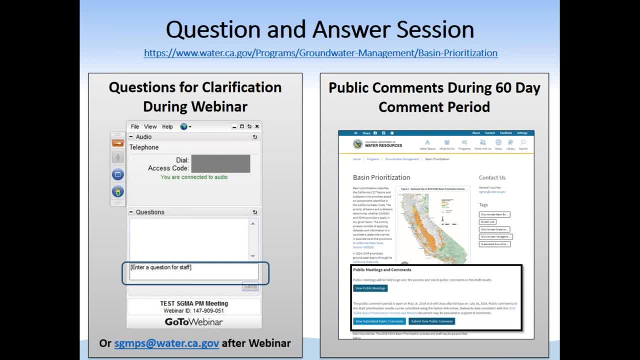 25%. so that was the reason for the 25%. so that was the reason for the discount back in 2014. all right, I don't discount back in 2014. all right, I don't discount back in 2014, all right. I don't think I was clear of my question for you. 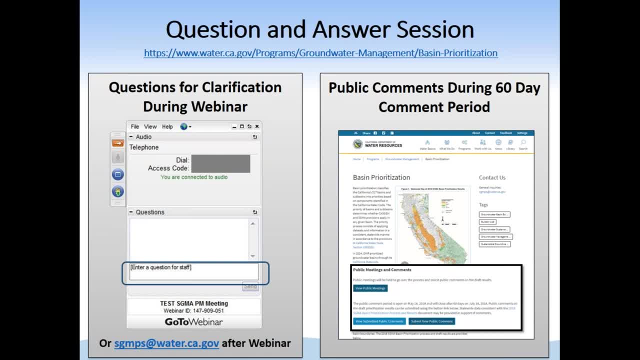 think I was clear of my question for you. think I was clear of my question for you. I think you answered there about the. I think you answered there about the. I think you answered there about the specific logs, the well logs themselves. specific logs, the well logs themselves. 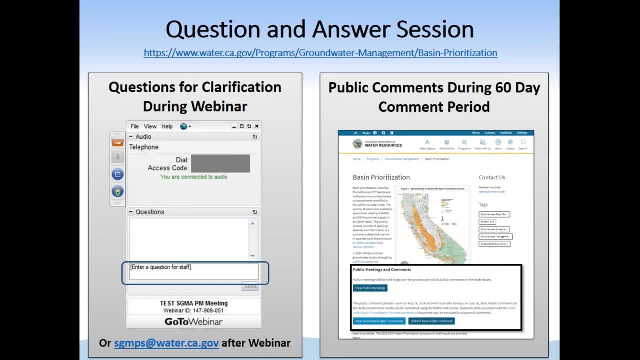 specific logs, the well logs themselves versus the population. so the question versus the population. so the question versus the population. so the question being asked is for component six used. a being asked is for component six used. a being asked is for component six used a third-party population data from 2014. 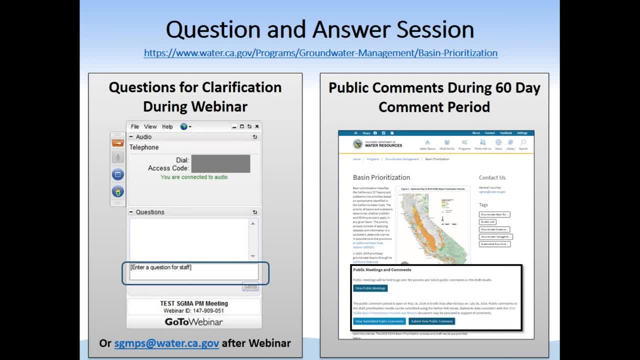 third-party population data from 2014. third-party population data from 2014. and we use the 2014 data there for, and we use the 2014 data there for, and we use the 2014 data there for population. why not use the component one? 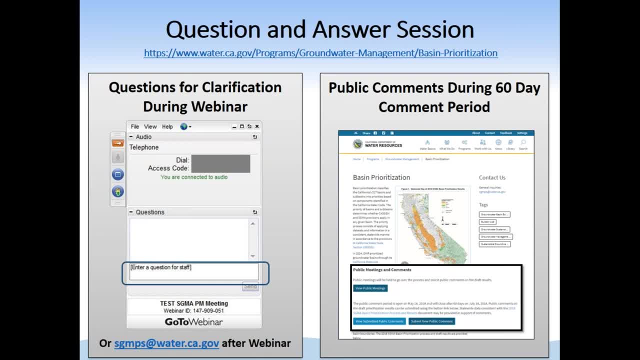 population. why not use the component one population? why not use the component one population rather than our component one population rather than our component one population rather than our component one population rather than 2010. why not use population rather than 2010? why not use population rather than 2010? why not use 2010 data? 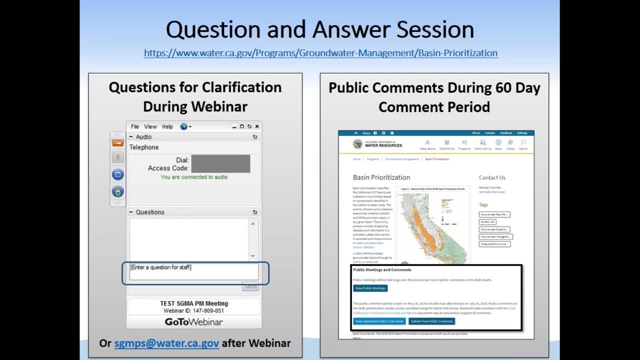 2010 data, 2010 data: well for the population, well, we did use. well for the population. well, we did use. well for the population. well, we did use. 2010 population for component one: yes. 2010 population for component one: yes. 2010 population for component one: yes. okay, we have a question through email. 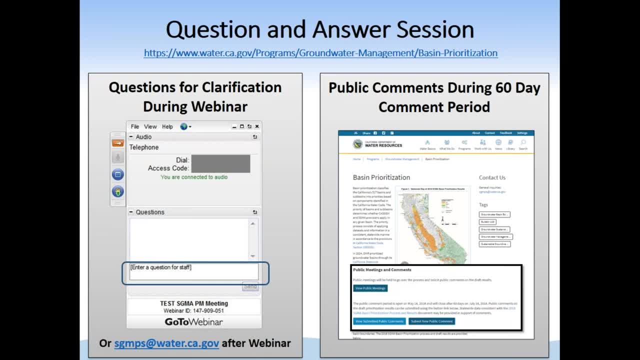 okay, we have a question through email. okay, we have a question through email to question reads. currently, our basin is to question reads. currently, our basin is to question reads. currently, our basin is shown as pumping less than 2,000 acre. shown as pumping less than 2,000 acre. 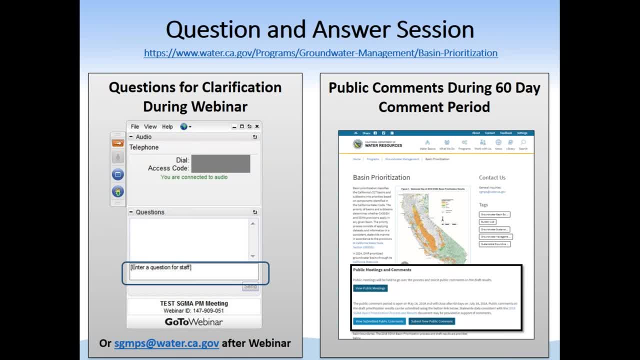 shown as pumping less than 2,000 acre feet, which of course is the threshold feet, which of course is the threshold feet, which of course is the threshold for which, for which, for which basin is being very low in the future. basin is being very low in the future. 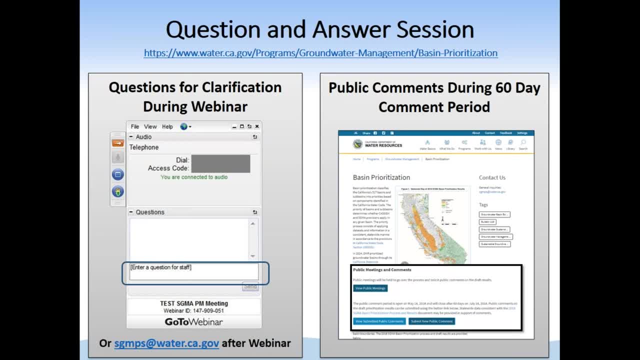 basin is being very low in the future if it's found to be more than 2,000 acre. if it's found to be more than 2,000 acre. if it's found to be more than 2,000 acre feet. what happens? how often does he do? 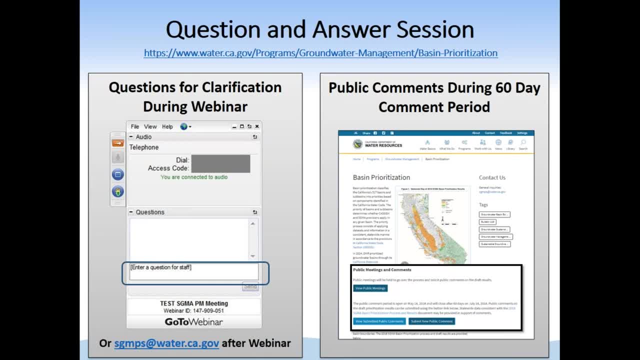 feet. what happens? how often does he do feet? what happens, how often does he do? our reprioritized base- so good question. our reprioritized base, so good question. our reprioritized base, so good question. you know, we will only evaluate this when. you know, we will only evaluate this when. 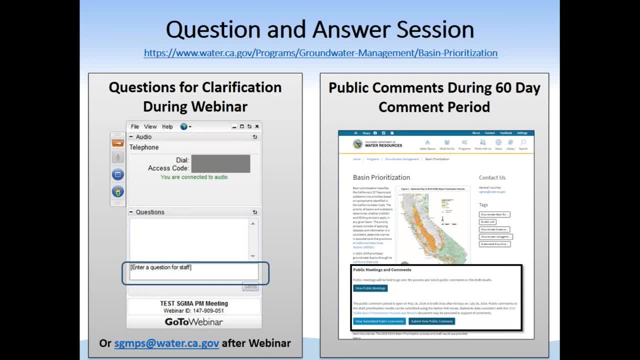 you know, we will only evaluate this when we do reprioritization, as I mentioned. we, we do reprioritization, as I mentioned. we, we do reprioritization, as I mentioned. we are not anticipating reprioritizing, are not anticipating reprioritizing. 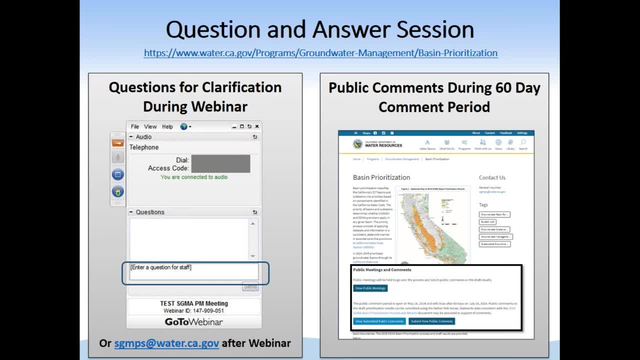 are not anticipating reprioritizing bases perhaps three to five years, but bases perhaps three to five years. but bases perhaps three to five years, but it's again based on whether there are, it's again based on whether there are, it's again based on whether there are based in boundary modifications and that 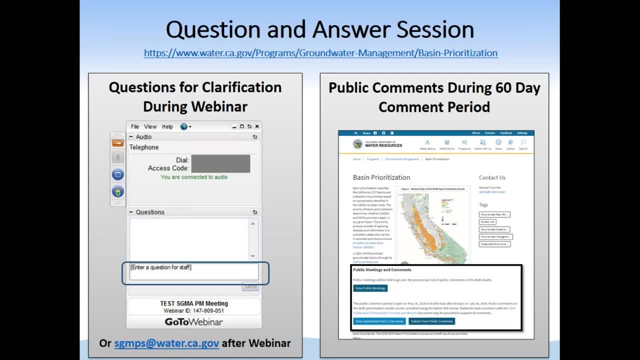 based in boundary modifications and that based in boundary modifications and that triggers our role to reevaluate. consider triggers our role to reevaluate. consider triggers our role to reevaluate, consider prioritization so if nothing were to go, prioritization so if nothing were to go. prioritization so if nothing were to go. up or down. now, between us prior, 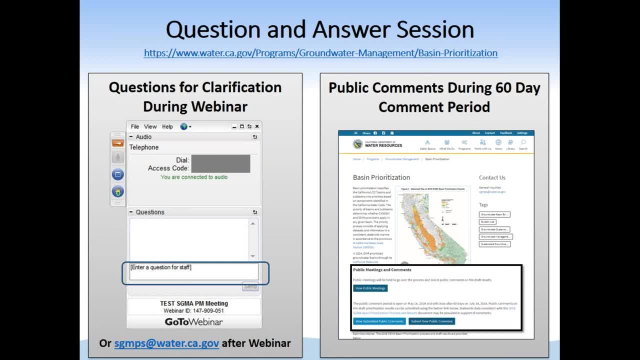 up or down now between us prior. up or down now between us prior. reprioritizing basins: really nothing. reprioritizing basins, really nothing. reprioritizing basins, really nothing. happens from our perspective, we are not. happens from our perspective, we are not. 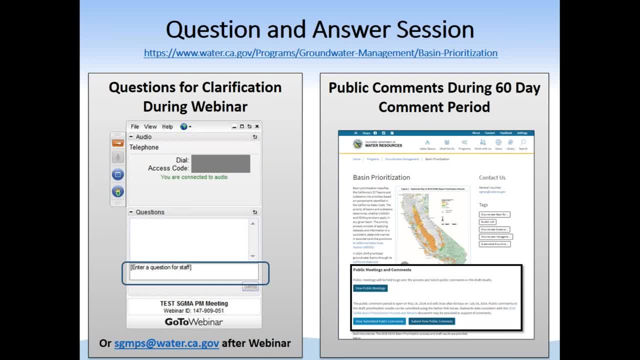 happens from our perspective? we are not. this is not kind of a real-time. if you, this is not kind of a real-time if you, this is not kind of a real-time if you will, analysis to evaluate the priority will, analysis to evaluate the priority will analysis to evaluate the priority invasions. it only happens at specific. 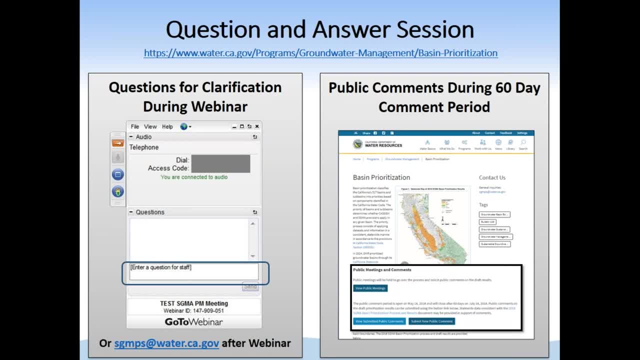 invasions. it only happens at specific invasions. it only happens at specific times when we really look at this easy times, when we really look at this easy times, when we really look at this easy based boundary modifications- great based boundary modifications- great based boundary modifications- great regarding irrigated acreage and 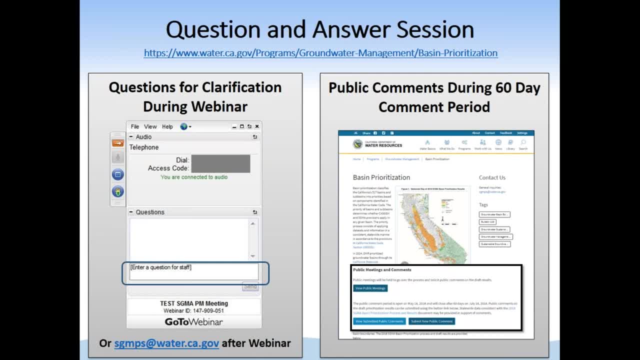 regarding irrigated acreage and regarding irrigated acreage and groundwater use for climate. regional groundwater use for climate. regional groundwater use for climate. regional climates considered as factors affecting climates. considered as factors affecting climates. considered as factors affecting crop irrigation demands, or where crop irrigation demands or where 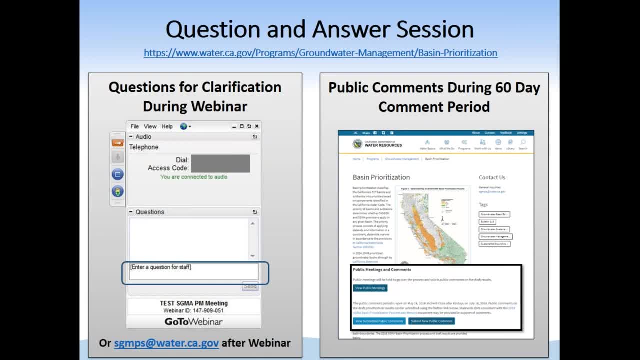 crop irrigation demands or where stock values applied statewide. so the stock values applied statewide. so the stock values applied statewide. so the short answer for that is yes. yes, we did. short answer for that is yes, yes, we did. short answer for that is yes. yes, we did make regional climates. trying to read: make regional climates trying to read. make regional climates trying to read the question at the same time. trying to the question at the same time. trying to the question at the same time, trying to answer it. okay, let me go back and answer it. okay, let me go back and. 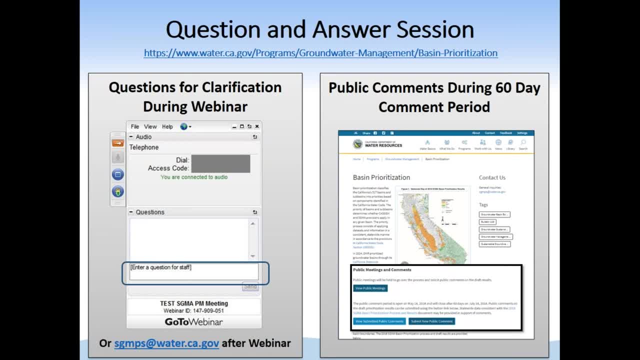 answer it. okay, let me go back and explain how we looked at that, explain how we looked at that. explain how we looked at that information. each basin was looked at in information. each basin was looked at in information. each basin was looked at in terms of its precip soil moisture. we 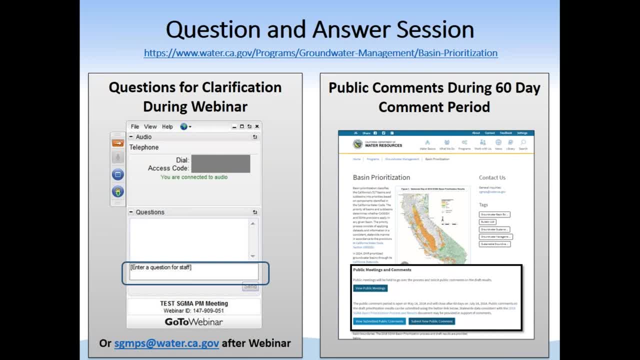 terms of its precip soil moisture. we terms of its precip soil moisture, we used the tool or an applicant model. used the tool or an applicant model. used the tool or an applicant model called calcimita, so all the regional. called calcimita, so all the regional. 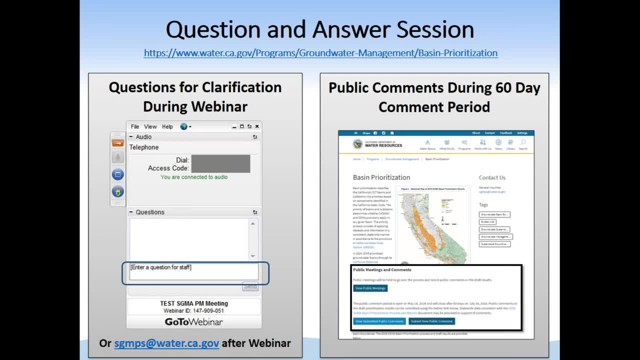 called calcimita. so all the regional down to a- what we call a detailed- down to a, what we call a detailed- down to a, what we call a detailed analysis unit was processed, so we looked. analysis unit was processed, so we looked. analysis unit was processed so we looked at cropping patterns, irrigated acreage. 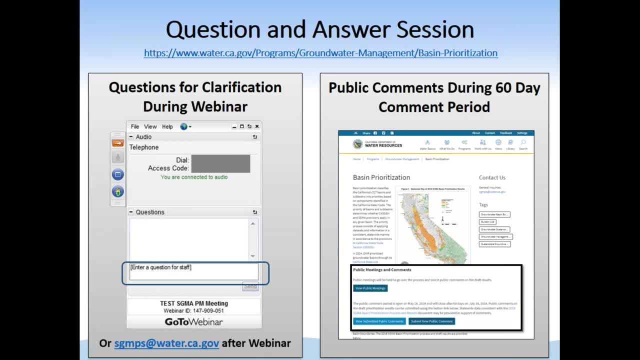 at cropping patterns- irrigated acreage. at cropping patterns- irrigated acreage. we looked at planting and harvesting. we looked at planting and harvesting. we looked at planting and harvesting times. we looked at precip soil moisture times. we looked at precip soil moisture times. we looked at precip soil moisture and, I'm sure, a host of other things. I 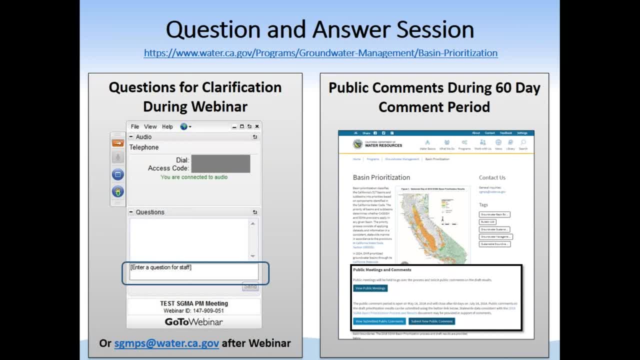 and I'm sure a host of other things. I and I'm sure a host of other things. I mean there's some modelers. that would mean there's some modelers. that would mean there's some modelers that would probably know all the details. but yes, we. 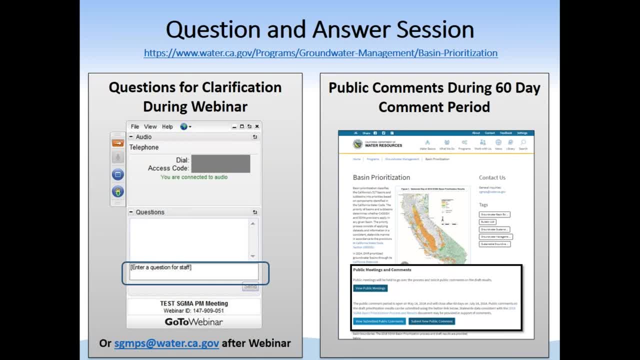 probably know all the details. but yes, we probably know all the details. but, yes, we looked at all that in each basin. but looked at all that in each basin. but looked at all that in each basin, but individually processed for that and the individually processed for that and the. 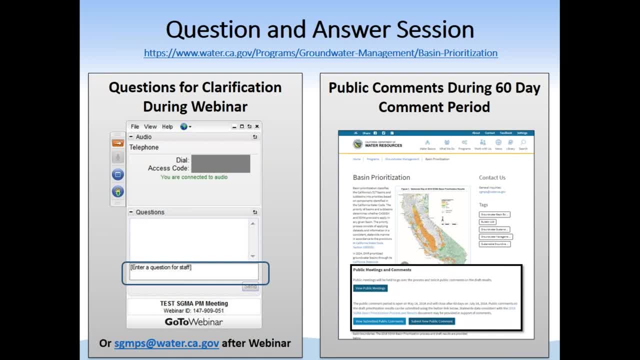 individually processed for that. and the land use folks who's been working with land use folks who's been working with land use folks who's been working with them for many years, have been keeping up them for many years, have been keeping up them for many years, have been keeping up on top of all that information- great, I. 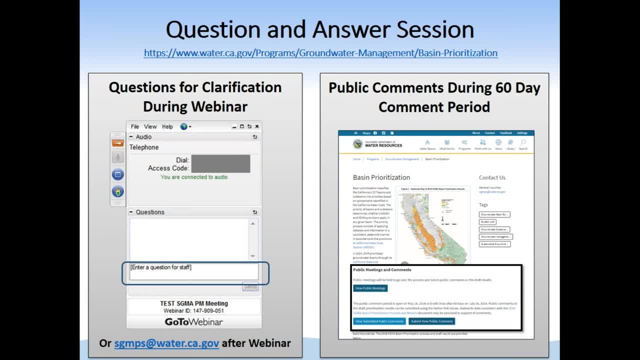 on top of all that information- great I. on top of all that information, great I think we've worked through our questions, think we've worked through our questions, think we've worked through our questions. that we've have it's kind of that we've have it's kind of. 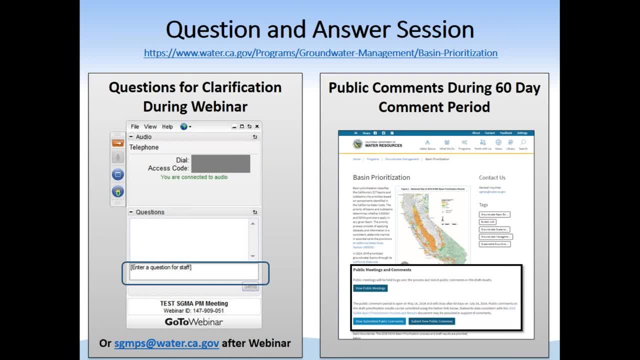 that we've have. it's kind of consolidate any last thoughts here, consolidate any last thoughts here, consolidate any last thoughts here, Steven, all right. so we'll wait a few, Steven. all right, so we'll wait a few, Steven. all right, so we'll wait a few more minutes to see if there's any. 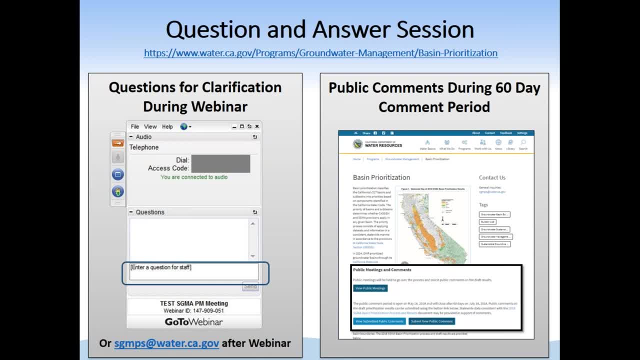 more minutes to see if there's any more minutes to see if there's any questions. additional questions that are questions. additional questions that are questions. additional questions that are coming in again. these questions are for coming in again. these questions are for coming in again. these questions are for clarification on the information that 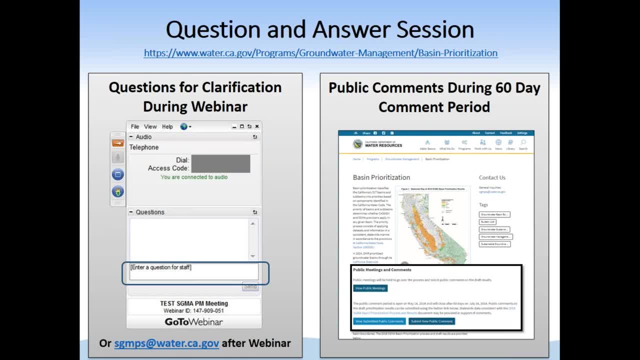 clarification on the information. that clarification on the information that was presented during the webinar today so was presented during the webinar today. so was presented during the webinar today. so we'll pause just for a moment to see if we'll pause just for a moment to see if. 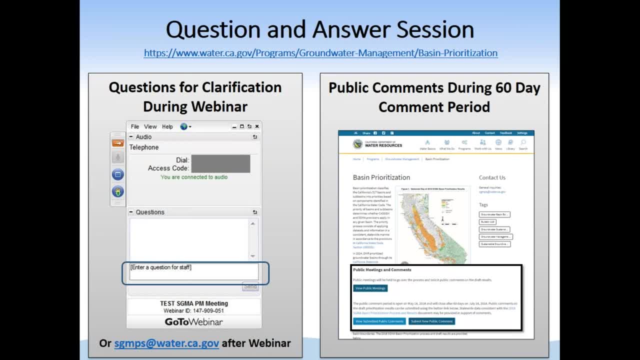 we'll pause just for a moment to see if any questions come in and we'll be back. any questions come in and we'll be back. any questions come in and we'll be back in just a moment. you, you, you, you all right, thanks for keeping. 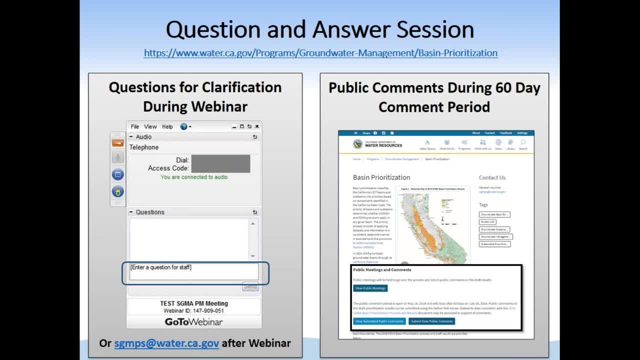 all right, thanks for keeping the comments coming. we've had a couple more, so a lot of data is based on the draft California water plan 2018, which is not final draft document. how can there be certainty in the data? could it change in? certain values change as. 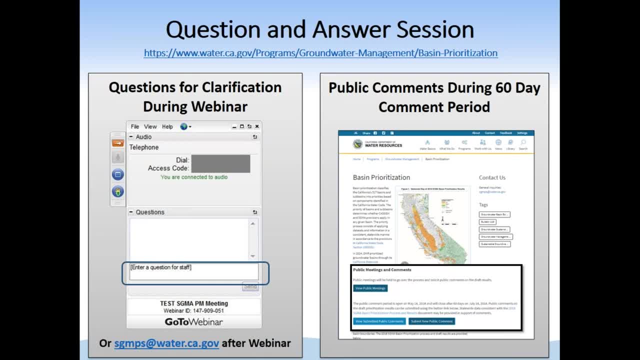 things before. well, both of both the plan and basin prioritization are draft at this point, so public comments are coming in for us on basin prioritization as well well as us for the water plan. the data sets that we used out of the water plan were were basically stable data sets, population information and 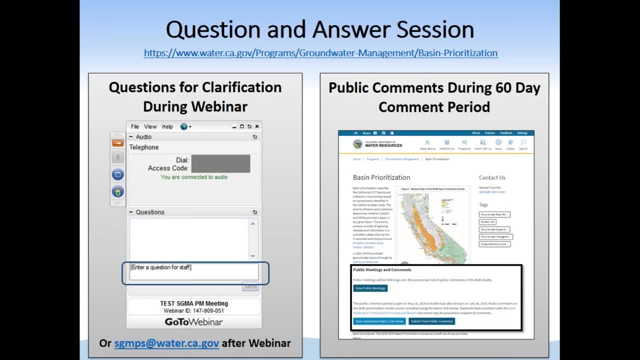 forecasting that have been basically repeated with respect to water plans of the past. they've been forecasting 20, 30, 20, 40, 20, 50, so we just picked up on the same data set as well as other information. now they do report on information going on with the conditions. 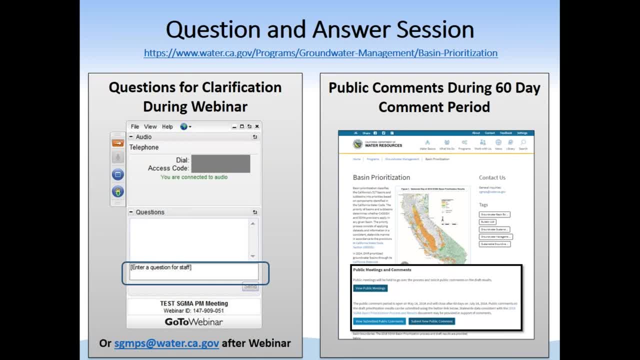 around the state that we also looked at and certainly, if, if any of that data changes, it would, it would be a good idea to discuss that with respect to an individual basin. so if it's not, if it's not correct, that's the whole point of the work. the work that we're seeing around you is to was Abby, what? 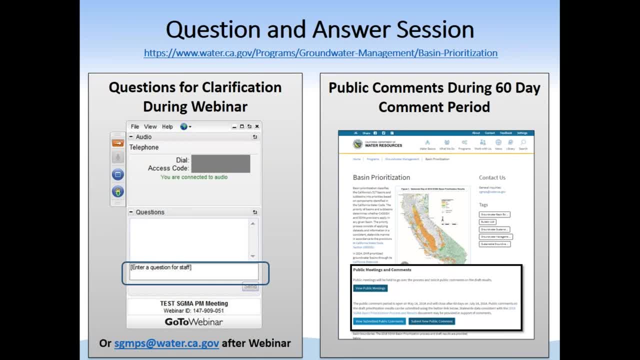 information would be a good direction. mathematical muffin: move the data at this point here, so by the end of the table. this dashboard is just a very simple look at where the water plant is going and how we could make some more WR triumph. that I don't think, indeed, would actually apply if you. 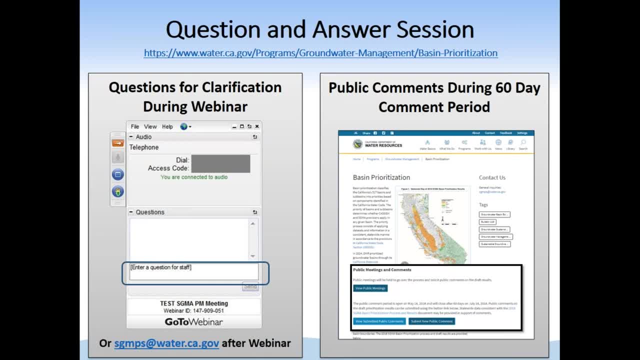 can dedi like are getting a couple more comments. I'm just trying to understand how to consolidate them. Great, Okay, so one more question regarding some of these components, specifically saline water intrusion. It seems that bulletin 118.2003 defines saline intrusion without regard to the cause of the intrusion, but it implies 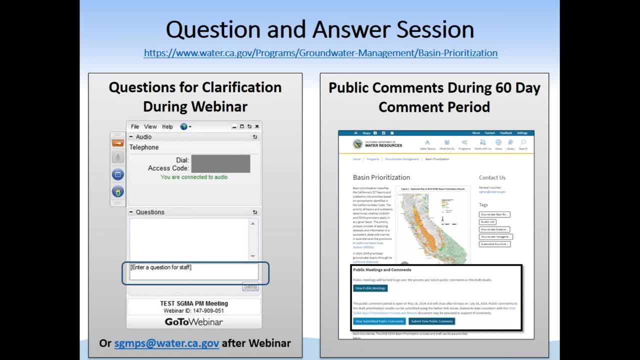 that occurrence of saline intrusion is a condition that is observed to have changed over time. Did the evaluation attempt- the evaluation being the prioritization process- attempt to determine whether salinity concentrations have changed over time? So the answer to that is no. Again, the approach we took on that was whether or not it is occurring currently. We did not. 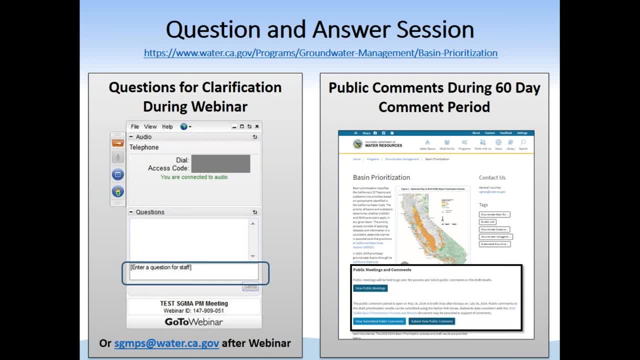 take into consideration any other factor, meaning, is it abated, is it getting worse? only because it's a very fluid type situation, tomorrow, today? So no, we did not make any assessment over its current condition, other than if it exists. Great, Okay, We're down to the last question here. 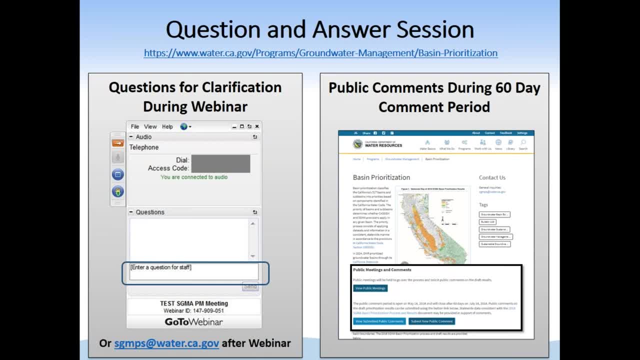 Do you anticipate that public comments will be an effective tool for refining the results of the prioritization? Yeah, I can handle that one. Yeah, we definitely do feel that public comments are going to be a part of this. It's an important reminder. 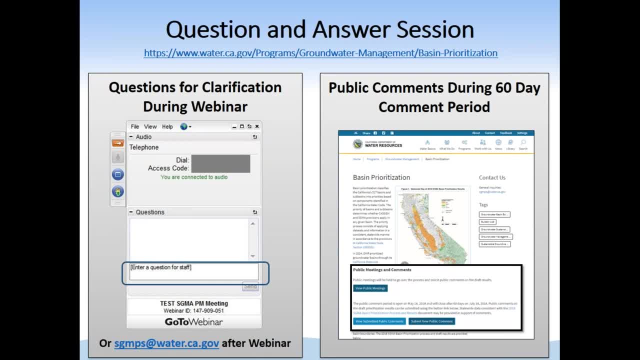 Okay, Again, these are draft results and we're looking to see if there's information that comes in that over the 60-day public comment period that we could use and that might mean that some of these results that are in draft now might change between draft and final. 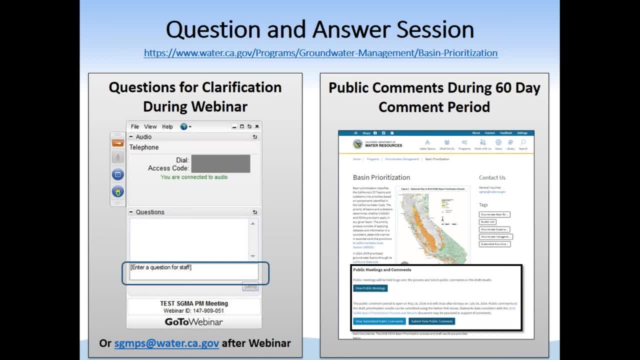 So, again, those type of comments we're looking for that would be submitted through the basin prioritization webpage that's on the screen there on the right. Our comments that focus directly on the draft 2018 prioritization results. again, comments that identify the specific water code components that are being commented on and specific references. 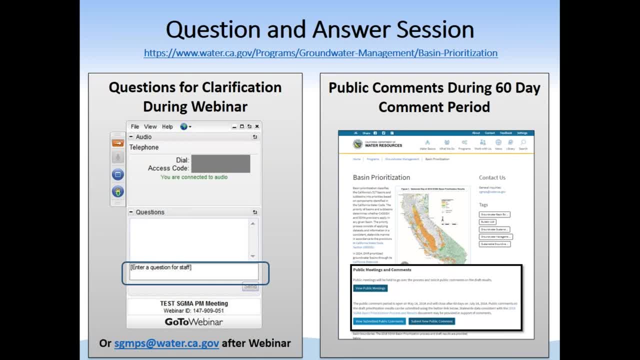 or citations that are included in those comments. And again, if there's supporting data that are out there in those basins that you're wanting to submit with your comments or associated with your comments, we're asking you to include that information with your comments as you submit it through the webpage.